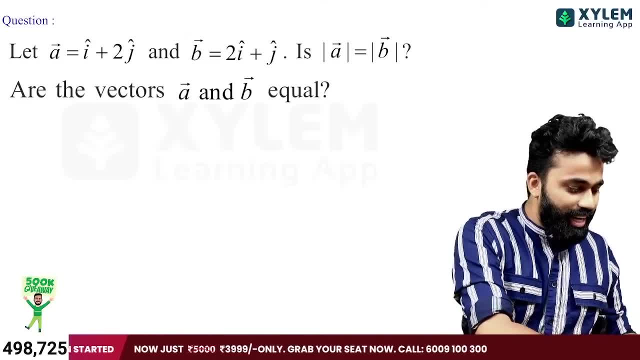 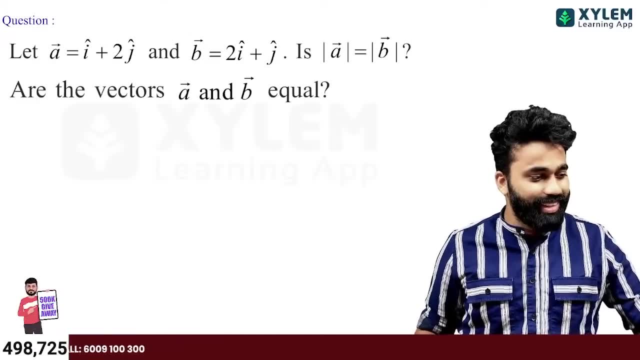 Yes, yes, yes. Only with 1300 people, Only with 5 lakhs. Has it not started yet? Yes, it has started, Only with the count of 1300.. What is it To get to the count of 5 lakhs? 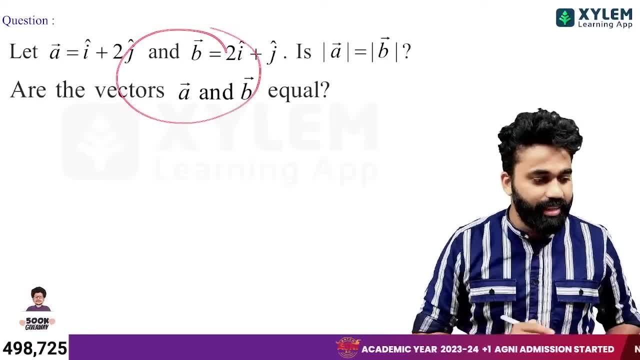 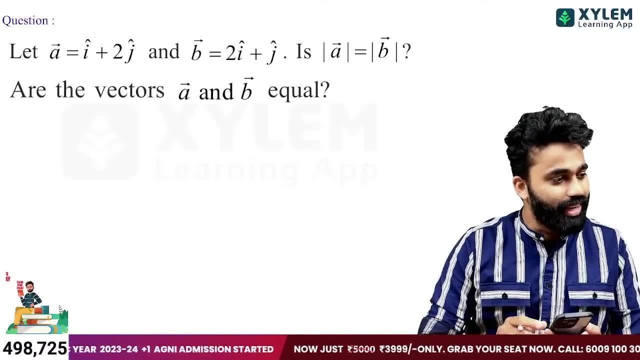 So, dear kids, be careful. Comment the answer to this question. How is the question? I'll check it in my phone. Is there an answer? Okay, Okay, There are 2.4K people here, If you think. 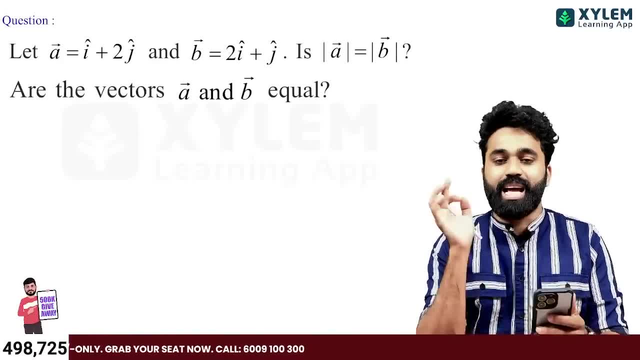 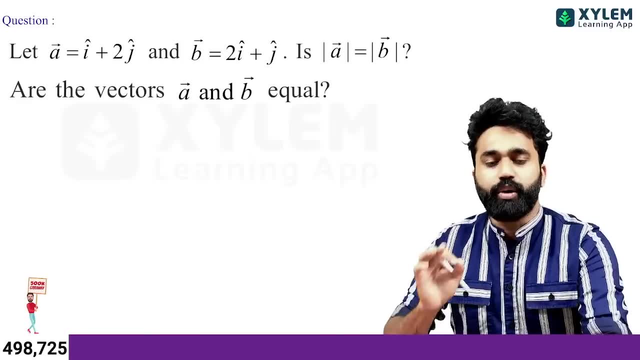 If you think, today, this day, Today, at this time, Who can celebrate my happiness? You have to think about it or you have to try. That's all I have to say. So one thing is for sure, dear kids: 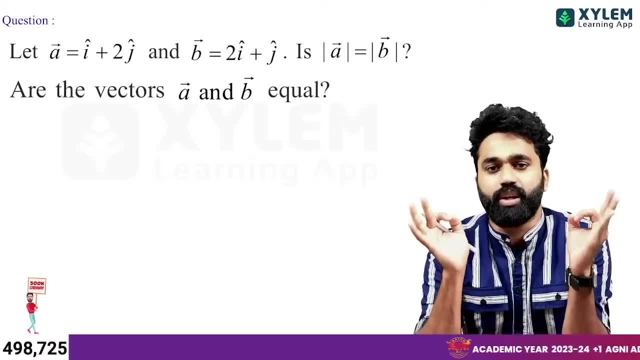 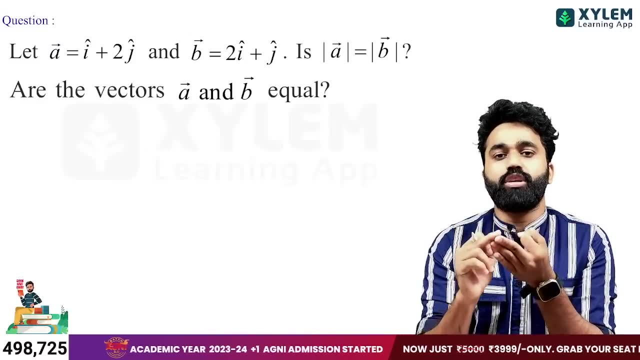 Those who want to get an A plus or a good mark. The chapters that can be studied most easily: Matrix Determinants, Vector algebra, Three dimensional geometry, LPP Relations and functions- This chapter- If you study only this chapter, you will get a good mark. 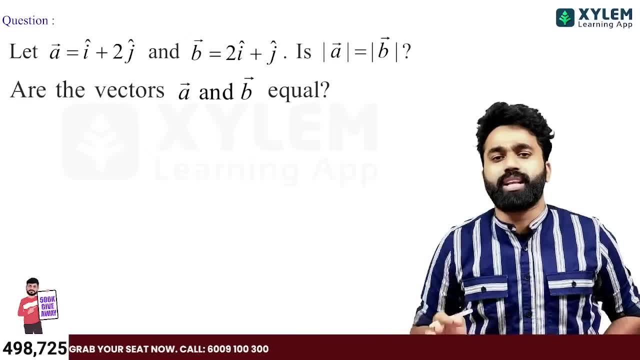 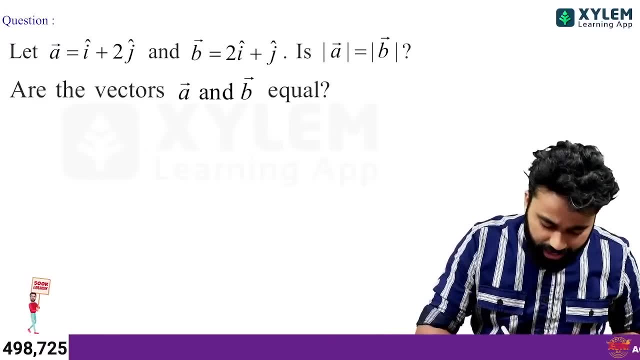 You can score a mark beyond what you expect. There is no doubt about it. It is 100% sure. You can see it with the weightage of each chapter: About 7 marks from the matrix, 9 marks from the determinants. 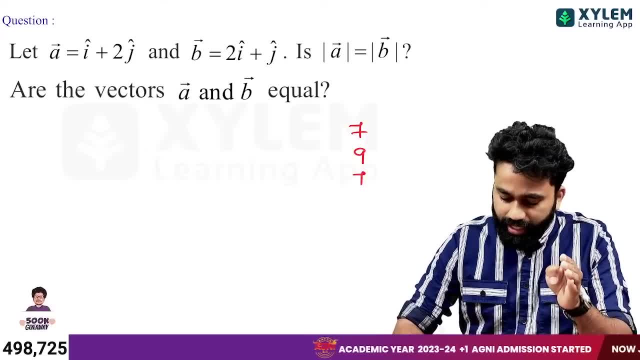 7 marks from the vector, 7 marks from the 3D, 6 marks from the LPP. Do you know how many marks it is if you study these 5 chapters? 9,, 7,, 16,, 7,, 23,, 7,, 30,, 36 marks. 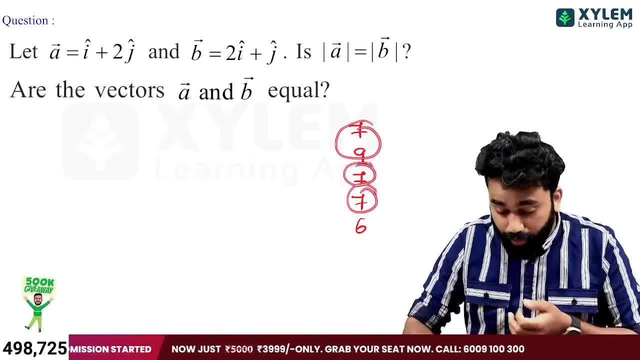 If you study these 5 chapters you will get a good mark 30.. 36 marks 6, 7,, 16,, 7, 36.. 36 from 60 is equal to B plus. It is very simple. 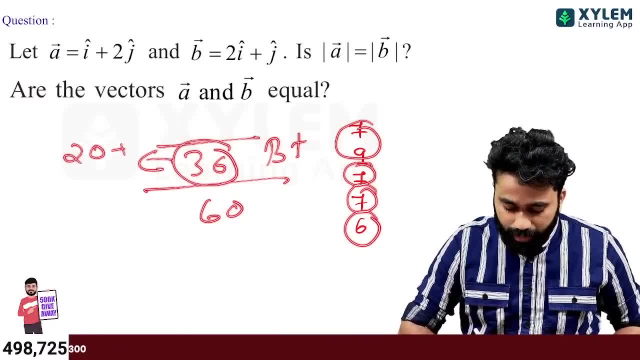 Fun fact: You will get a good mark beyond 20.. You will get a C mark. A C mark will result in 20.. Or if you score at least 15 marks, you will get a lab mark. 20 marks will be declared as 20.. 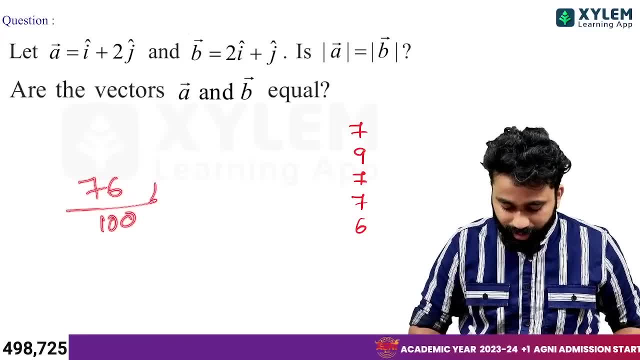 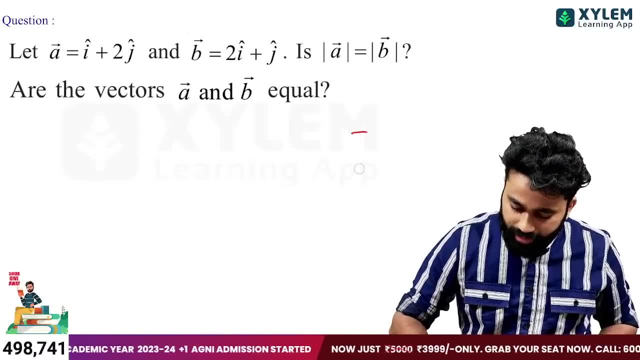 45 plus 36 is equal to 76 marks out of 100.. Simple right. It is not like what you think. So, girls, Bear the question here. Bear the question here. Yes, Here is the question. We have given 2 vectors. 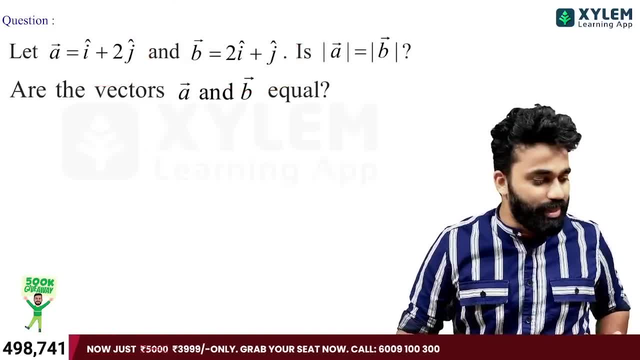 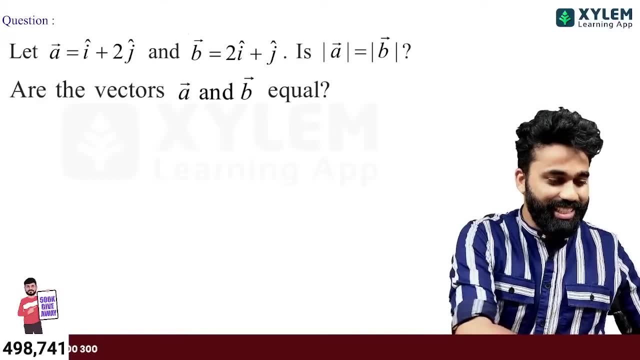 When you read this, you can understand. There are no other vectors. We can understand it at the same time. Are you ready? Can you set it up? 5 lakhs subscribers. I am giving you a status. I am saying the same as Madhav sir. 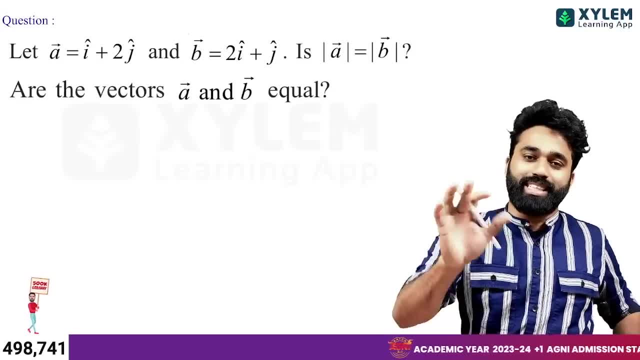 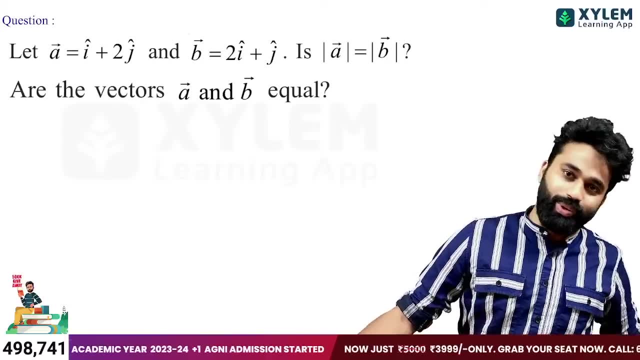 You mention it. We will do the re-mention when we get a story. You don't have to worry about it. Our aim is to make it 5 lakhs subscribers. That is what I am thinking. 5 lakhs would be great. 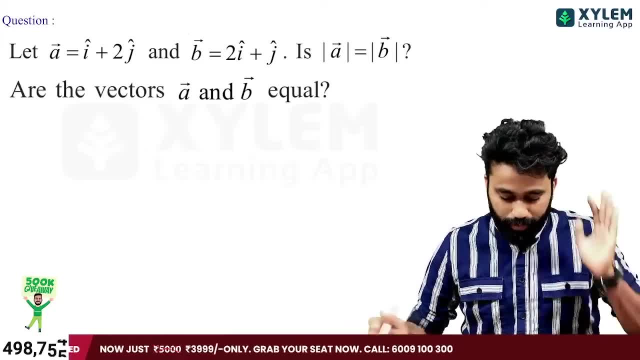 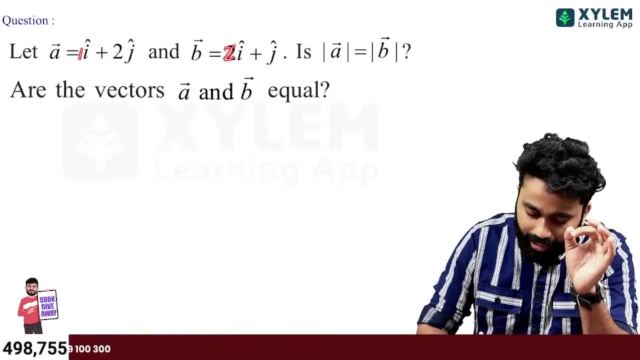 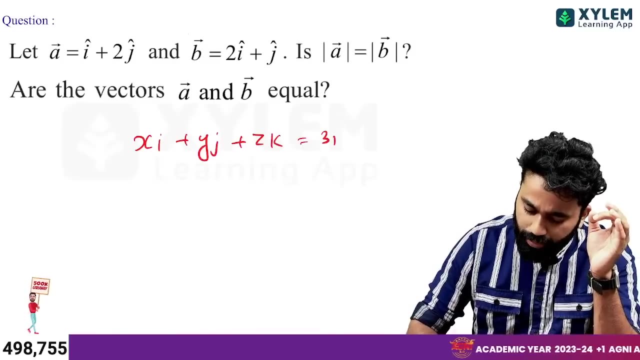 But it is an effort. It will happen only if you think so. If two vectors are equal, the i component should not be 2.. For example, if xi plus yj plus zk is equal to 3i plus 4j minus 2k, 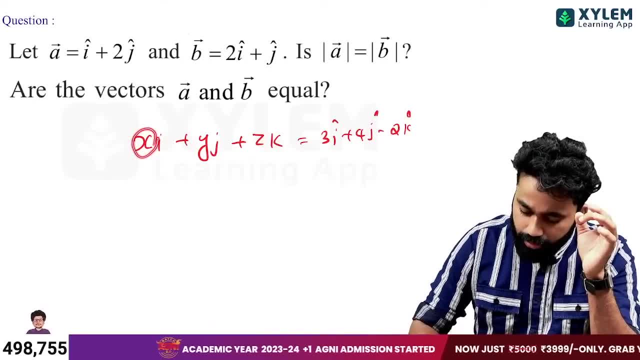 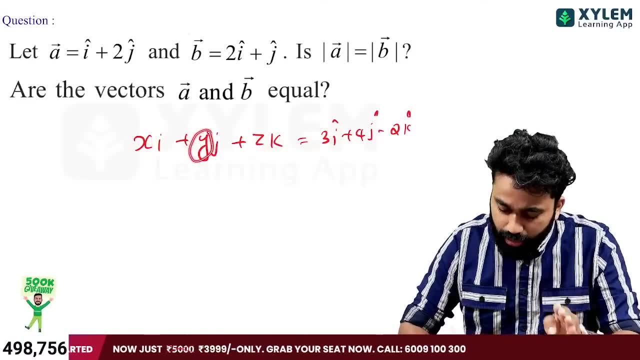 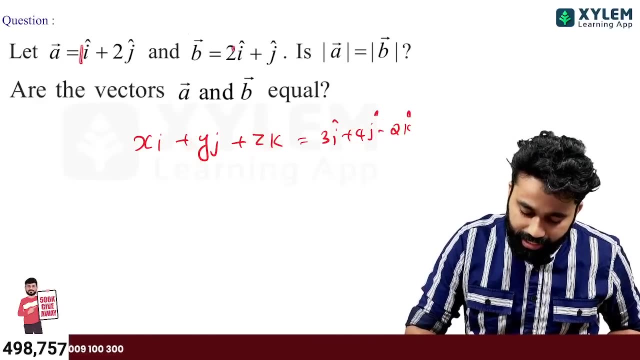 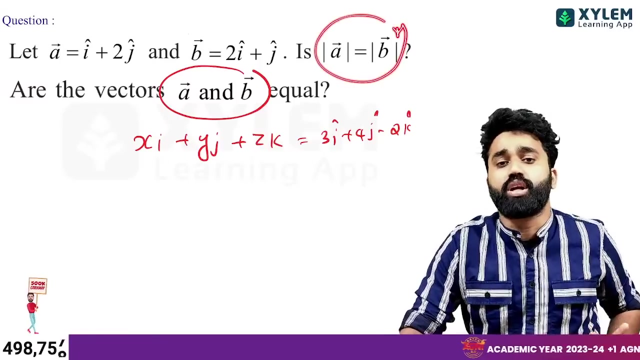 make sure that the i coefficient is equal to the j coefficient, is equal to the k coefficient is equal to the k coefficient because the two are not equal. a vector not equal to b vector. But there is a question: Is the magnitude of a equal to the magnitude of b? 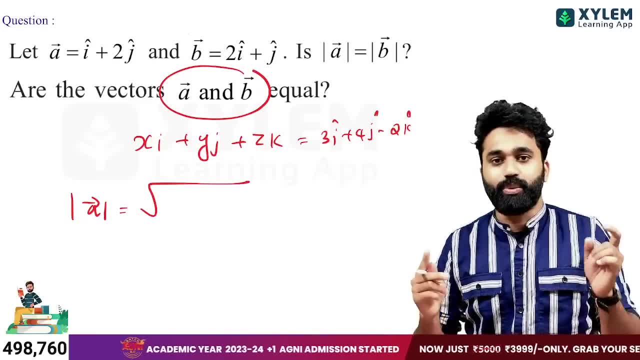 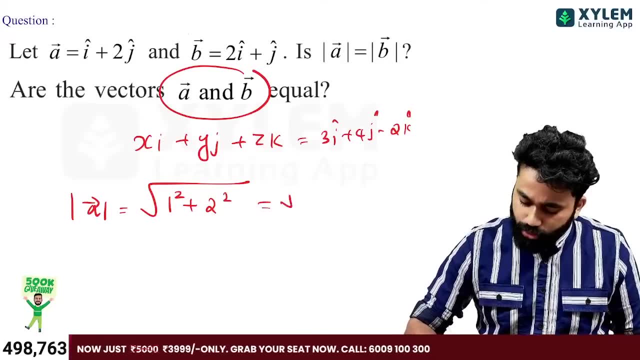 Let us see What is the magnitude of a. I haven't paused it. The magnitude of a is 1 square plus 2 square. Root of 1 square plus 2 square is root 5.. The magnitude of b is 2 square plus 1 square. 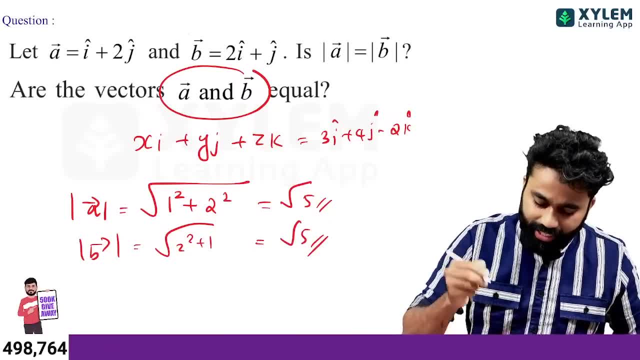 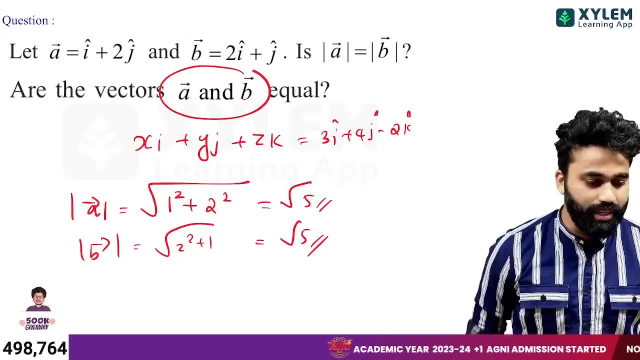 Both of these things are the same. Both of these things are clear and perfect. Those who understand, please smile. Both of these things are clear and perfect. Those who understand, please smile. Those who understand, please smile. Sir, are you getting tensed? Yes, you should. 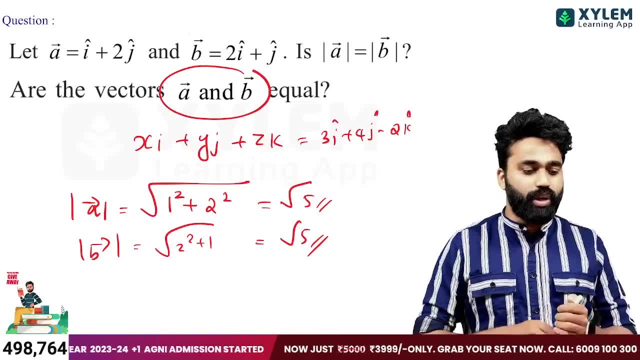 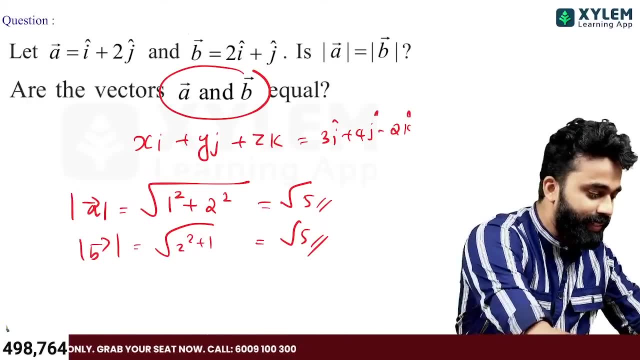 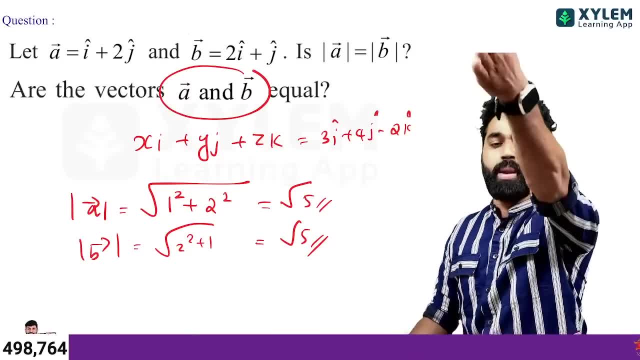 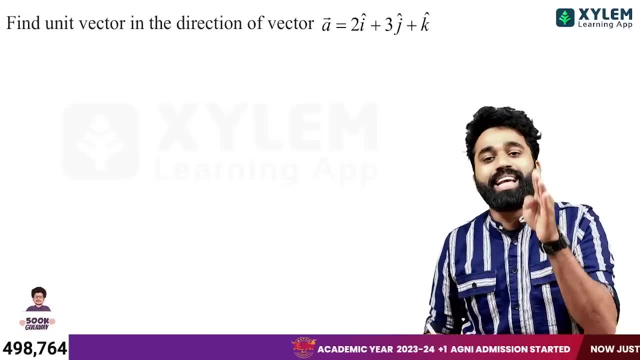 I am not a YouTuber. You are going up after 309044.. You are going up after 309044.. Yes, this is your energy and power. Please be careful. This is important to say. You have asked the question of the modern exam. 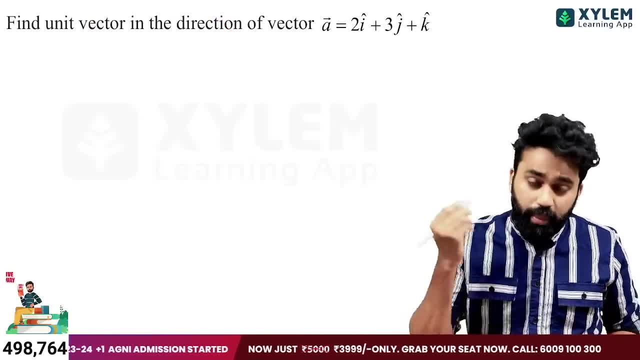 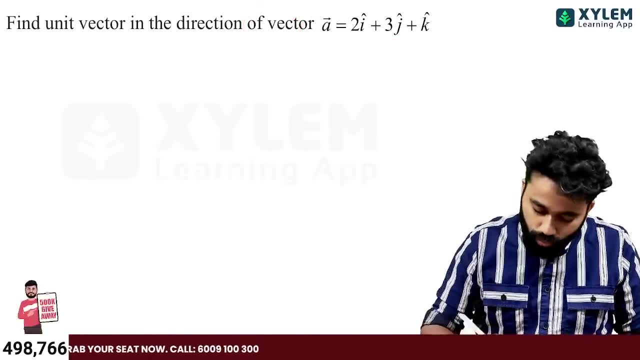 That too, for 3 marks. You have asked for 3 marks. I will show you another question for 3 marks. Find unit vector in the direction of the vector A. Find unit vector in the direction of the vector A. There is no problem. 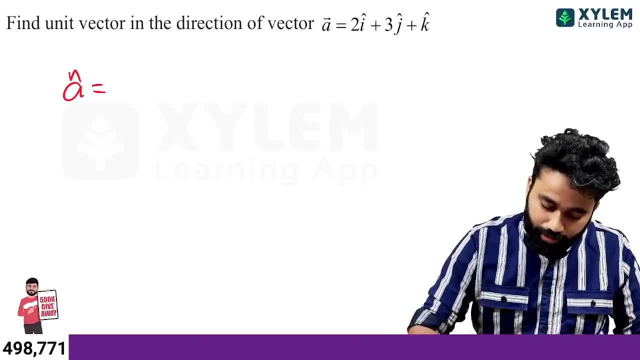 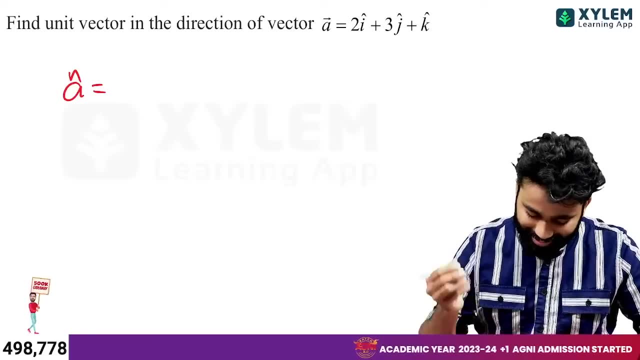 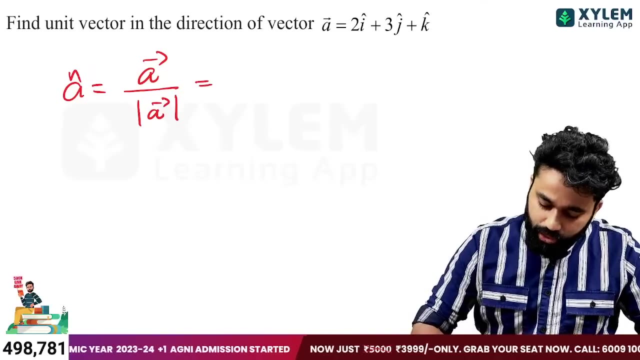 To see unit. vector A is the cap. It is a cap. It is a Javan vector. It is a Javan vector. Do you remember Javan vector A? cap is vector A divided by magnitude of A. Vector A is 2i plus. 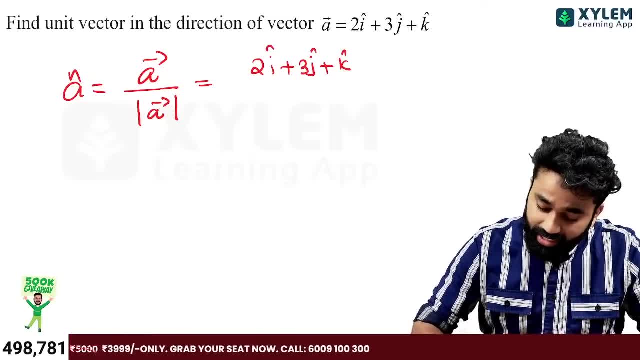 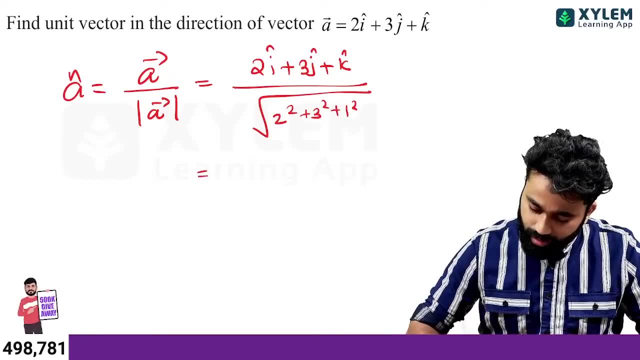 3j plus k. This is the model of your exam. This is the model of your exam By root of 2 square plus 3 square plus 1 square. The answer is 2i plus 3j. The answer is: 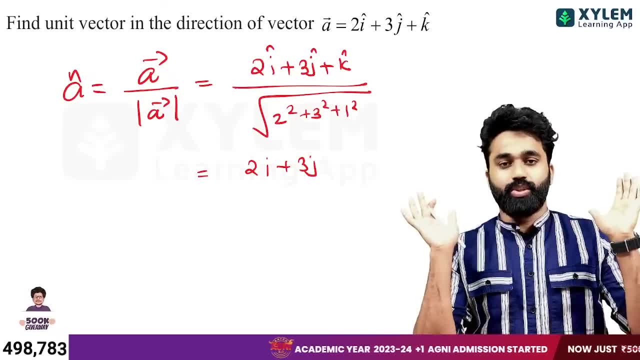 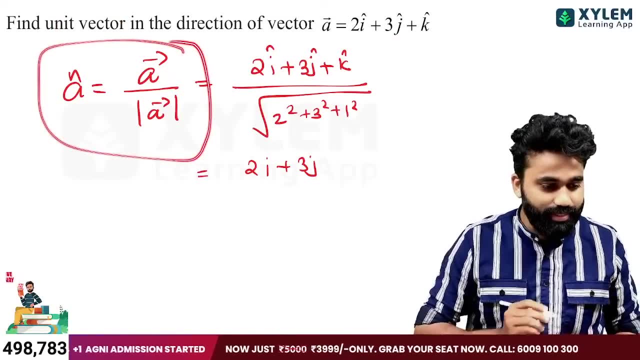 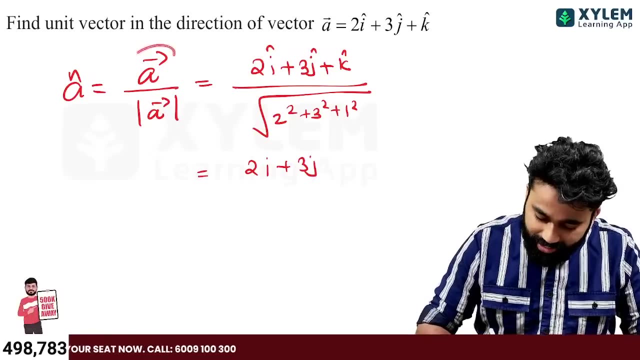 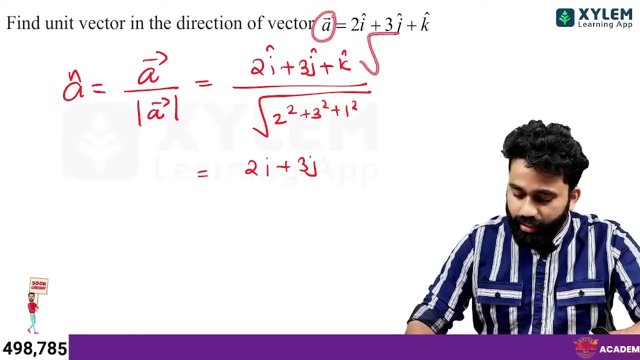 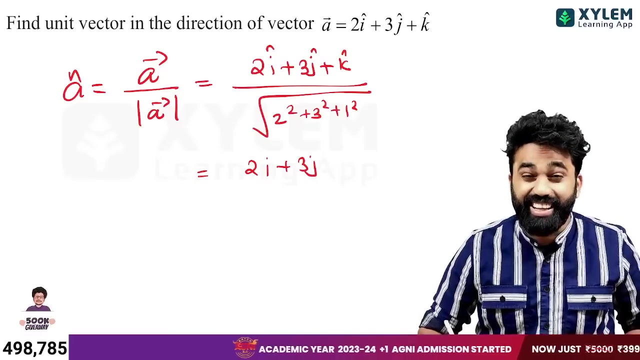 2i plus 3j. The answer is 2i plus 3j. the correct answer is 2i plus 3j of the vector. As you can see, the measurement is unit vector day. okay, so if it's a thing like a insular, insular, a easier to. 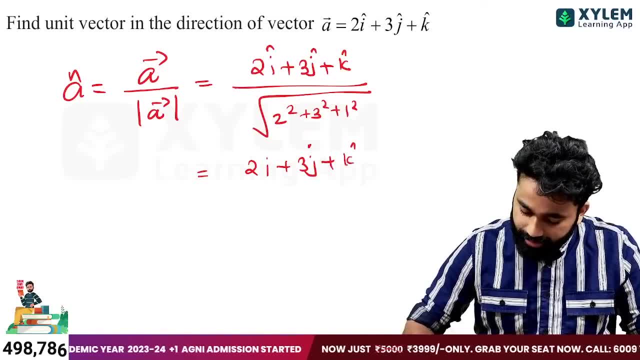 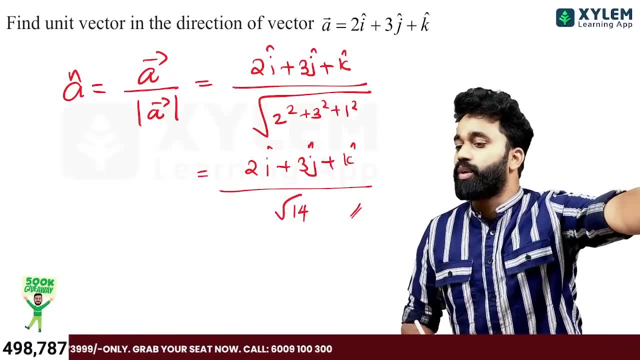 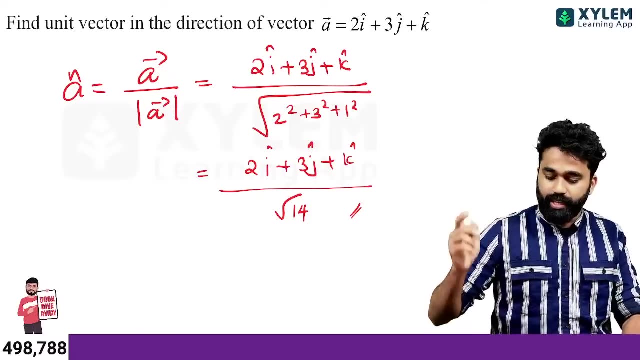 answer: yeah, 2i plus 3j plus K, divided by 1, 9, 13 root, 14, just a can of which it a question of didn't know. no, no, no joke, okay, okay, I'm not, okay, I'm not clear, I know, yeah, I need you, or, if I remember, typically the man over on the separate. 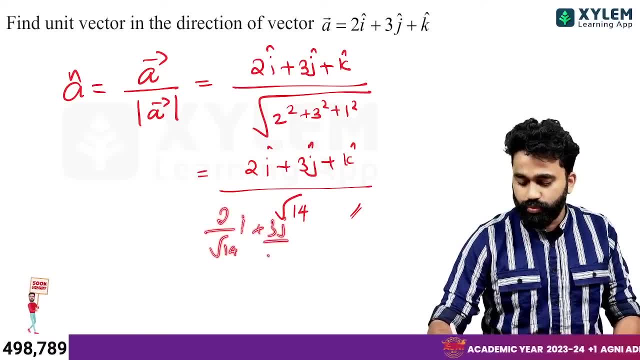 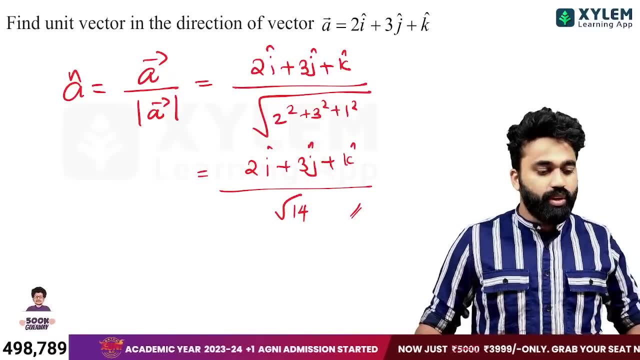 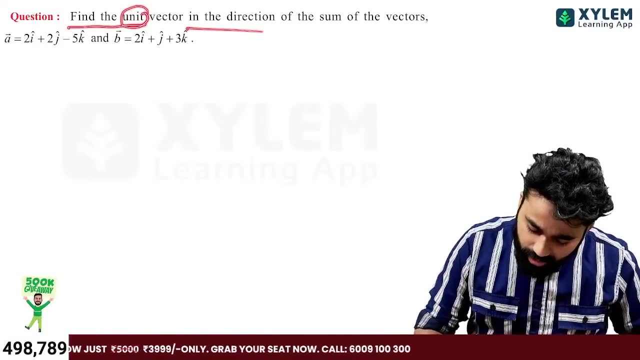 data to 2 by root of 14 I plus 3j by root of 14 K, J plus K by root of 14 K. satellite calculus occurred. could add to the new political or on the water right in the world, I don't know, the Jonah find the unit vector in the direction of the. 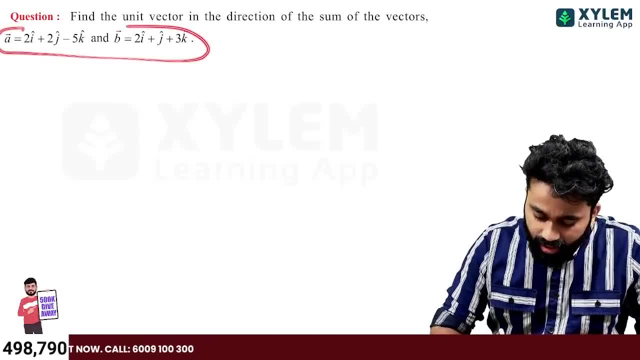 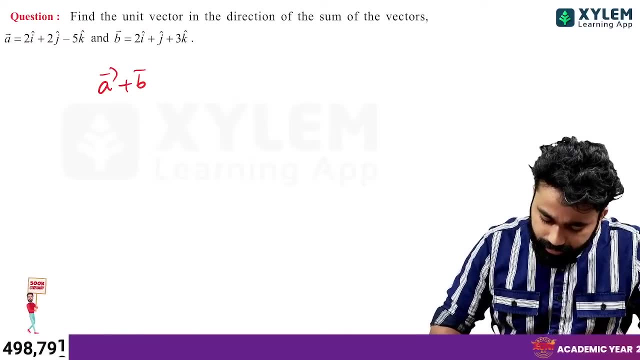 sum of the vectors eat under you can the gender vector girl, the sum in the unit vector. about our other, the? you know I had a some we're under. you know you need better important. I don't know, I don't know some country, Canada, I, you, I, you go to end. 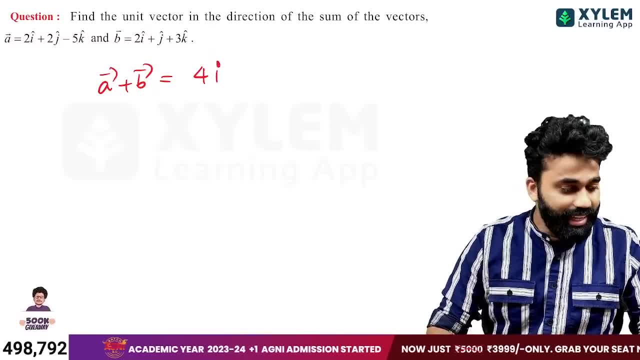 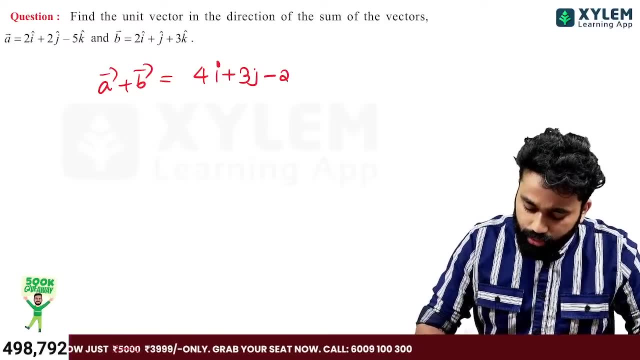 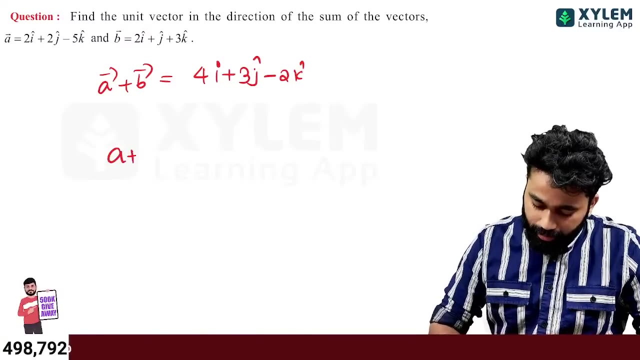 up listening to Nali I James, you go to end up less on the. that is 3j minus 5 plus 3, minus 5 plus 3 and minus 2 K. okay, it's not a a plus B and I'm okay, you didn't matter to tell you. each and I know can talk about it. I'm going to eat. 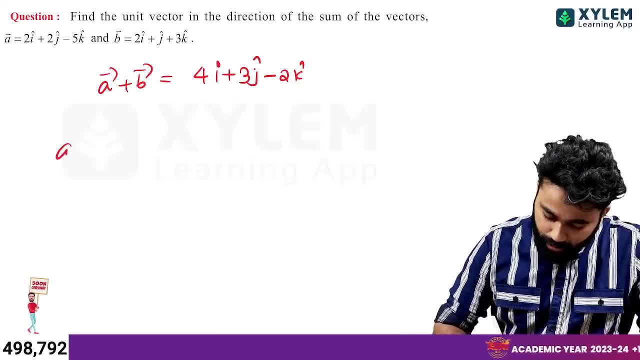 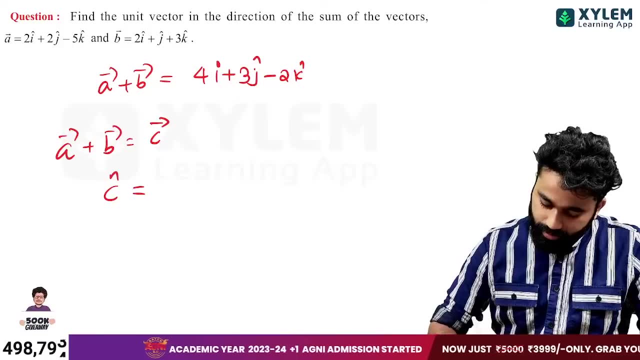 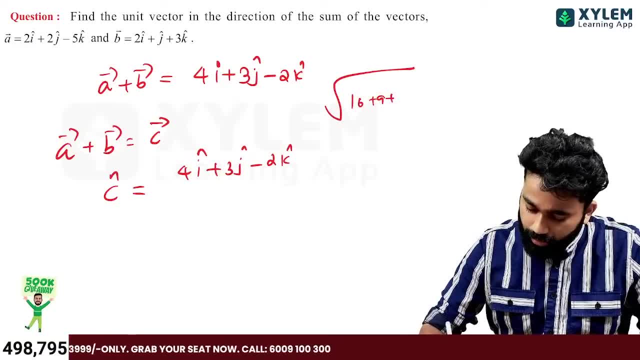 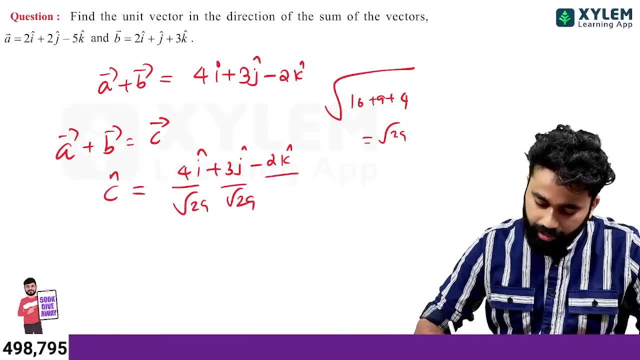 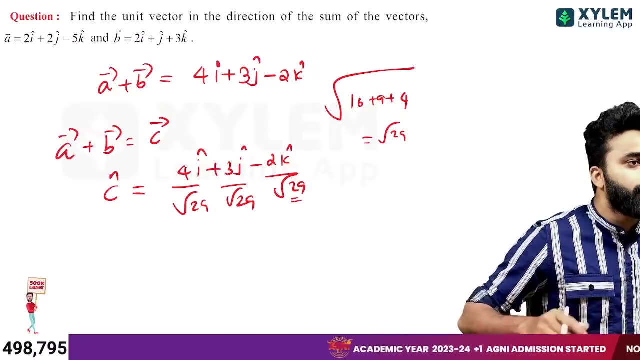 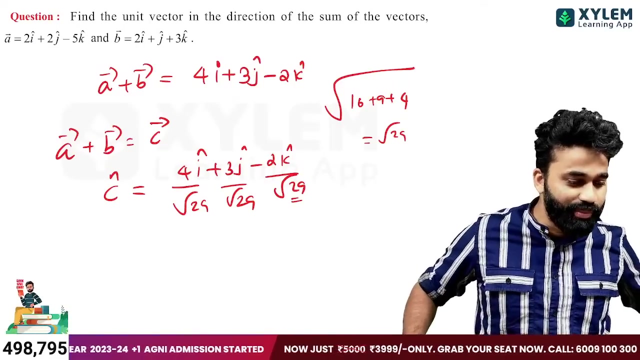 Danada magnitude under you for the nine plus on the day, plus booty, 29 by 29 and by sitting on a really yes, yes, sarsina, or thank you, sir Sina. clear, no doubt. ok, Sanju, only ok. I hope the idea is clear. 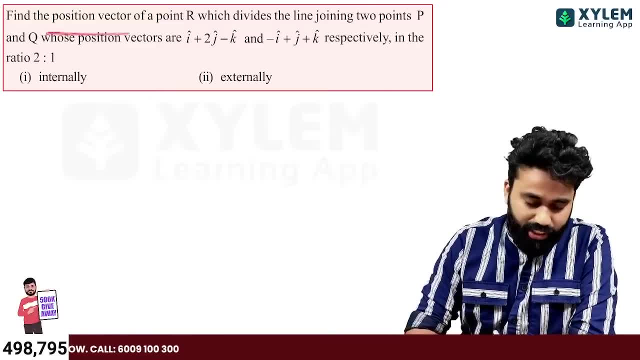 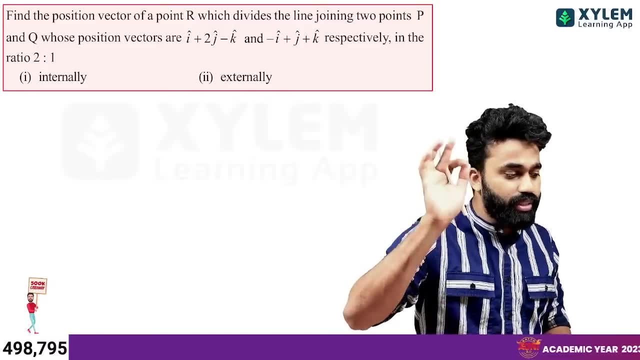 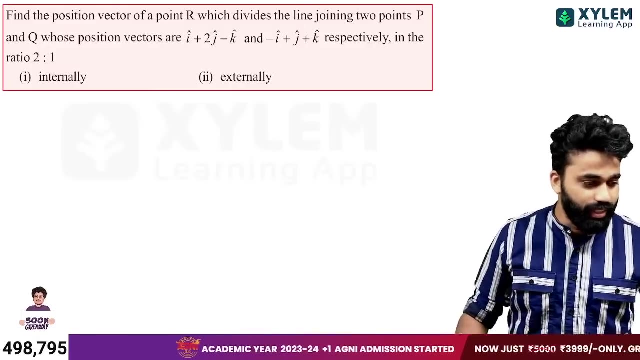 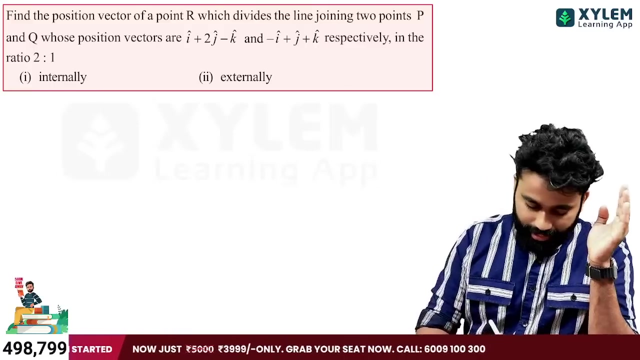 even if you haven't asked the exam, you can ask section formula: 7 marks. not like you think you are going to study. 7 marks: 4,99,000, 4,99,000. ok, if you have a question, you have to use yes. 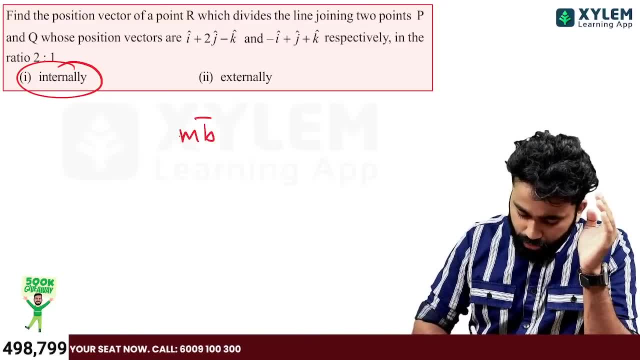 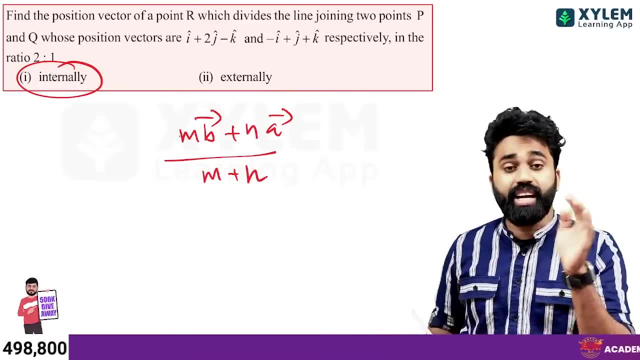 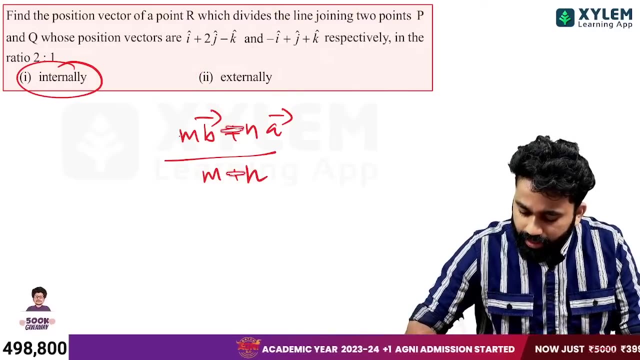 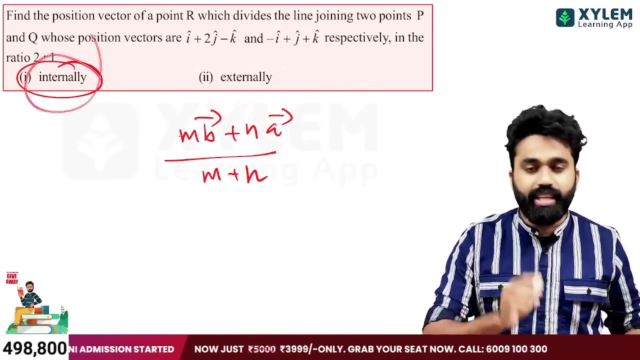 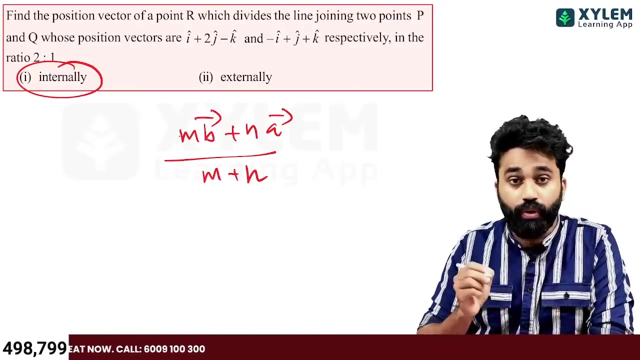 you have to use this equation: m b plus n, a divided by m plus n. this is the equation if it is internal. if given externally, only m b minus, there is no change. if given externally, use it. if not, use it internally, ok. m is 2, n is 1. 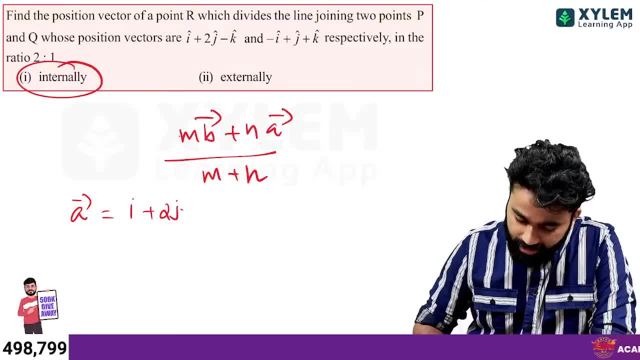 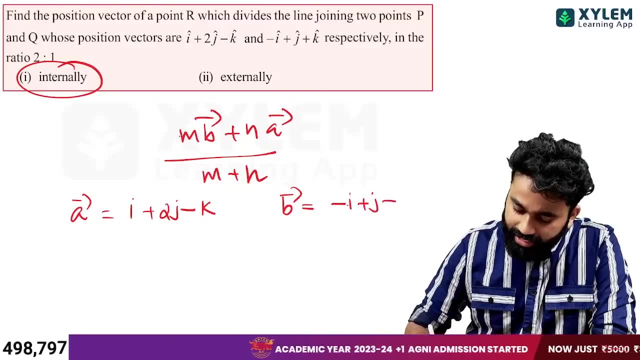 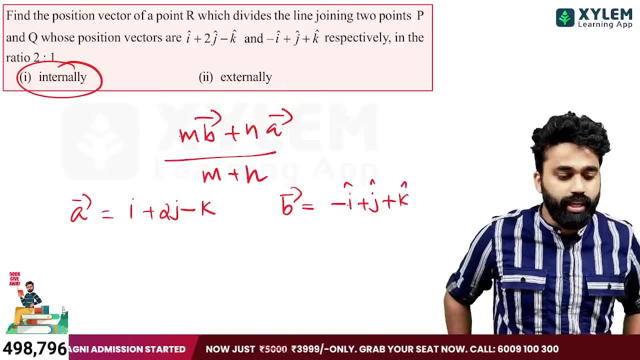 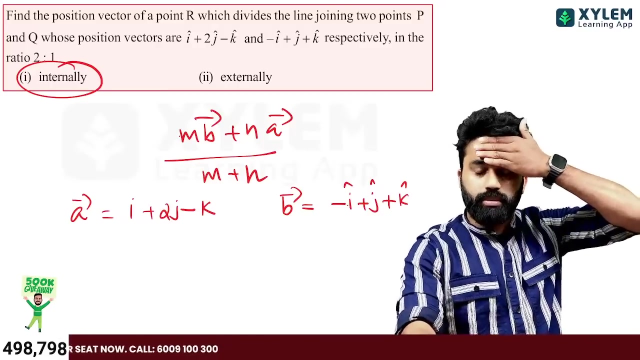 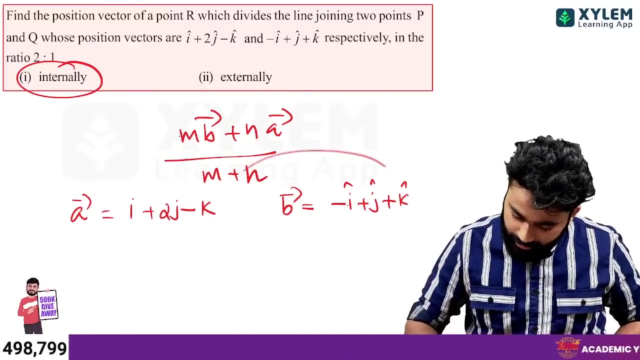 a is the first vector. i plus 2j minus k. b is the second vector, that is minus i plus j plus k. after this class you have to say m b plus n a, also m b plus n. a. m 2. b is the second vector. 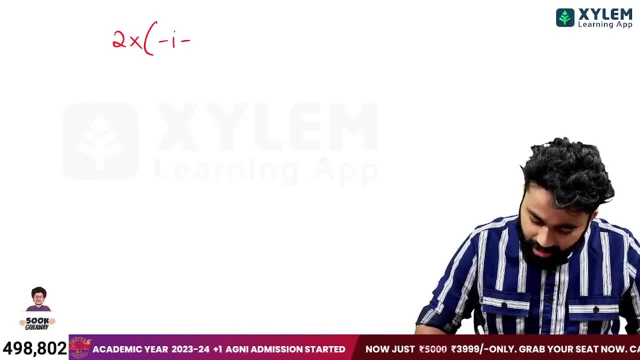 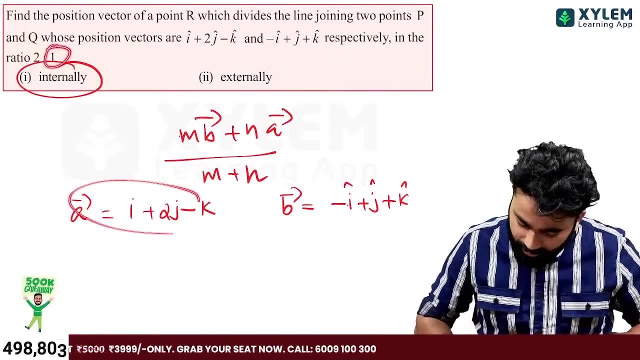 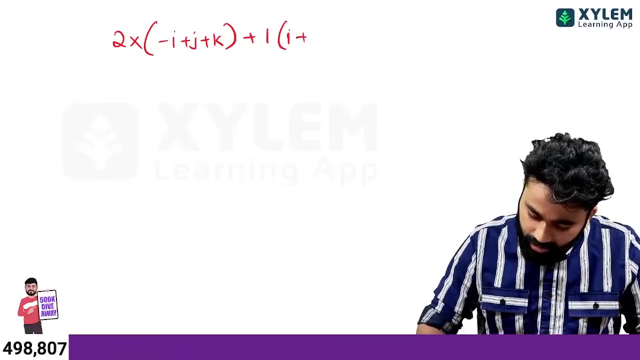 minus. i plus j plus k minus. i plus j plus k m b plus n a plus 2j plus 2k m b plus 2j plus 2k plus 2j plus 2k plus i plus 2 j m b plus 2j. 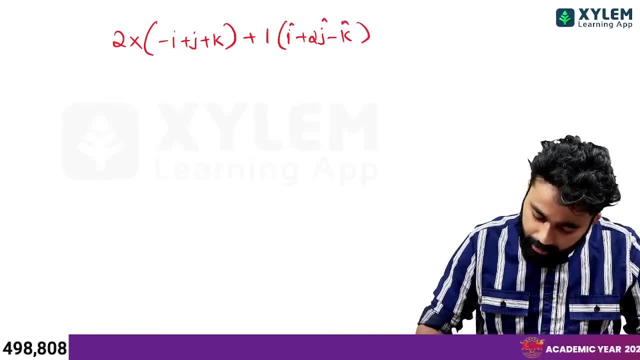 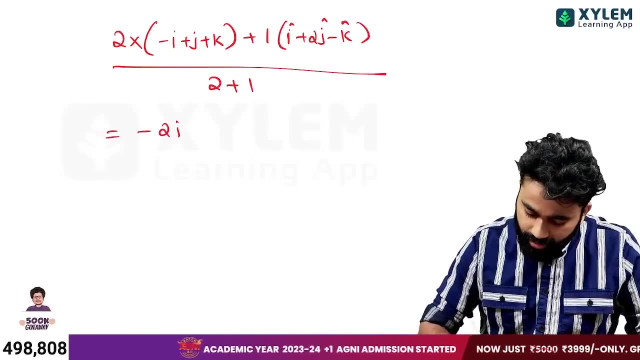 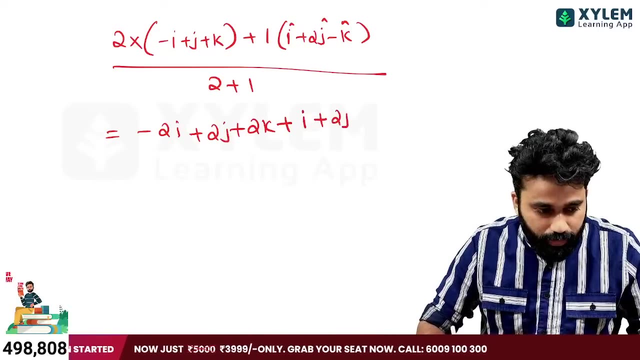 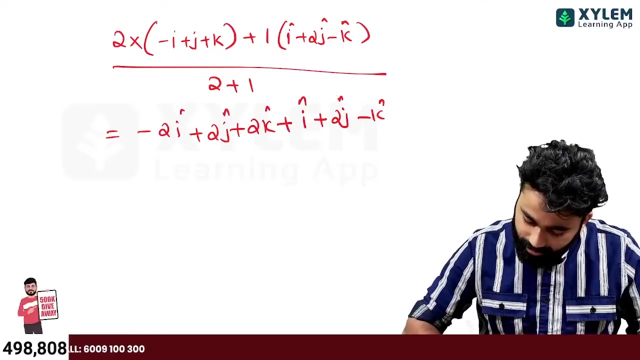 plus 2k, n is 1. 1 into n is 1. dont be scared of the ninth. I into: i plus 2j minus k. i plus 2j minus k, m, b plus n. a. divided by m plus n, j, Yes minus k. Divider by Now let's put the answer. What is the answer? Minus 2i. 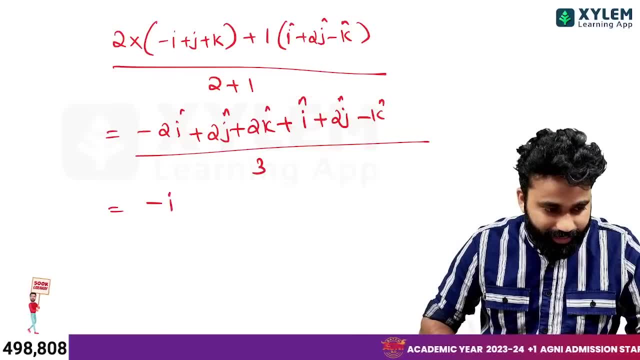 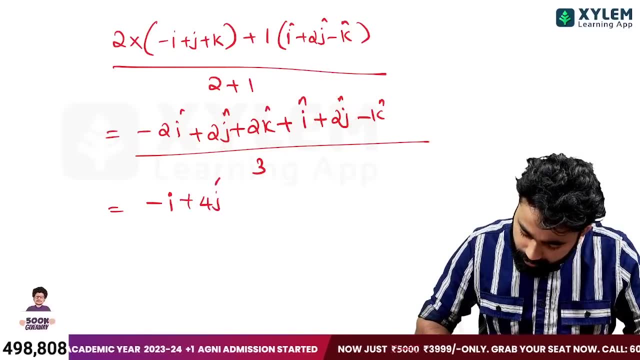 Minus 2i. plus i, That is equal to minus i. Okay, Plus 2j. plus 2j, That is equal to 4j. Plus 2k: minus k, That is equal to plus k. That is the answer. Bye, That is the final. 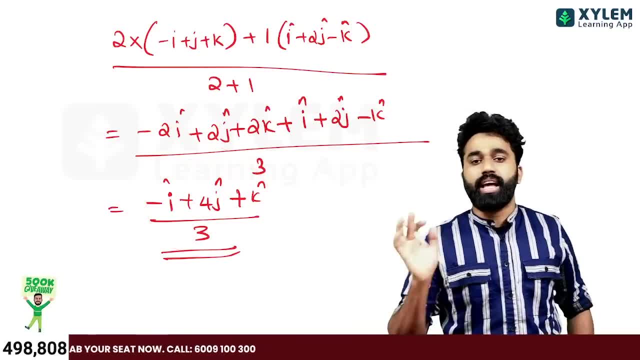 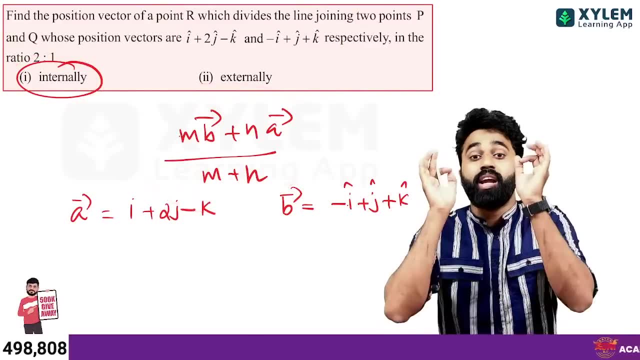 answer. If you do this, what will you get? You will get the direction. What do you say? You will get the internal vector. I will repeat it once again. Just remember this question: m b plus n a, divided by m plus a, Sorry, m plus n a. It is very simple. What can you? 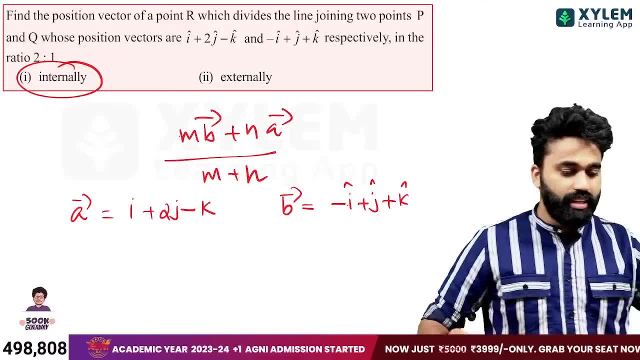 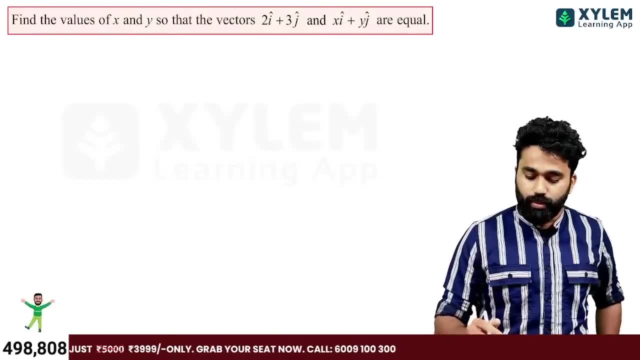 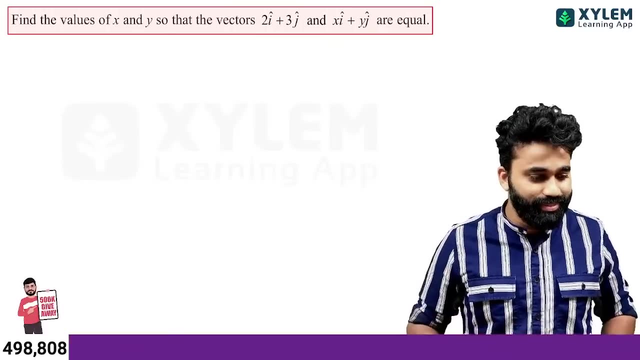 do. You can do this answer Okay, But I am not saying that you should take a lot of time to learn. But this section, formula, is a topic that you can learn if you think Okay. Now please do remember the article. you have just travelled, So if you finish this parable, 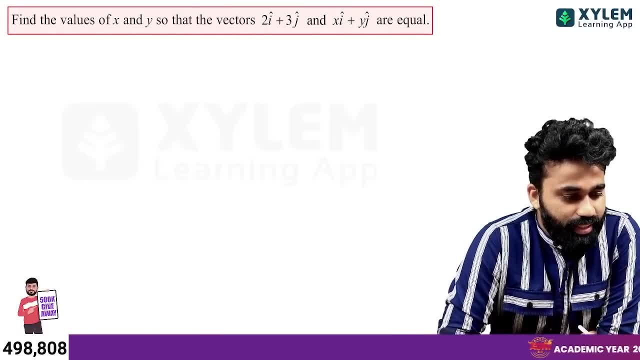 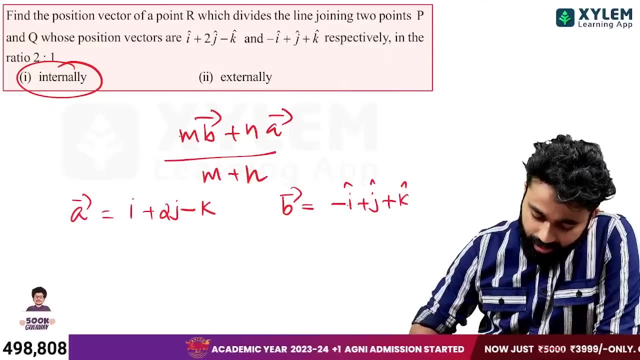 you show me the answer. Do you know the data you heard and how much you will get? Oh, yes, See, here, That is the answer. That is the first and everything is Porko One, then another and this Yes. Now, that is really simple. You will get the answer. 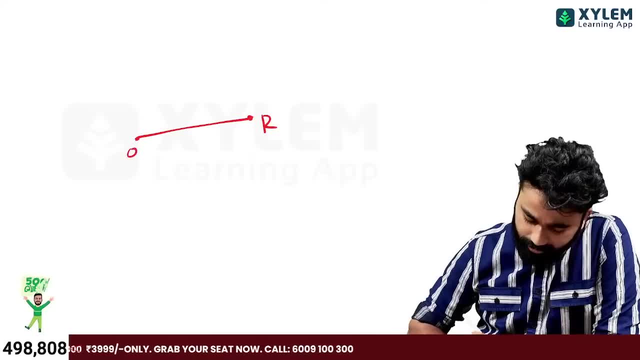 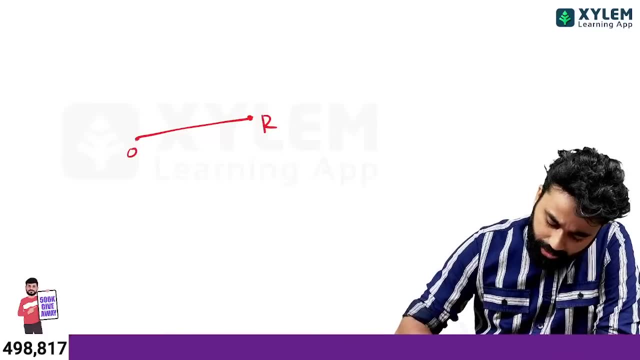 each time you talk about it, Then don't worry about getting wrong answers. And what will be the solution then? OK, joining two points: P and Q. P and Q is a line. P and Q- R is a point in this line. Okay. 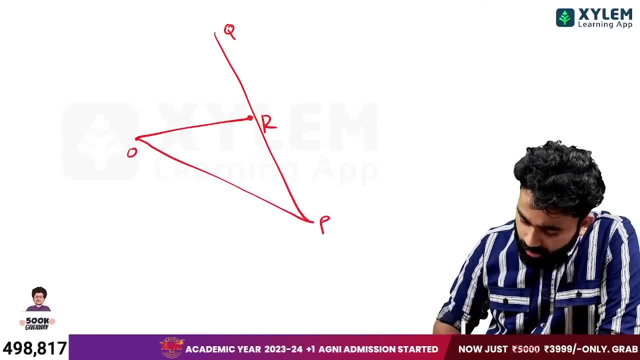 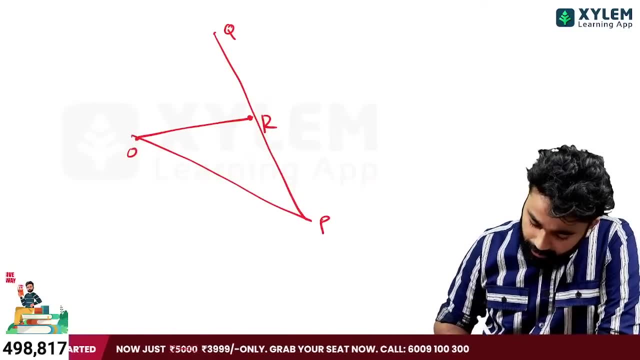 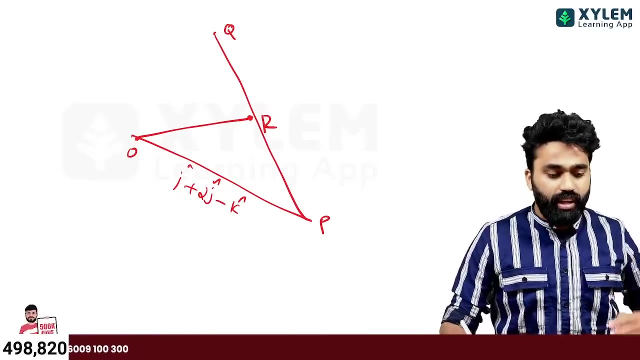 Position vectors are: The position vector of this is O. This is one OP vector That is equal to I plus 2J minus K. This figure is coming. This figure In the internal section formula. this figure is coming In the section formula. this figure is coming. The second: 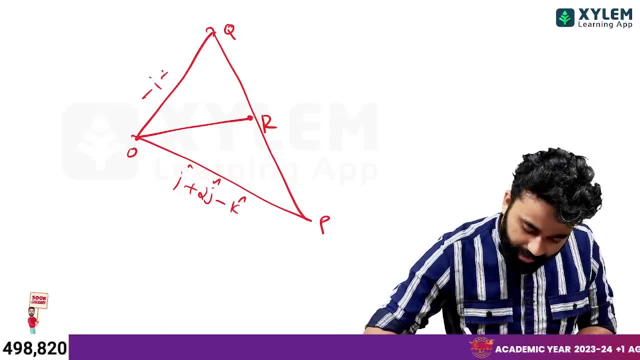 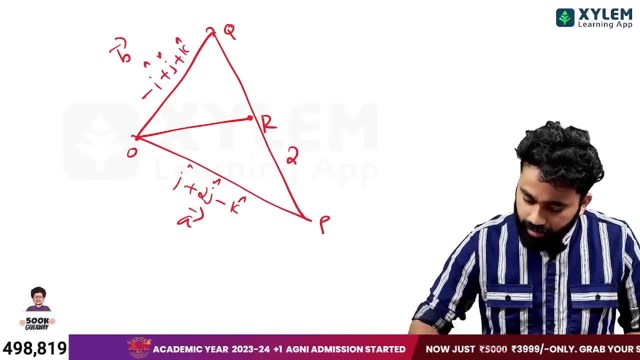 vector is minus I plus J plus K. You can see in the textbook: Minus I plus J plus K. Okay, This is A vector, This is B vector, This is M and this is N. A comes here and M comes there. 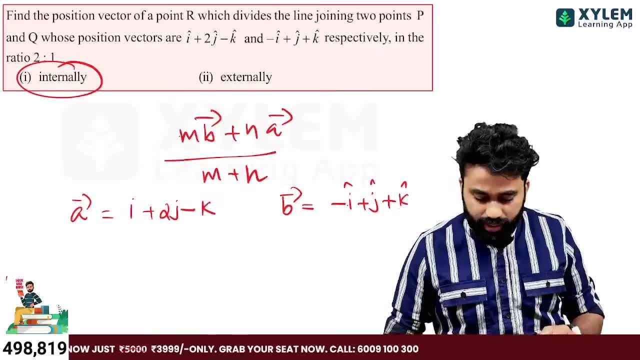 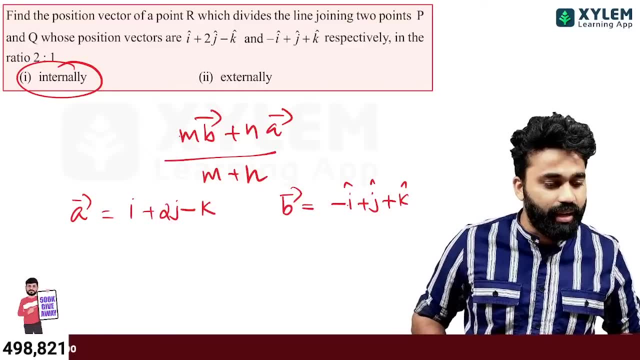 We will answer with this External equation: MB minus NA Minus NA divided by M minus N. That is all. It is not that important. If you want, you can do it. You can look at the internal and external equations. In the internal equation this P and Q will be. 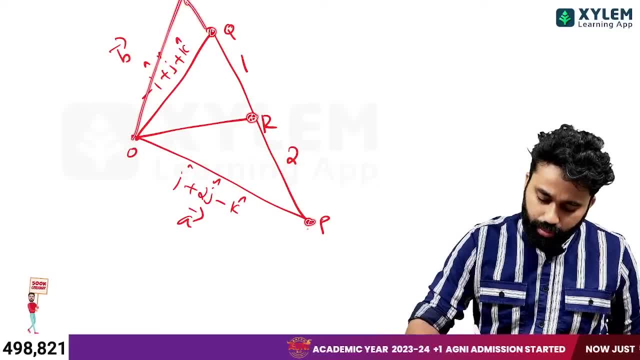 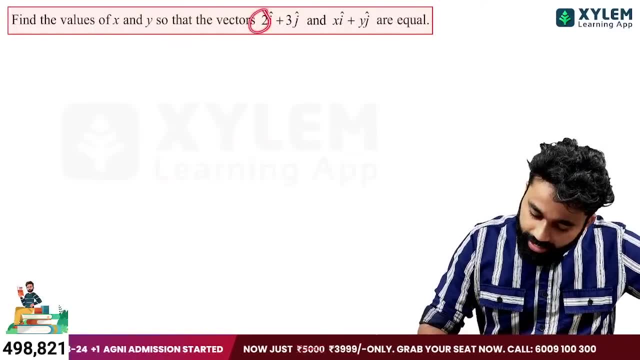 inside the Q. If it is external, this P and Q will be outside the Q. R is the change. So guys pay attention. Yes, X is 2.. X is equal to 2.. Y is 3.. This is the answer Full. 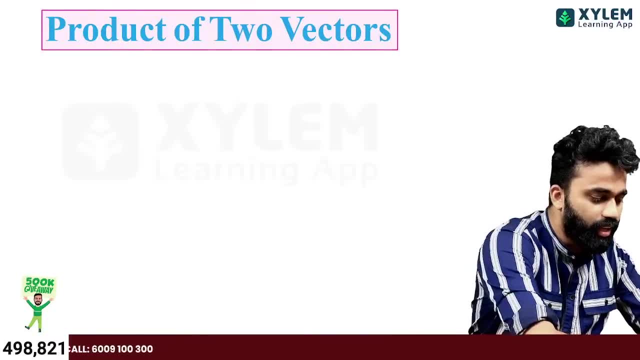 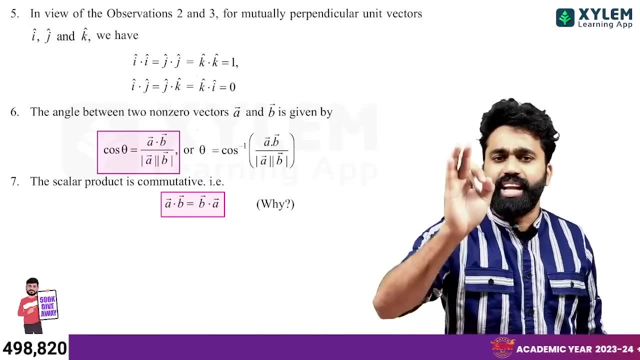 mark. Okay, Maybe you can ask a mark. Okay. This is the most important Guys, if you touch. If it is not clear enough, you can take a look at it again. Now pay close attention. here There are two topics. 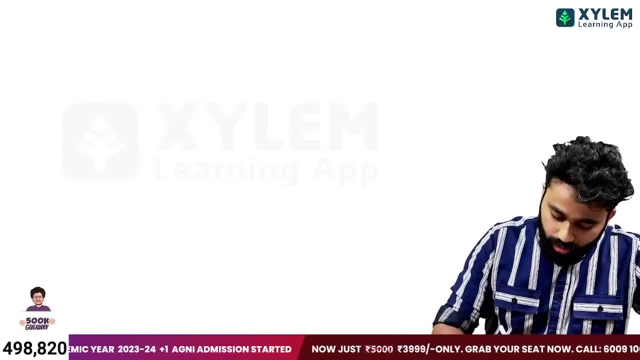 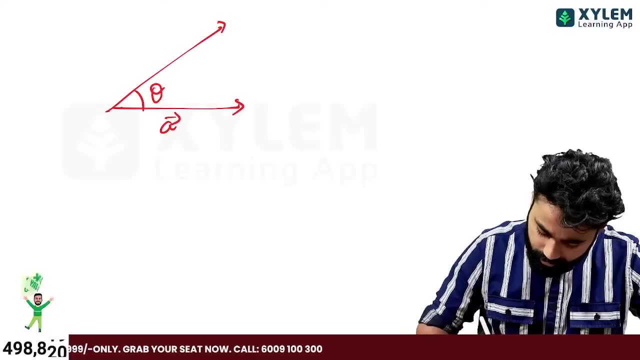 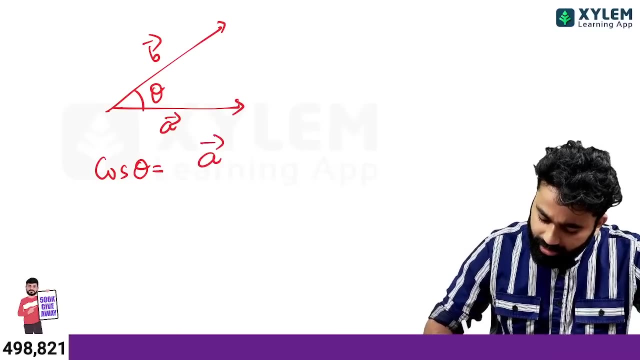 Dot product and projection. Ask that That's all Two vectors. The angle between them is theta. Then the angle between these two angles, cos theta, is equal to the dot product of those two vectors. Magnitude of A into magnitude of B. 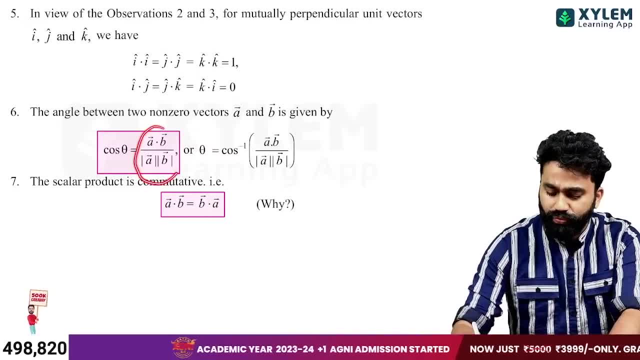 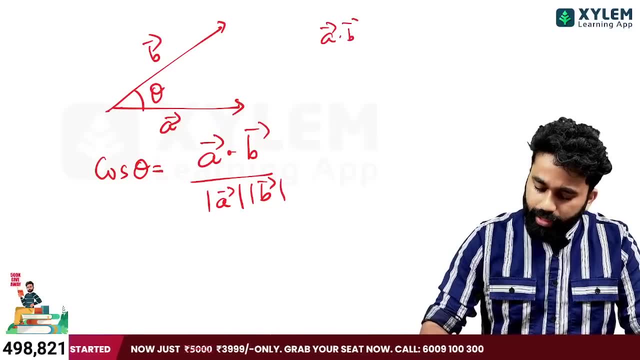 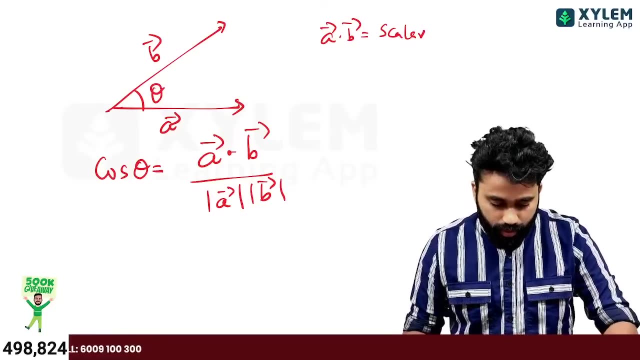 A dot B, divided by magnitude of A into magnitude of B. Remember one more thing: A dot B is always a scalar, It is a number. It is always a number, It is always a number. I will show you a question related to this. 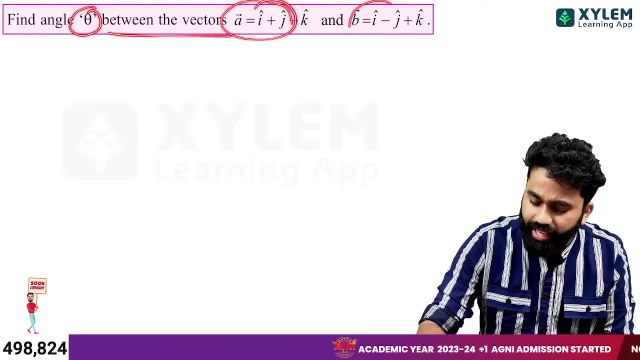 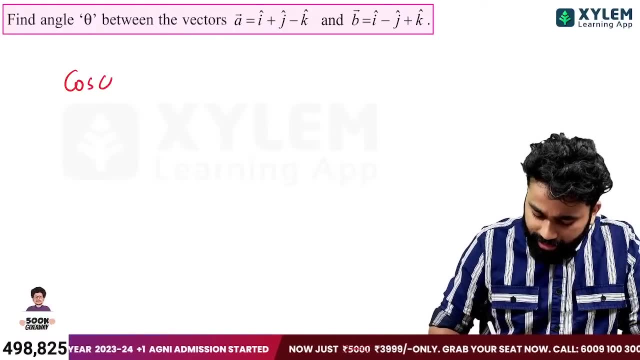 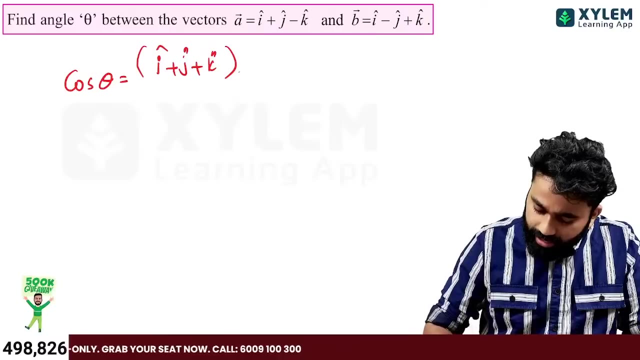 Find angle theta between these two vectors. The angle between these two vectors. The angle between these two vectors is cos. theta is equal to A dot B. A dot B. The first vector, Dot The second vector, A dot B, Divided by: 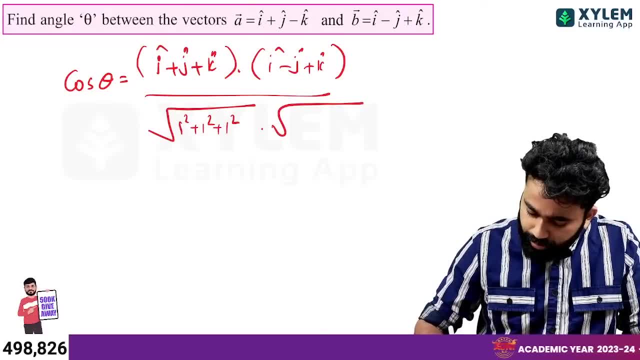 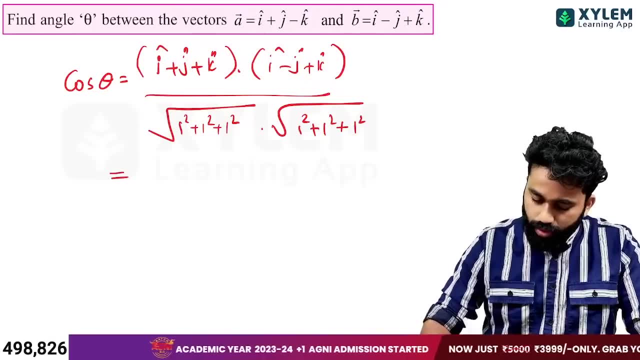 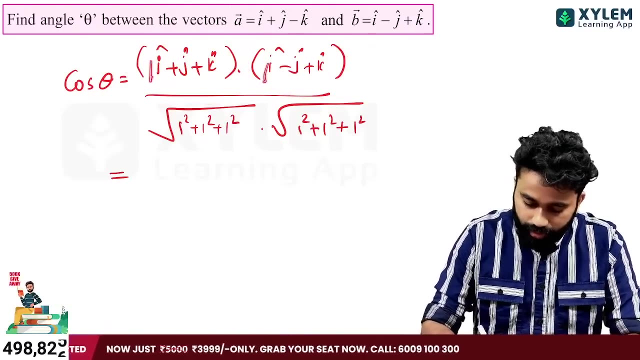 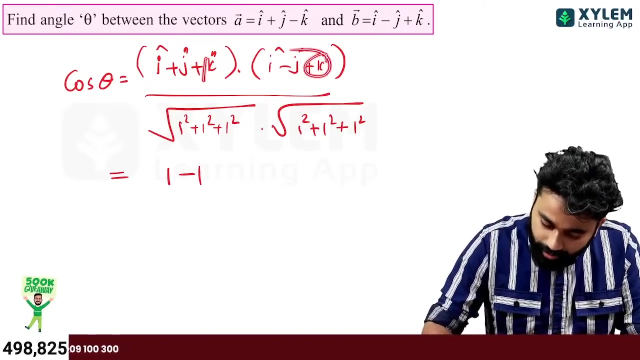 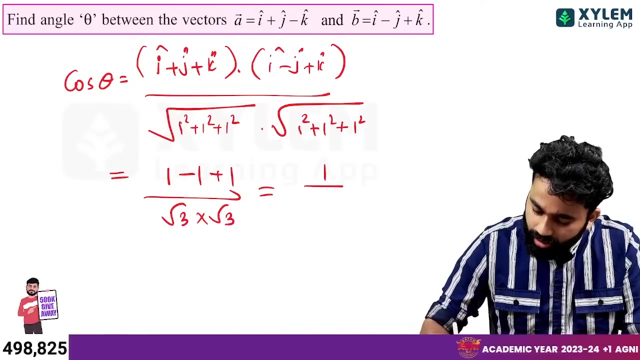 magnitude of A into magnitude of B, Two products 나왔습니다: Magnitude, velocity, r-scan values, A-scan value ested. So the product of is 0 itself Bit of. What's the difference between root 3 and root 3? that is equal to 1.5?. 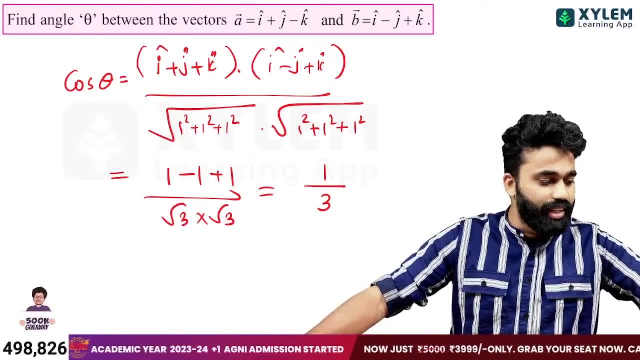 I think it's because of your model exam, right, I came to you live at the end. Then you said, sir, you don't have any energy. Sir, sir, what is it Sir? I have asked a lot of questions about headache. 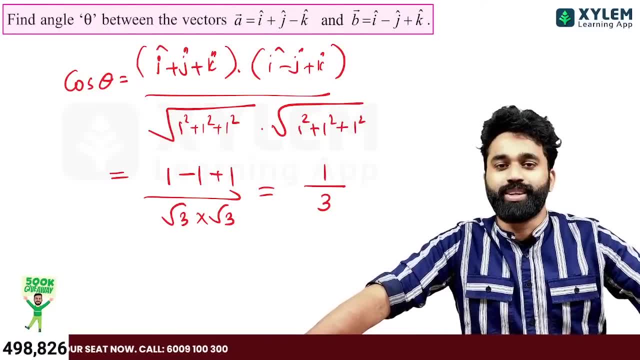 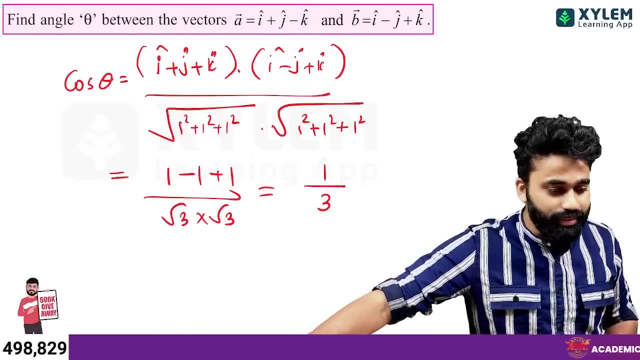 But pay attention to one thing: Have you ever asked any of the questions we asked Whether it is 3D vector? any matrix- my son's matrix- is directly like that Vector and 3D. Yes, yes, yes, yes. 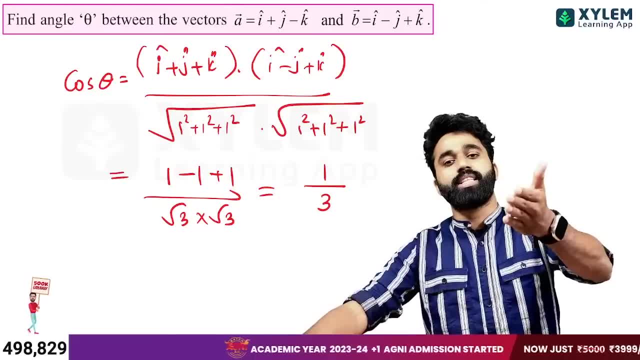 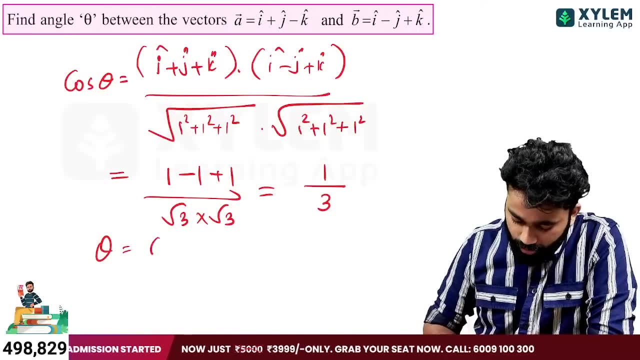 Application or derivative. There is no need to say anything else. I told you that the question to see the intervals is definitely there- What to do. But the question is not like that. Theta equal to cos inverse of 1 by 3.. 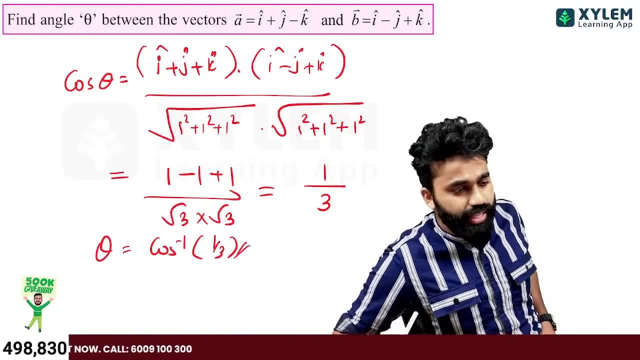 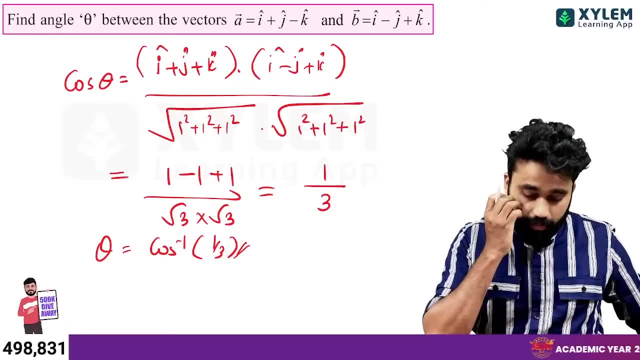 Is it set? Is it set? Is it set When we should take 1 is to 1?? When we take 1 is to 1, the midpoint is 1 is to 1.. Okay, Sir, is it minus k? 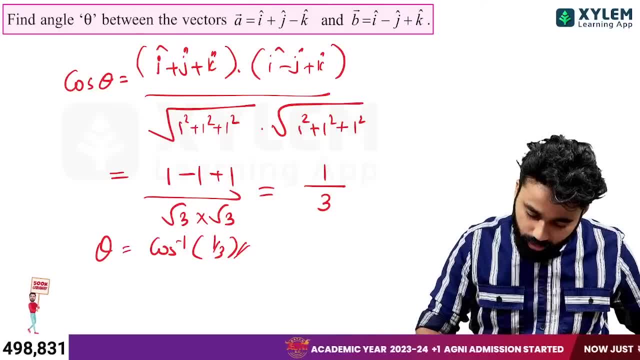 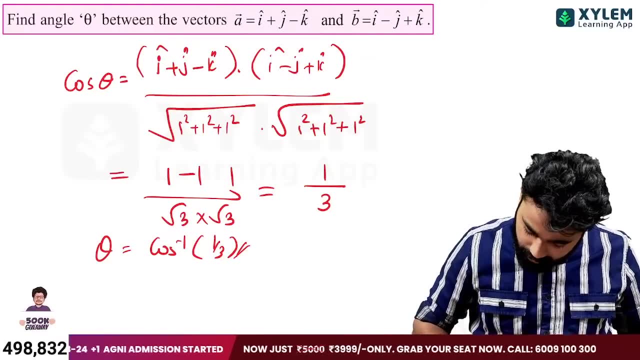 Where is minus k? Yes, here is minus k. Sorry, here is minus k, So here is minus 1, right, Here is minus 1.. Here is minus 1.. Set, set, set. Yes, I think it is okay. 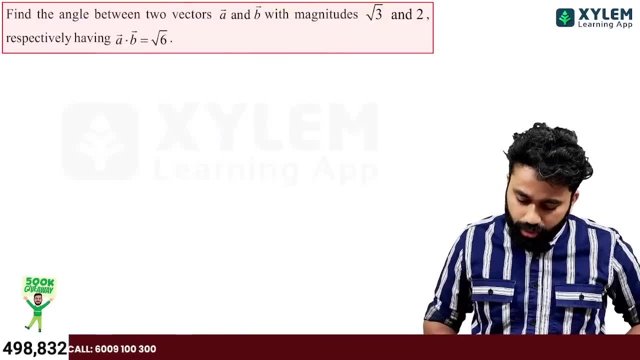 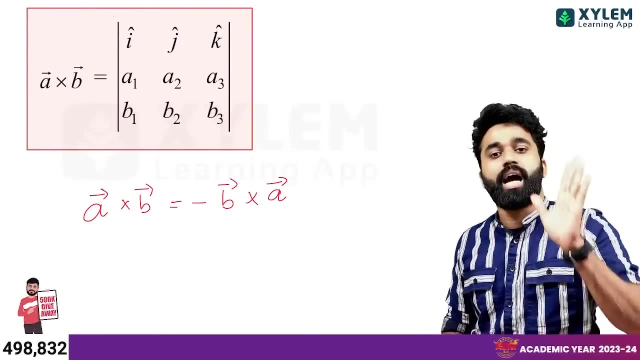 I think it is okay, guys, Pay attention. Pay attention to the next question, guys. Yes, this is not good for you Now. it is cross-product, Like this projection and cross-product. Those two topics are over. We will come to such questions. 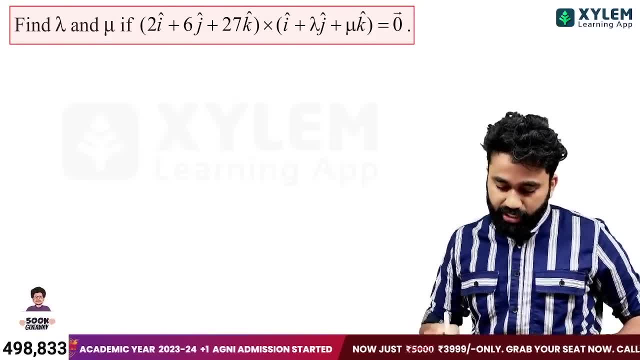 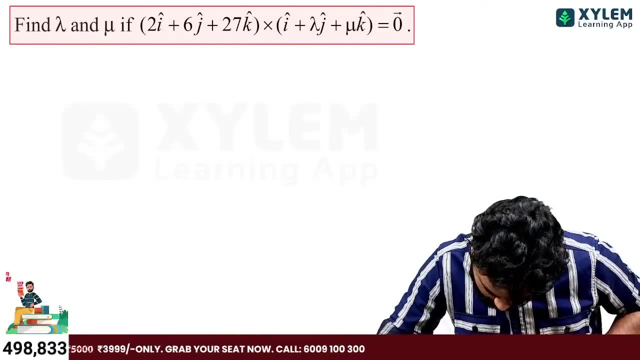 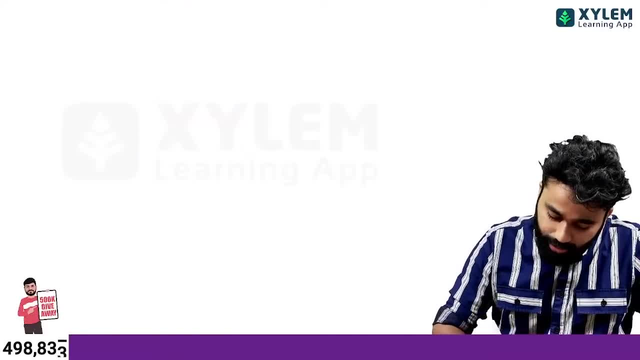 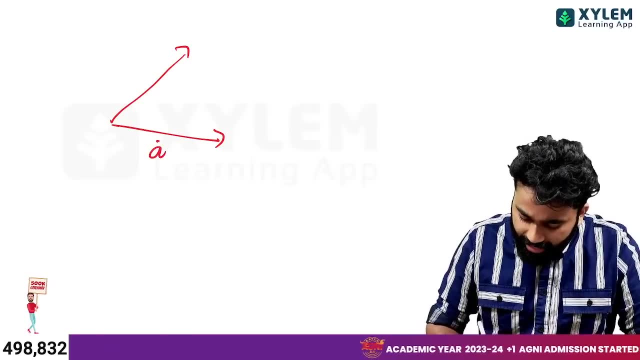 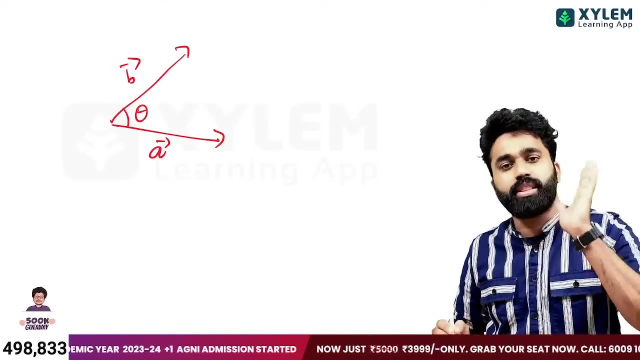 Next one, Second one: I will do projection now. If the question is like this: there are two vectors. Guys, there are two things to find the angle. This is the vector A, This is the vector B. There are two vectors. 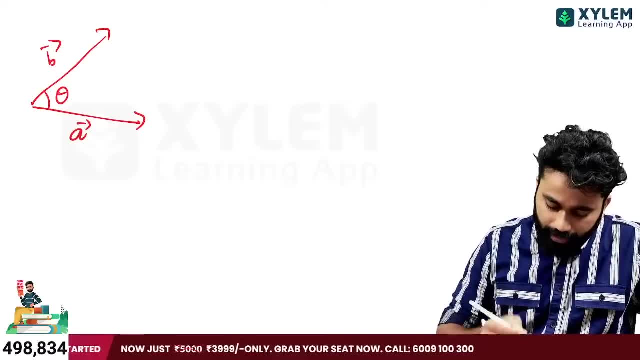 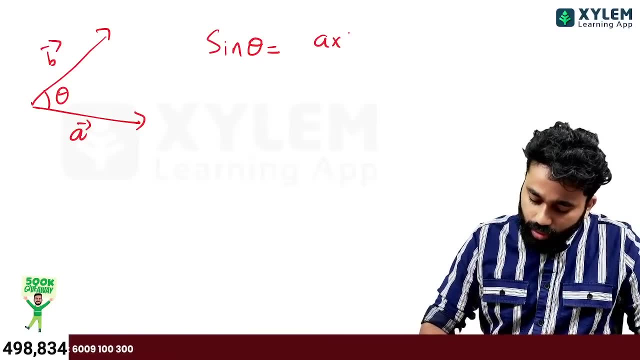 First we will use cos theta. If you have used cos theta now, if you want, you can use sin theta. It is not a mistake. Sin theta is equal to a cross b divided by magnitude of a into magnitude of b. 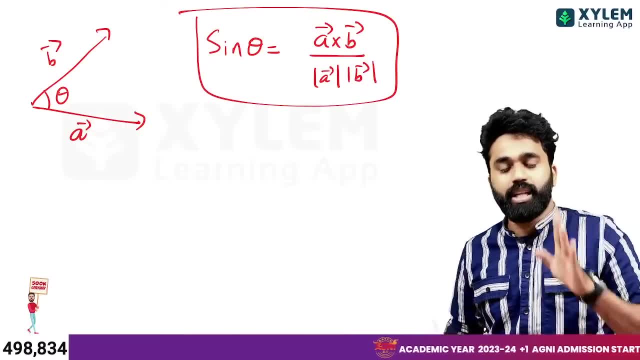 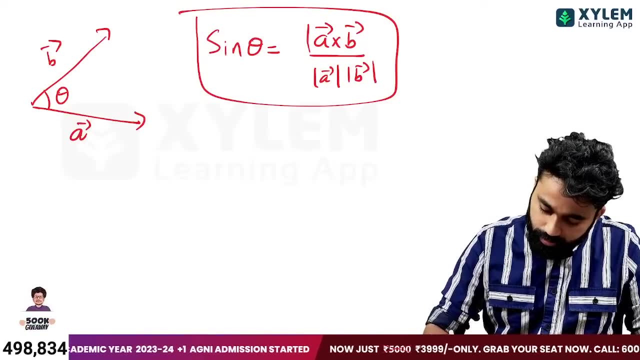 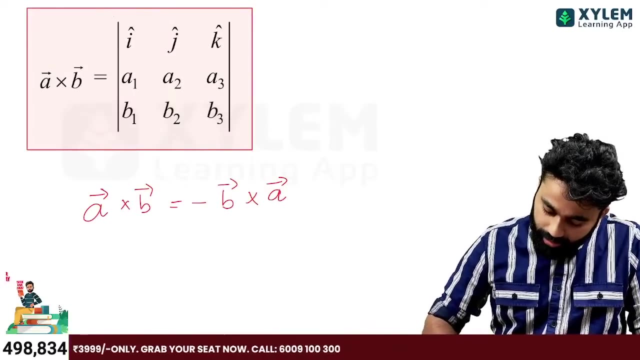 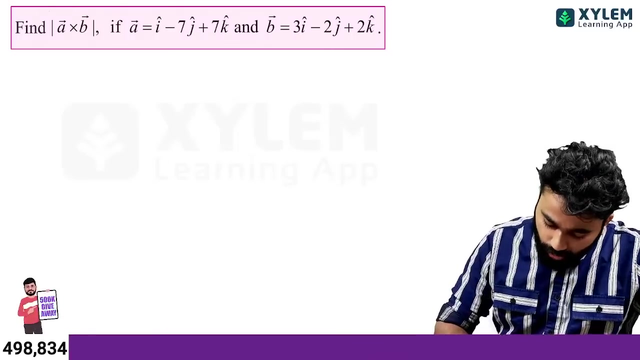 This is sin theta. Very important, very important. What is sin theta? a cross b divided by magnitude of a into magnitude of b. It is more or less like that. Okay, Magnitude, simple. Let's look at the answer to this question. Yes, find A cross B first. First, I'll show you how to find A cross B. So to find A cross B, you have to use the usual. 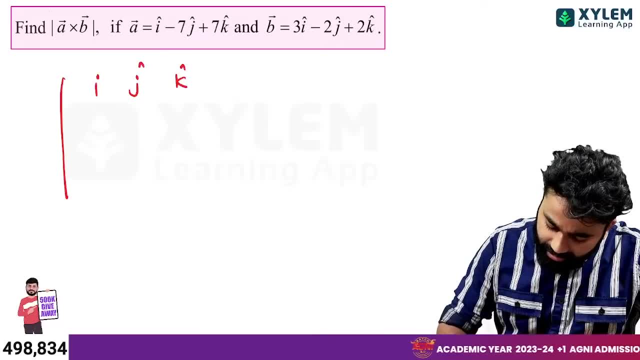 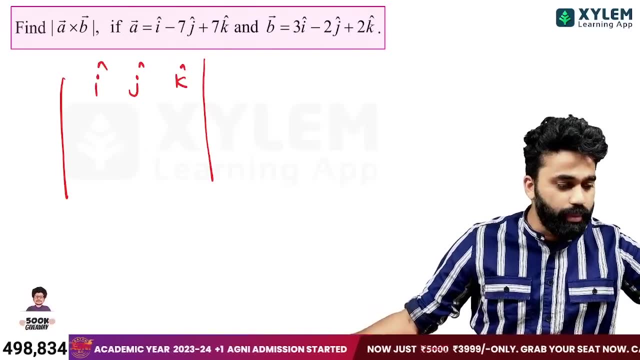 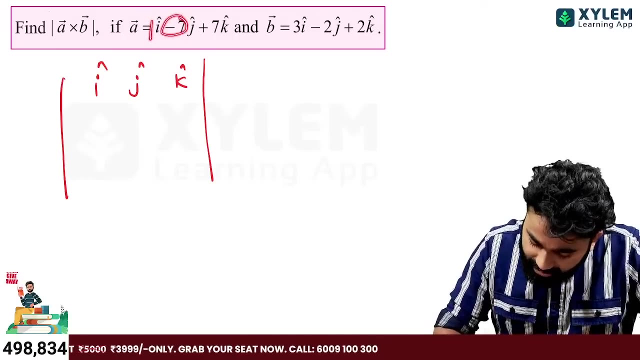 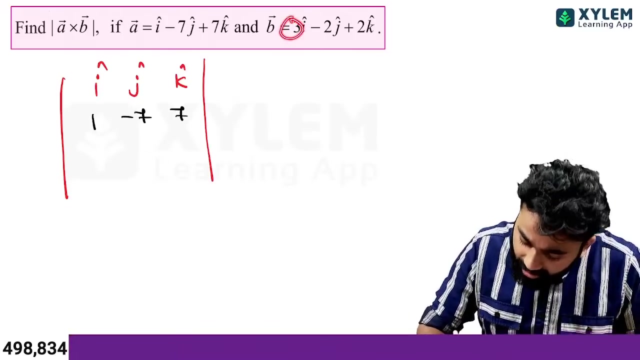 determinant method: IJK, IJK. You have to learn this, children. This is something that comes to your exam 100%. This topic comes to your exam 100%. This topic is called IJK. First, write the components 1, minus 7, 7.. 1, minus 7, 7.. Second, write the topic: 3, minus 2, 2.. 3, minus 2, 2.. As usual. 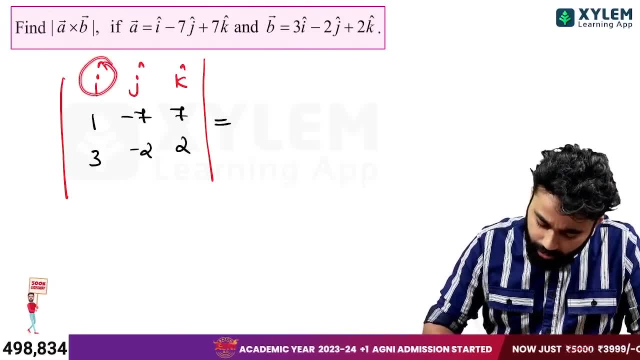 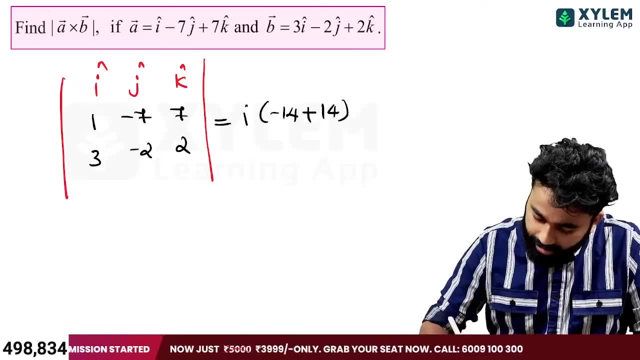 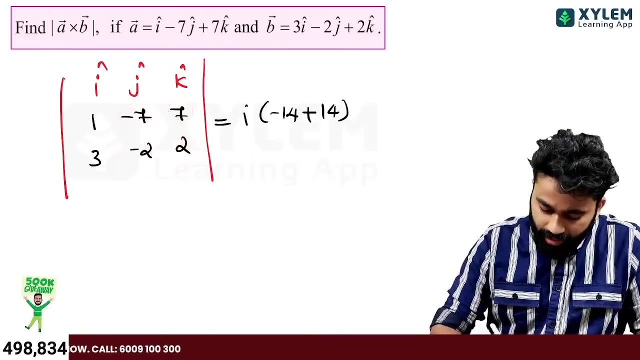 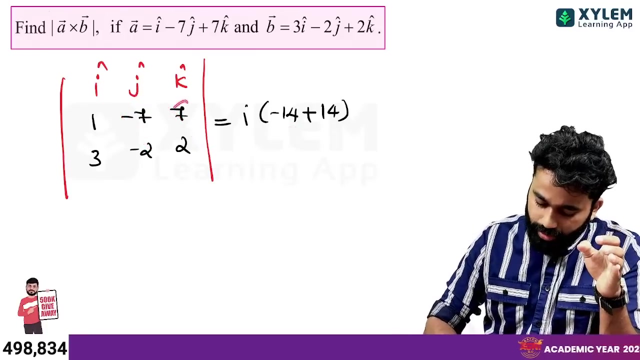 remember, I into the usual determinant, I into minus 14, plus 14.. That is minus 7 into 2, that is minus 14, minus minus 14.. I repeat again: Take these two numbers and divide them and get minus 14.. Then, like an equation, take the minus and add these two numbers and divide the number and get the minus. 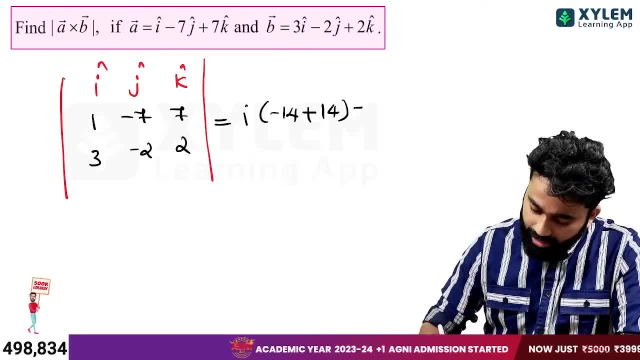 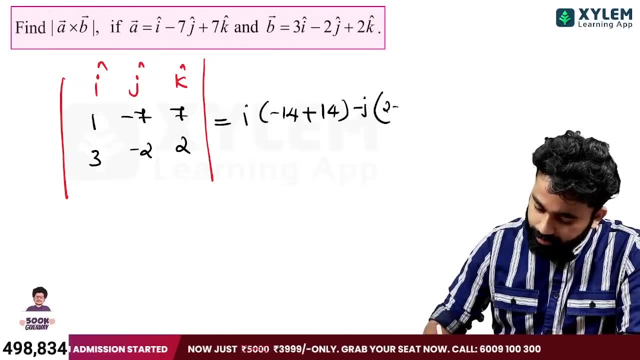 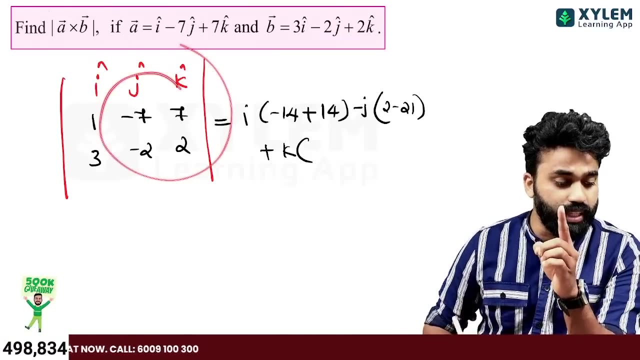 The two minuses come together and become the plus Next automatically. take the equation You know: minus J into 2 minus 21.. Plus K into Do you know which exam this is? Which exam is this? Which exam is this? 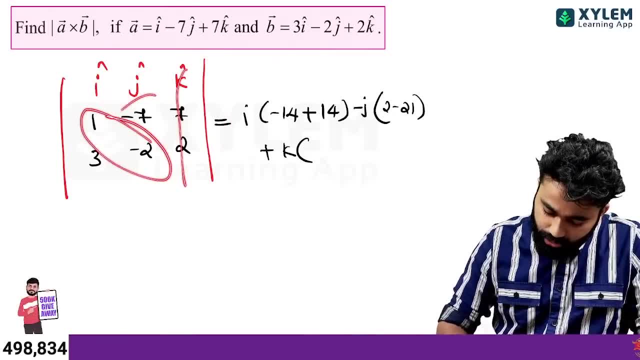 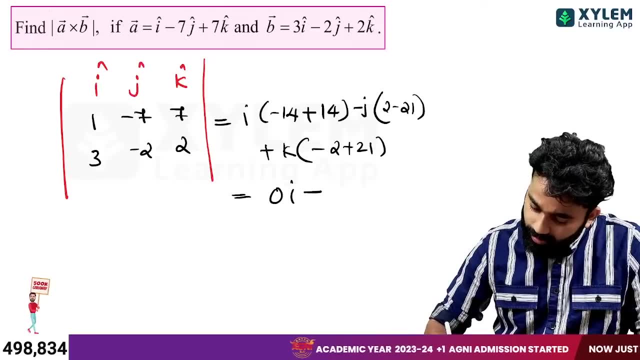 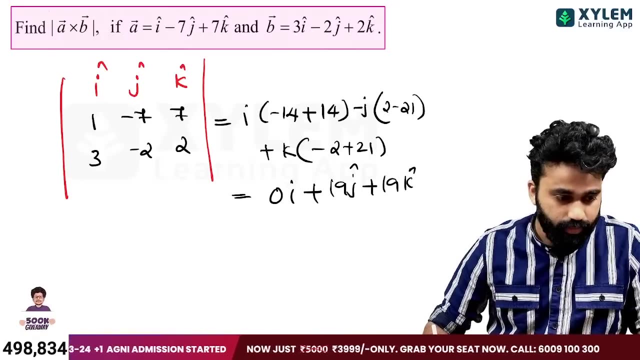 Which exam is this? Write this exam Minus 2 plus 21.. What will you get? That is equal to 0i minus minus plus 19j plus 19k. Yes, Yes, Yes, Minus 14.. Yes, 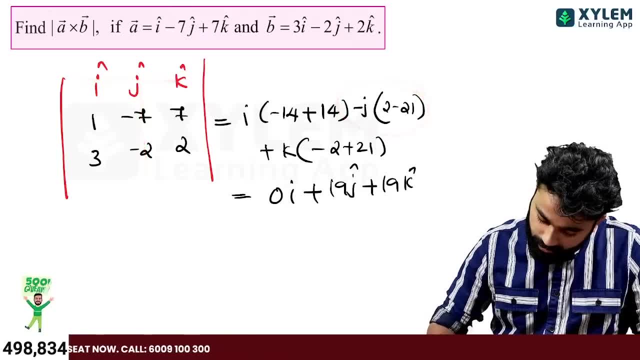 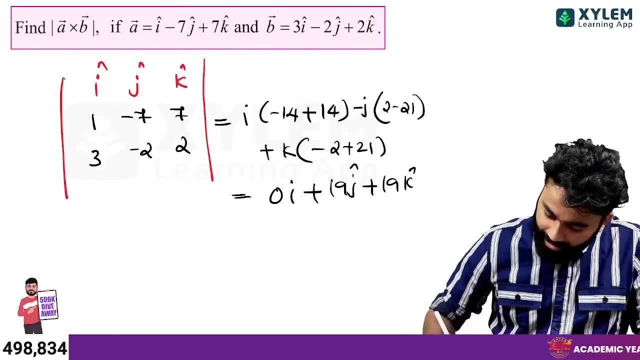 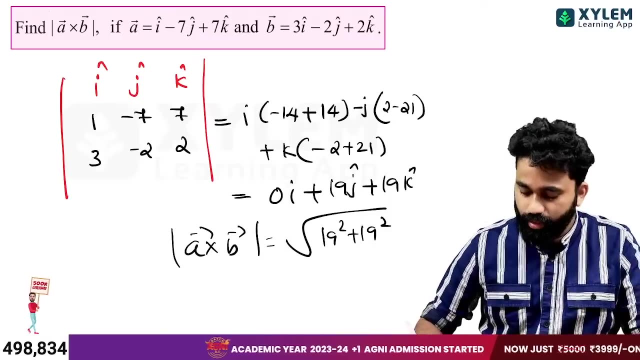 2 minus 21.. Correct: Minus 2 plus Yes, Correct. The magnitude of this is: The magnitude of this is magnitude of a cross b is equal to root of 19 square plus 19 square. That is 2 root. 2 root 19 square. 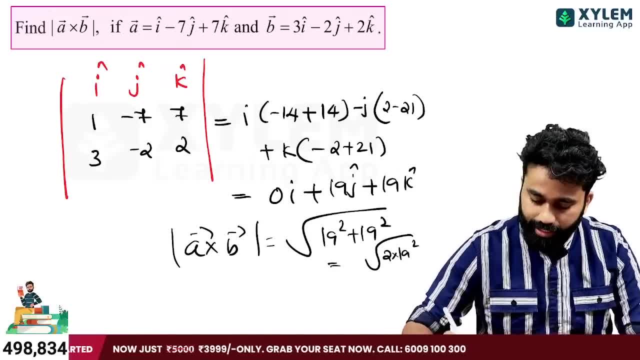 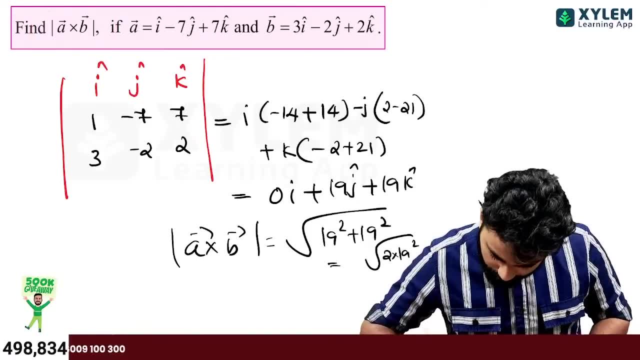 So 19 root 2 is the right answer. I will make it short. Yes, It is a Christmas exam. The same question came to your exam. I will show you the question. Do you remember that? Yes, Same model. 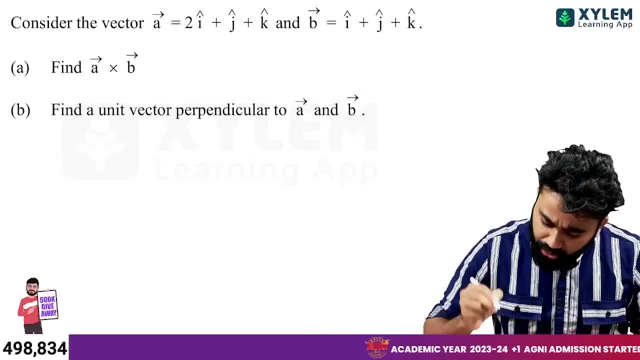 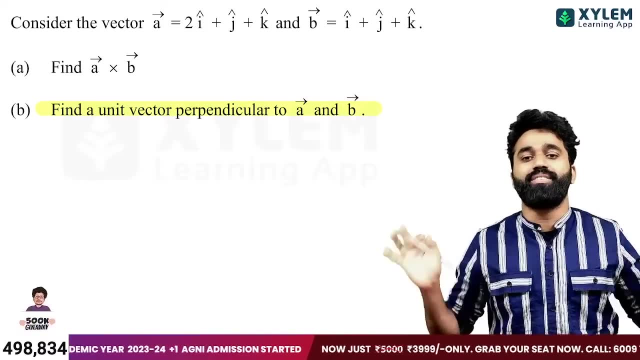 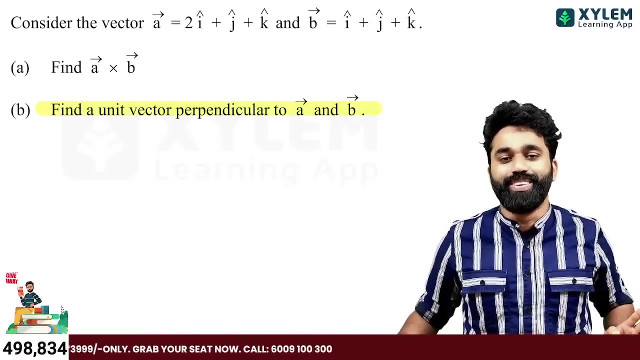 Children don't study 100%. The most important, The most important, is the question. I am trying to understand This question. This is called Javan Vector. Cross product vector is Javan Vector. Children pay attention. Look at the Javan Vector. 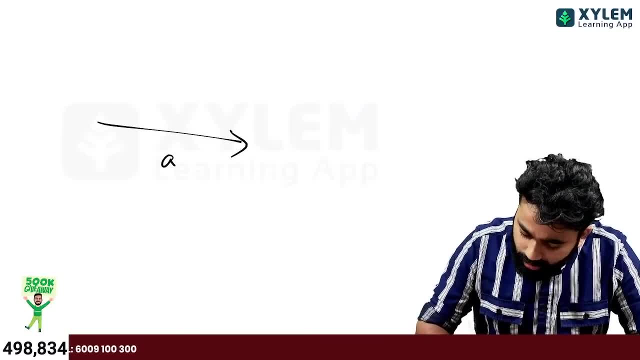 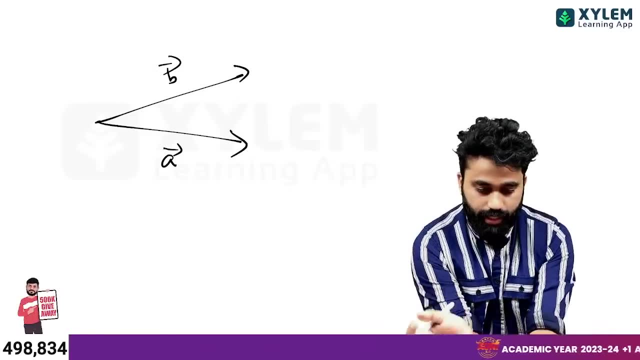 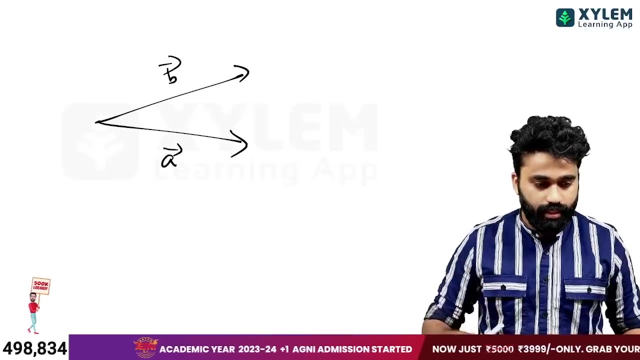 Do you know what is cross product? Two vectors in Tamil, This Javan Vector is. It is a vector that suicide Genau. I was told. 2 vectors: One to the right is 1,, two to the left is 1.. All two 0's. 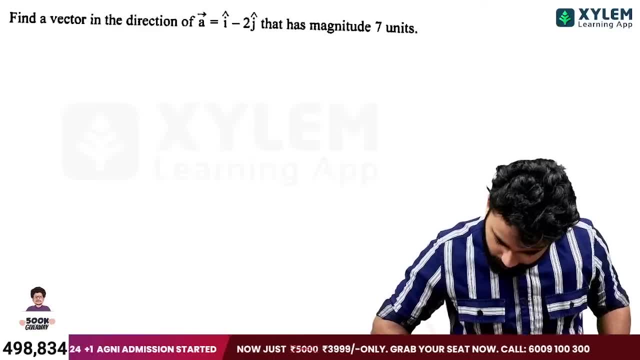 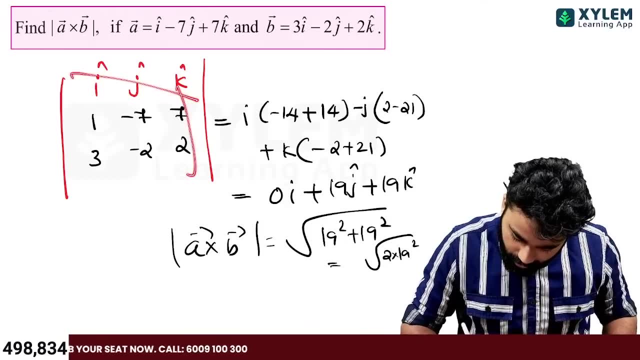 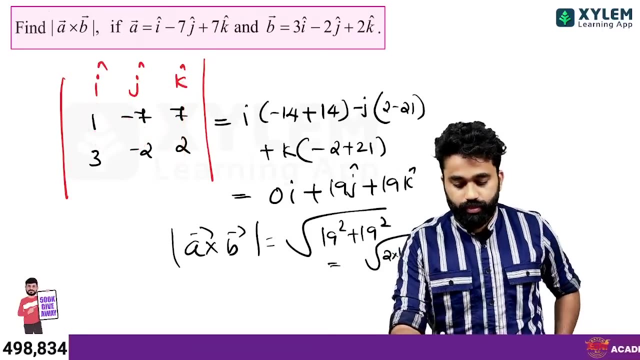 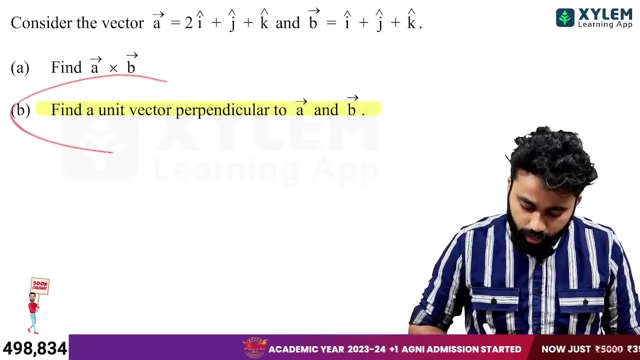 Aren't they Minus 21?? Let me see the question again. Look at the list. There is K right here. Let me see: Press the campus: Minus 2 plus 21.. Minus 2 plus 21.. No, Minus 21.. Where was it? This is the question. 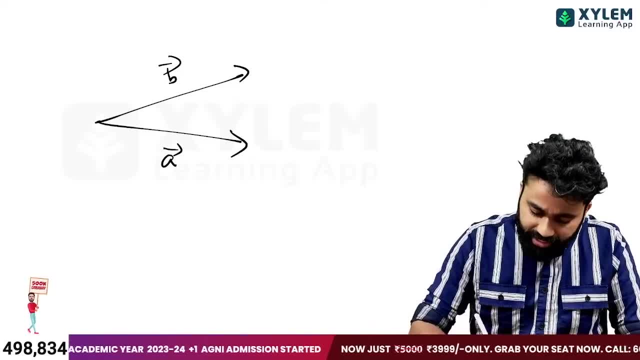 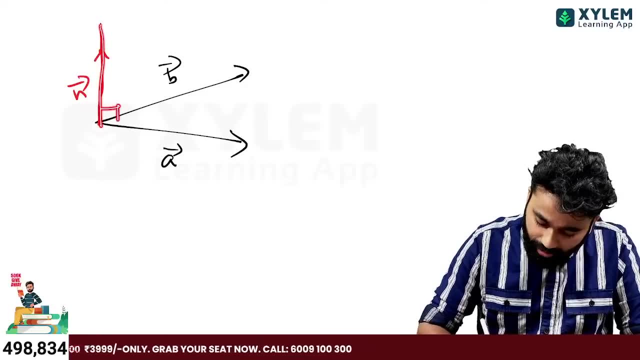 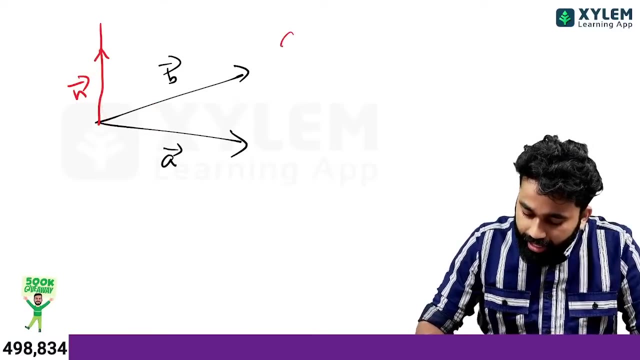 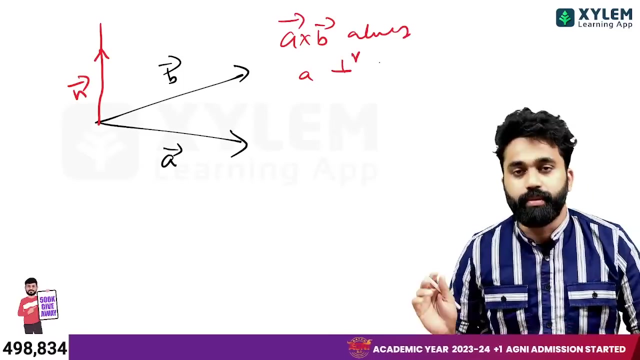 Children pay attention. There is one thing you need to pay attention to: If I take two vectors- cross product in Tamil- I get a unit, not a unit, a perpendicular vector. If I get a vector that is perpendicular to these two vectors, I always get a cross product. A cross B, always a perpendicular vector, Always a perpendicular vector. This is very important. This is an idea. 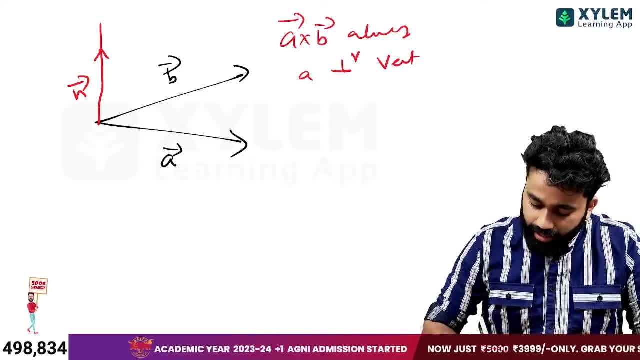 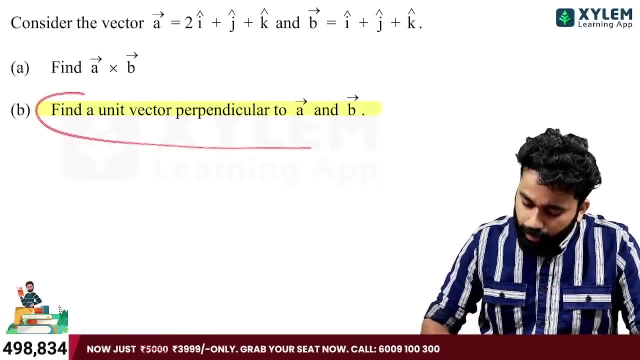 A cross B- always a perpendicular vector. Everyone gets a perpendicular vector for A and B. So if you get such a question, children pay attention. If you want to see a perpendicular vector for these two vectors, you need to do A cross B- always a perpendicular vector. 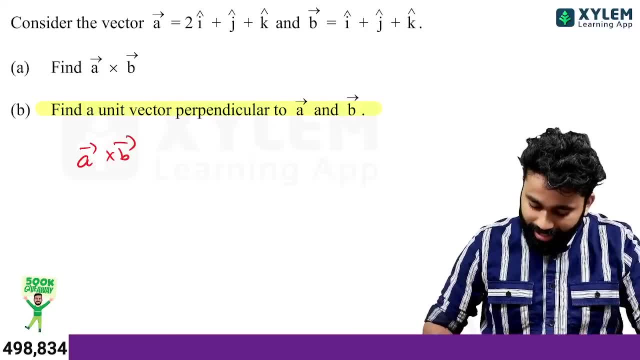 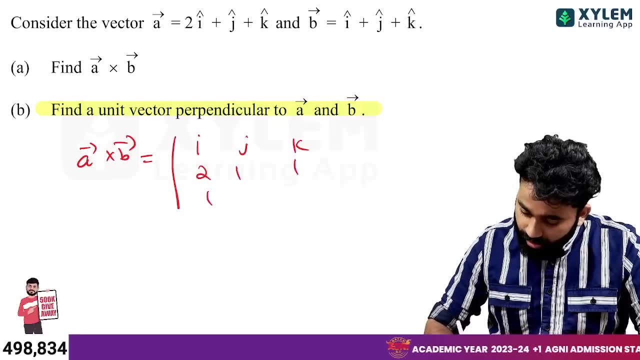 This is called a Javan vector. If you see A cross B, you know what IJK, IJK, As we did. now you do it alone: 2, 1, 1.. 1,, 1, 1.. 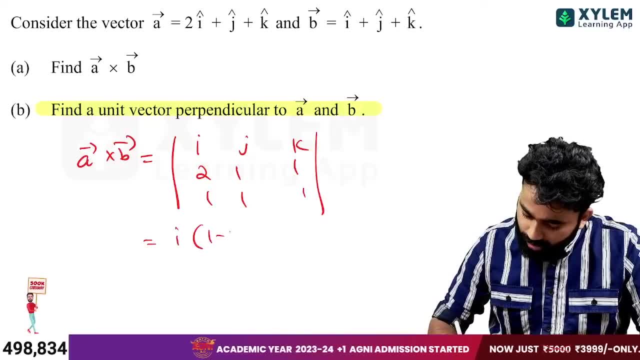 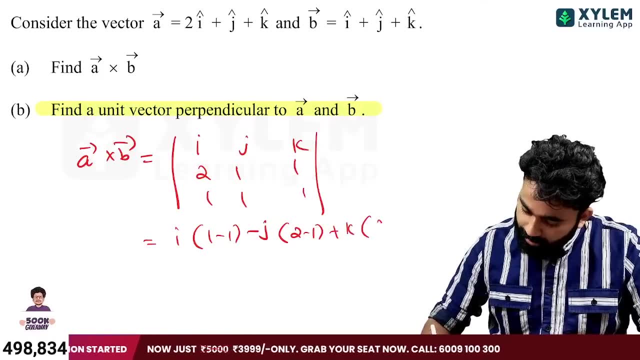 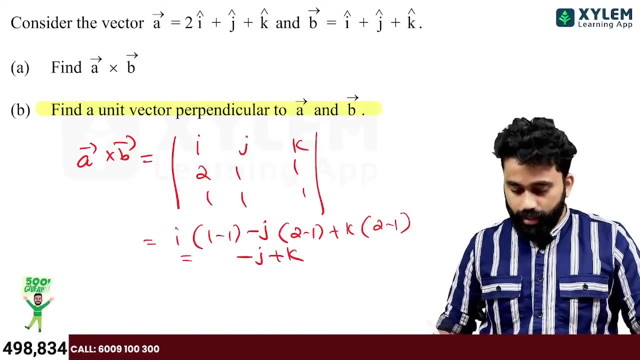 So you get I into 1 minus 1 minus J, into 2 minus 1 plus K, into 2 minus 1.. So you get minus J plus K. Okay, So the magnitude of this is Okay. So what is the magnitude of this? 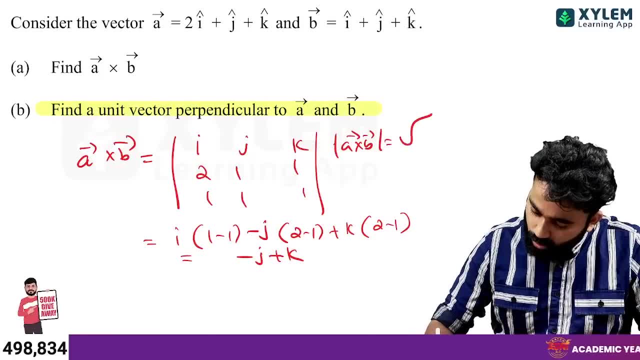 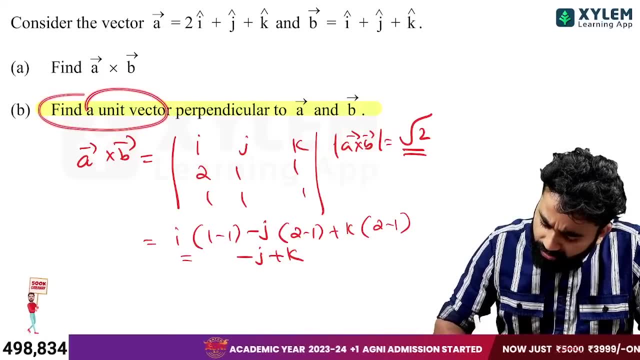 What is the magnitude of A cross B? That is equal to root 1 square plus 1 square, That is root 2.. Is that okay? You asked to find a unit vector perpendicular to A and B. So when you see A cross B, you get a vector. 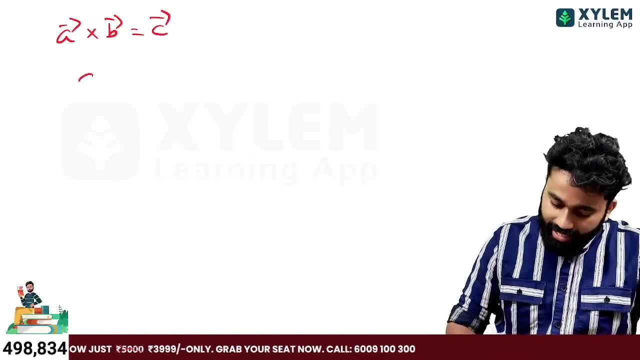 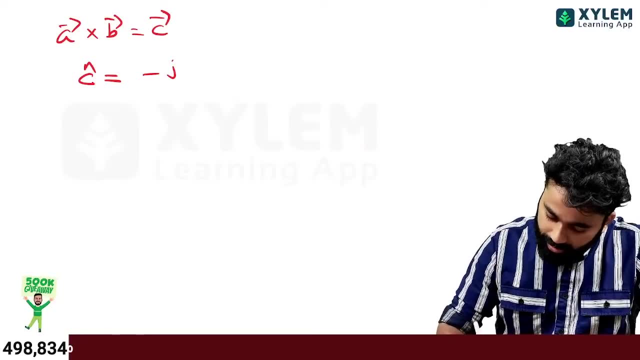 You get a new vector, That is C vector. But when you see its unit vector, what is the final answer? So what is C vector? Minus J plus K. Minus J plus K divided by root 1.. Minus J plus K divided by root 2.. 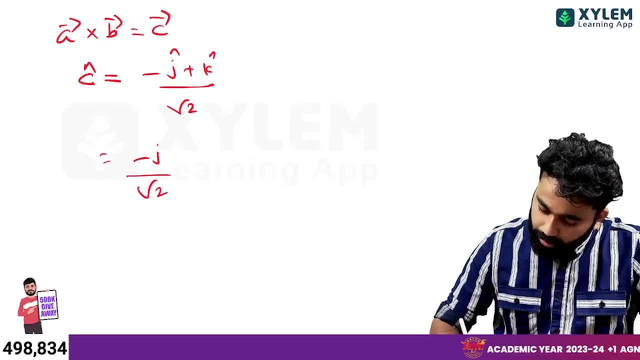 So the final answer is- And this question has to be asked in your exam- This is important. There is more than one chance to ask this. This is very important. You have to teach your children. You have to learn it 100%. 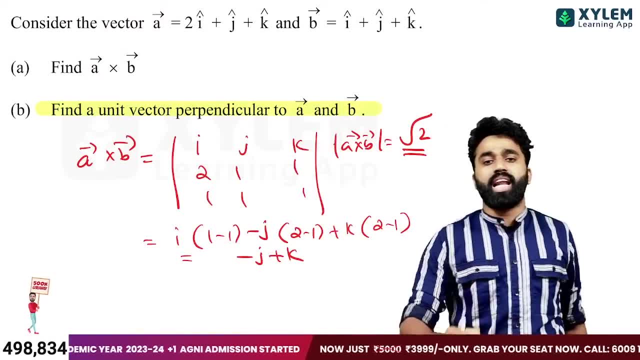 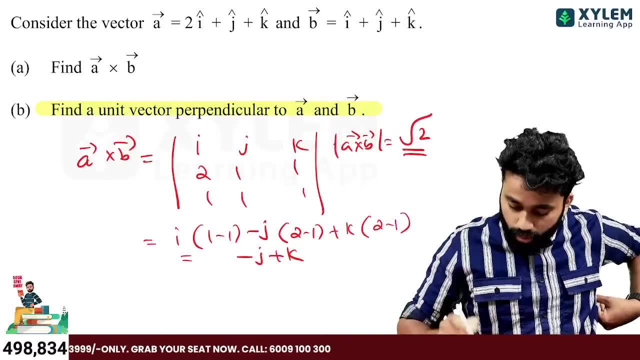 You have to learn it 100%, children. You have to learn it 100%. This method, or this question, is very important. You have to use only this much idea. Do you know what that idea is, Children? yes, That is its idea. 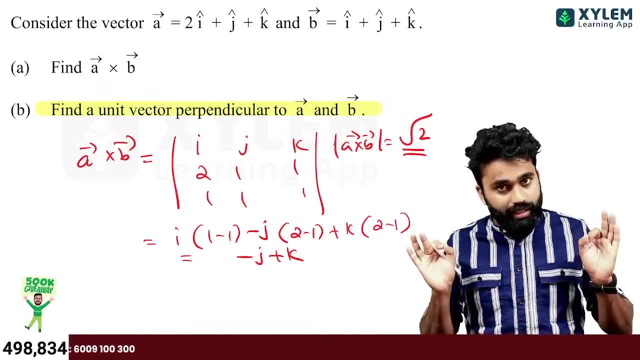 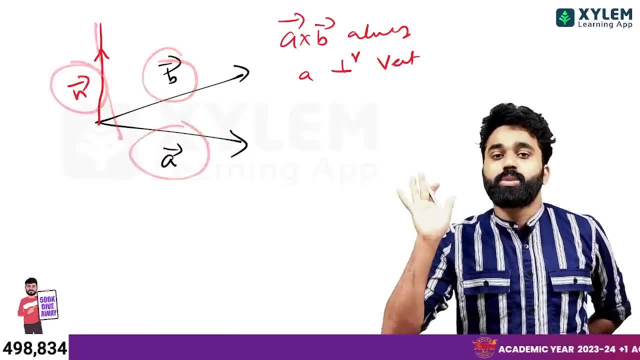 Find a unit vector perpendicular to A and B. If you need to find a unit vector perpendicular to A and B, you have to find it. This is just one. you have to find the cross product of it, So you will get a new vector. 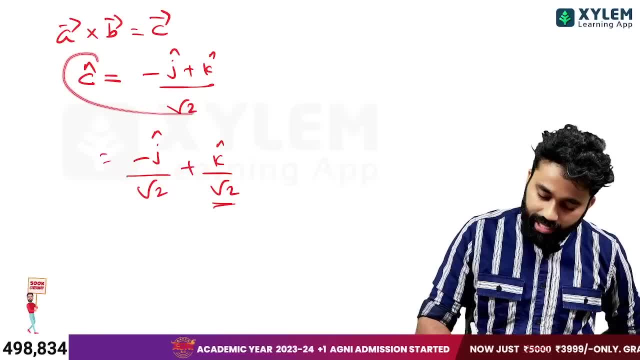 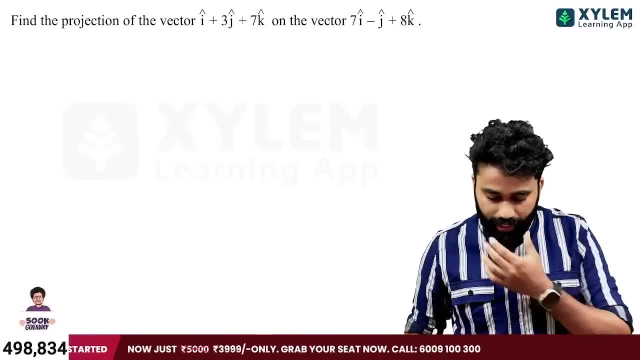 It will be perpendicular to this and this. Then, how to find the new vector, Find the union vector. This is very important to all the people in mind who have put fire emoji- Very important. The next topic is called projection. Which one should I say Projection? 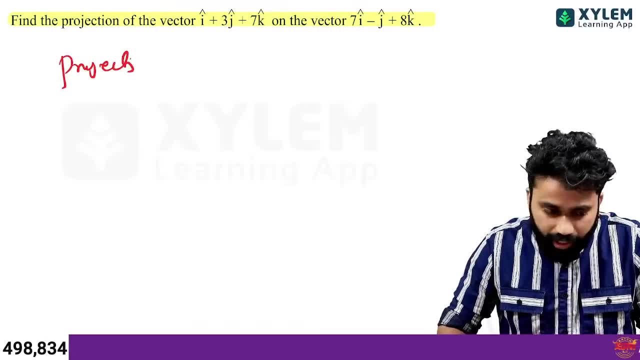 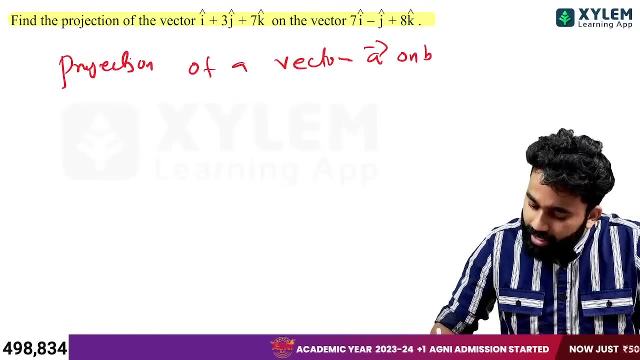 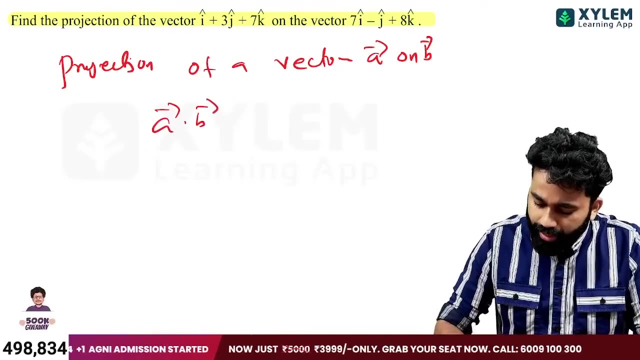 Children. projection of a vector. I am looking at this method. Projection of a vector A on B. Projection of a vector A on B. That is all A dot B divided by Isn't A on B, It is B at the bottom. 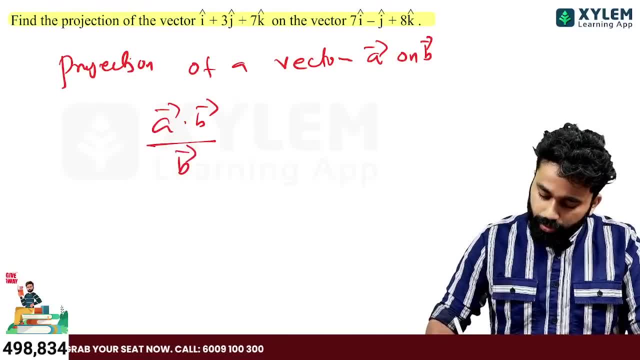 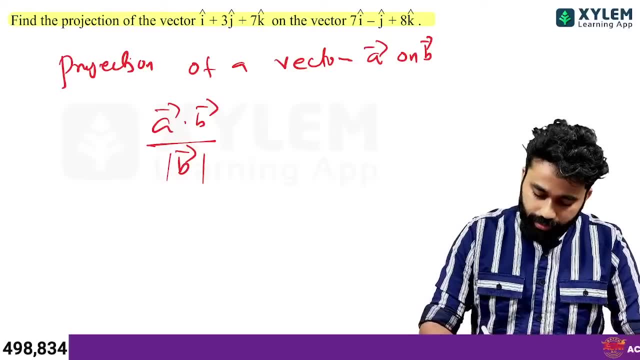 If it is B on A, it is A at the bottom. That is the difference Projection of a vector A on B. Take two dots and take the magnitude at the bottom. So the answer is very simple: A dot B. children pay attention. 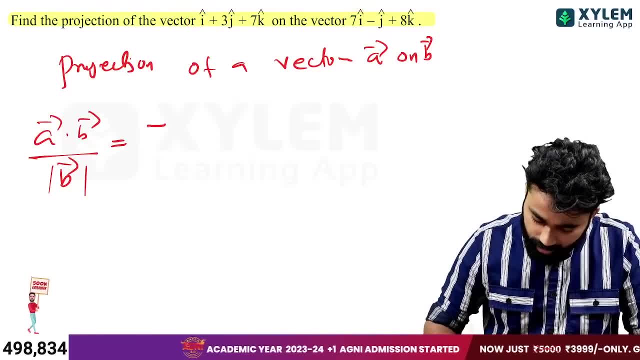 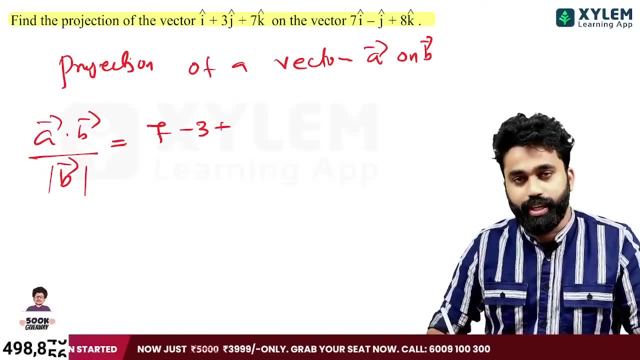 1 into 7. I into this and I into that. 1 into 7.. 7. Plus 3 into minus 1. That is minus 3.. Plus 7 into 8.. 8 times 8 is 64.. 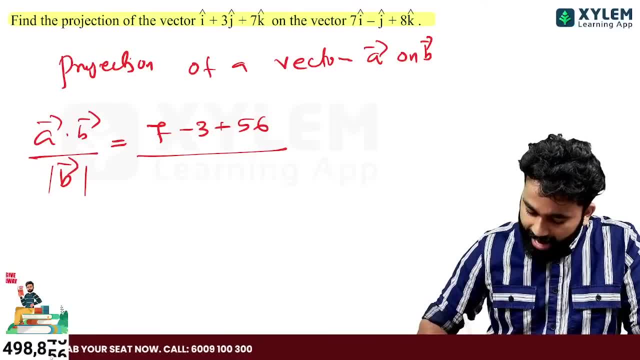 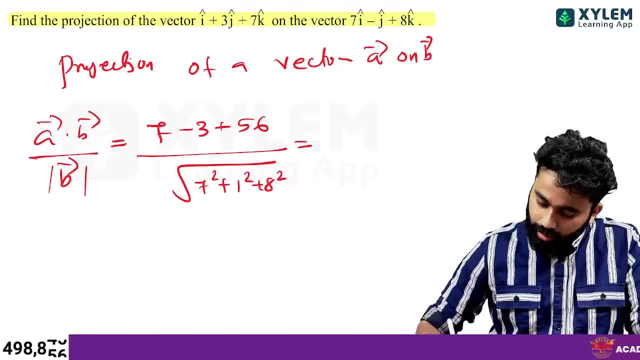 64 times 8 is 56.. Divided by the magnitude of B: The magnitude of B. So the answer is very simple: 3 times 3 is 4.. 56 times 4 is 60.. Divided by 64.. 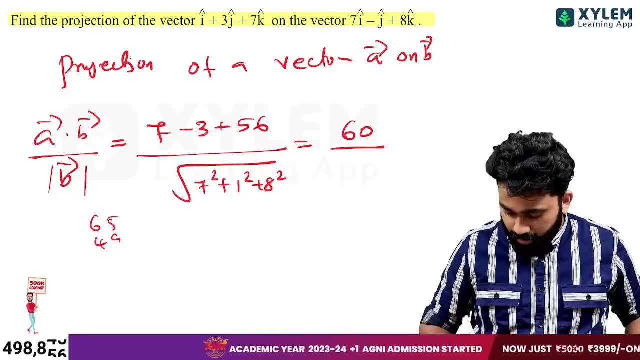 64 times 4 is 65.. 65 times 4 is 49.. 65 times 4 is 49.. 4 times 4 is 10.. 10 times 4 is 114.. This is the final answer. 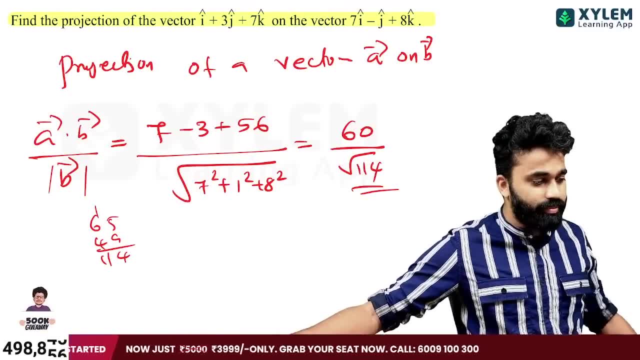 It is a set. It is a set. It is a set. I am going to cheat. I am not going to cheat, son, I am going to cheat. I have asked all of you, Ask your parents If they get married. I will. 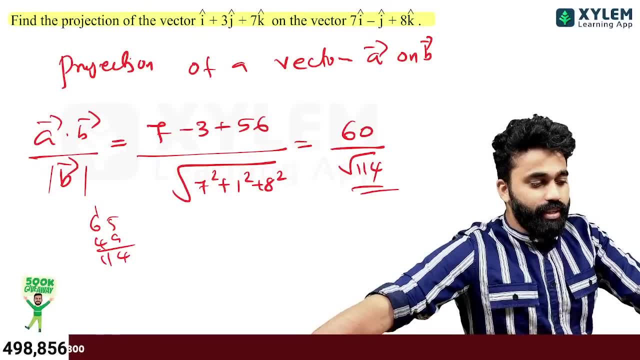 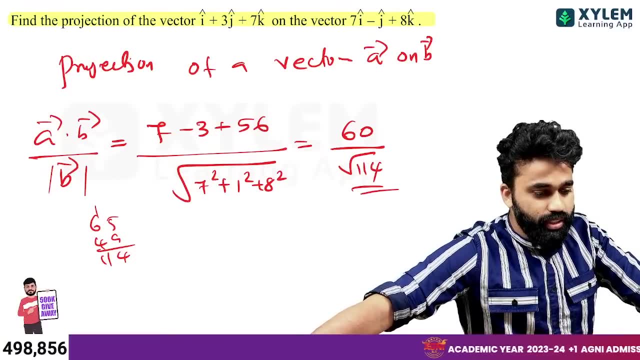 My son. If not, ask them. If you have good cheats to sell, tell me There are people to buy. Will you leave all the questions in Sir's mind? All the questions in Sir's mind, All the questions in Sir's mind. 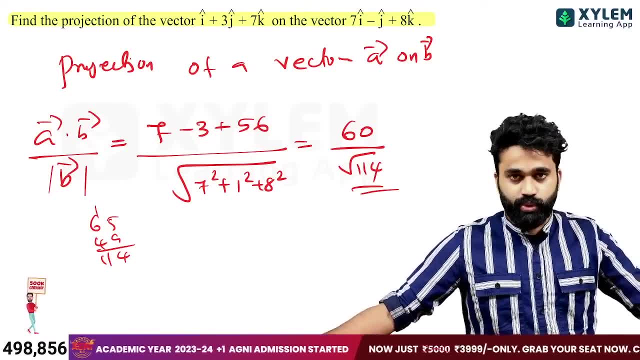 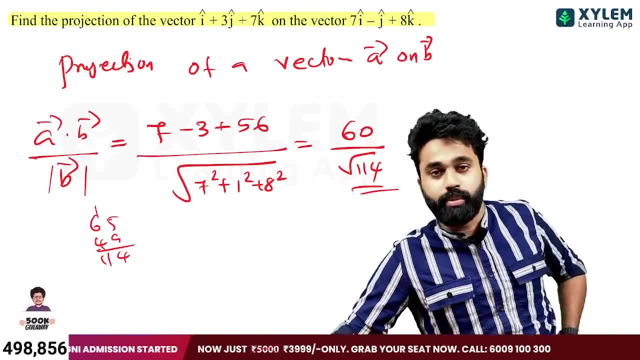 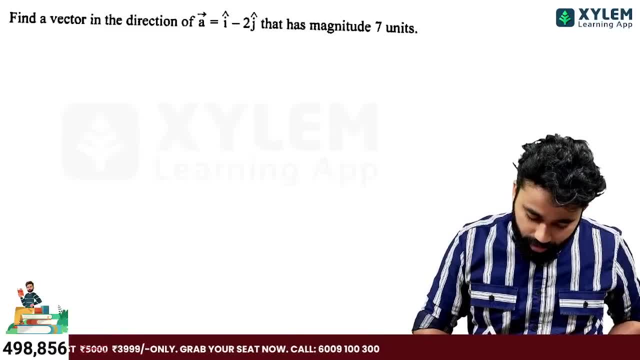 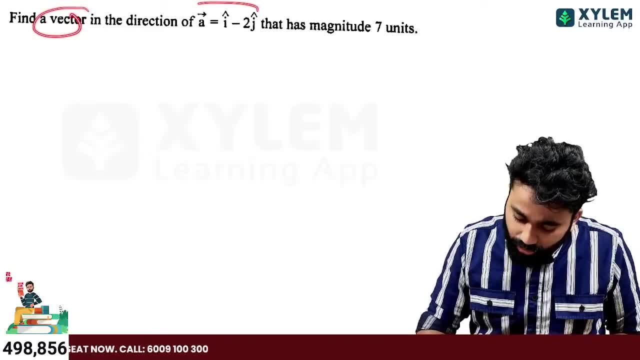 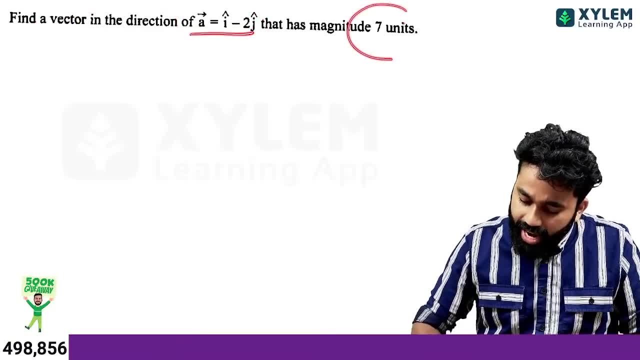 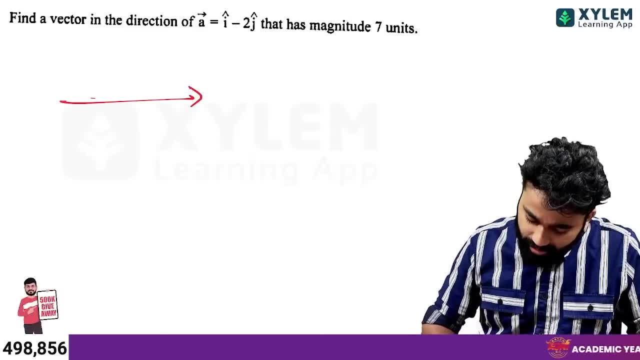 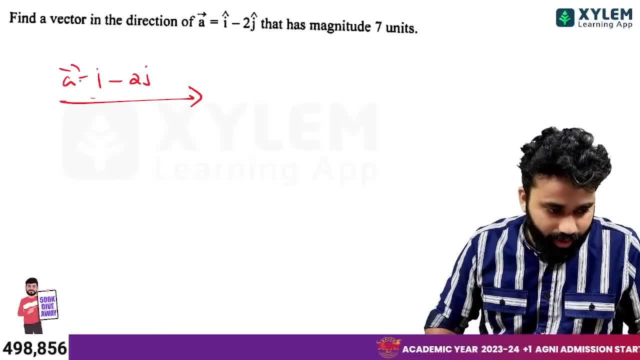 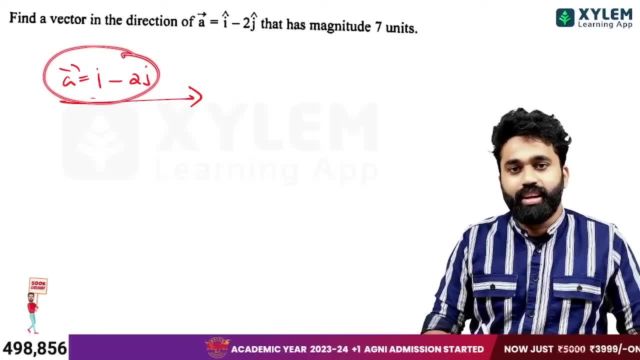 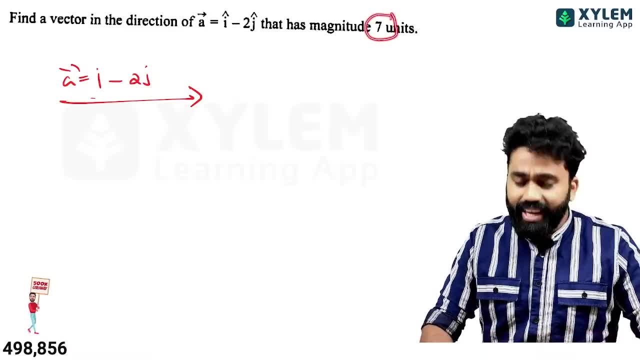 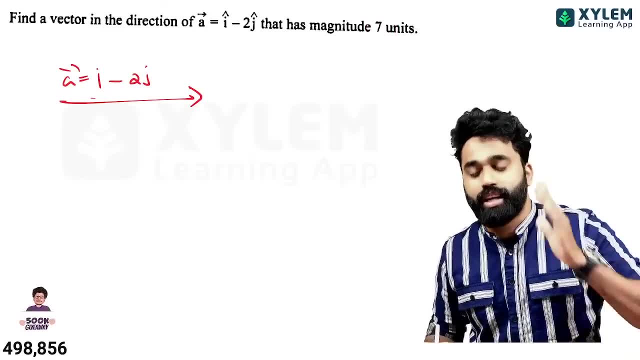 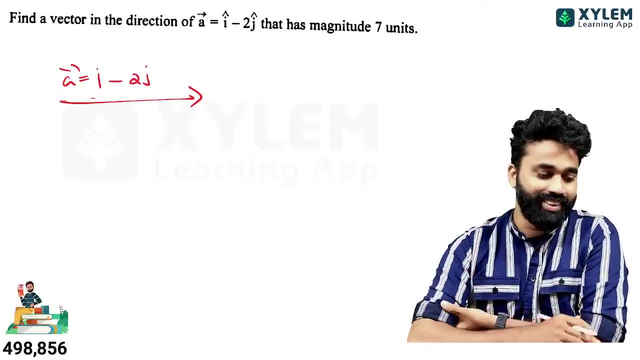 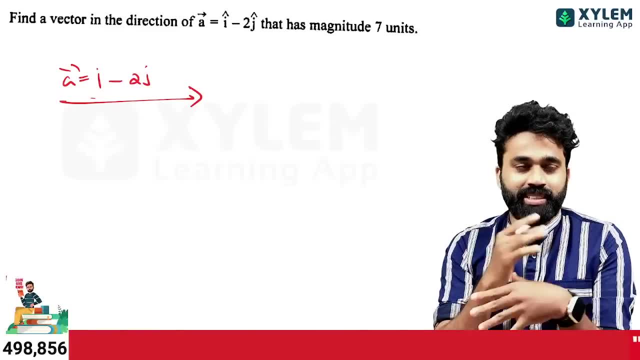 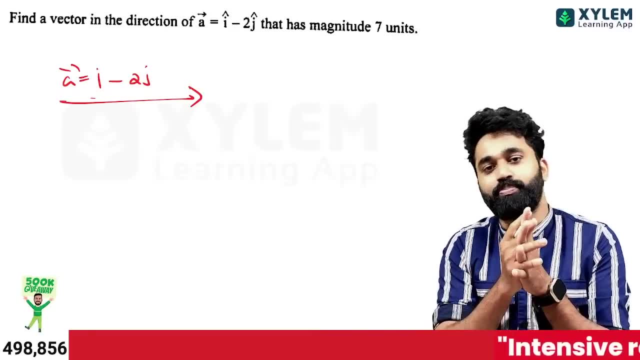 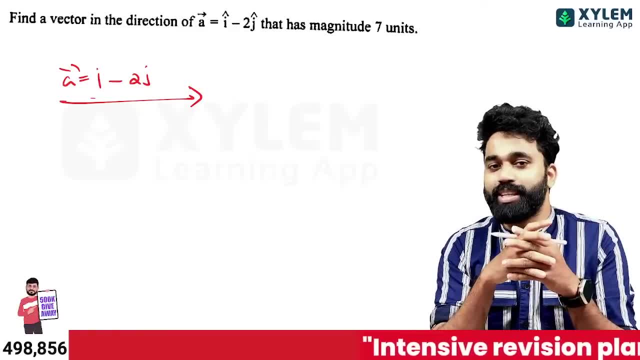 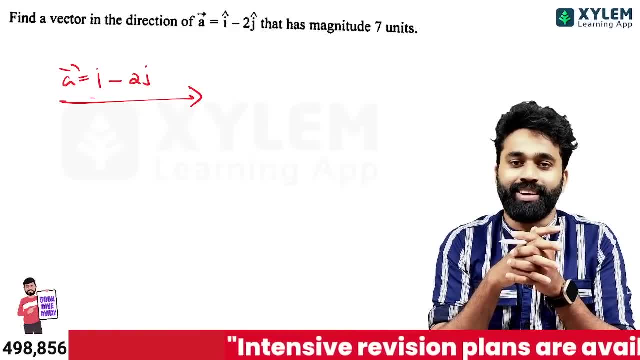 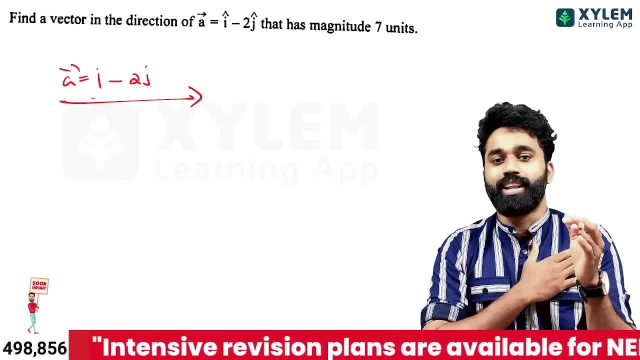 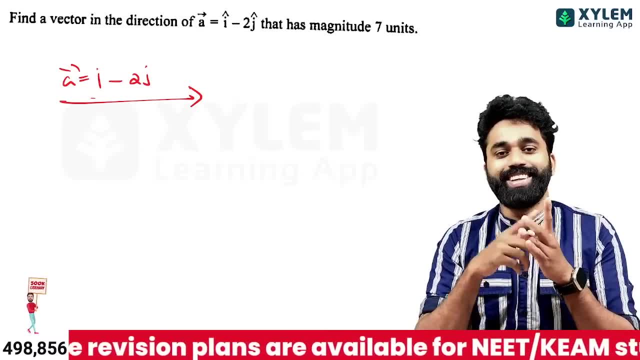 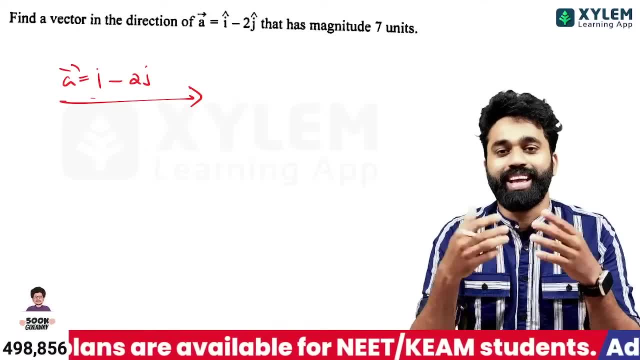 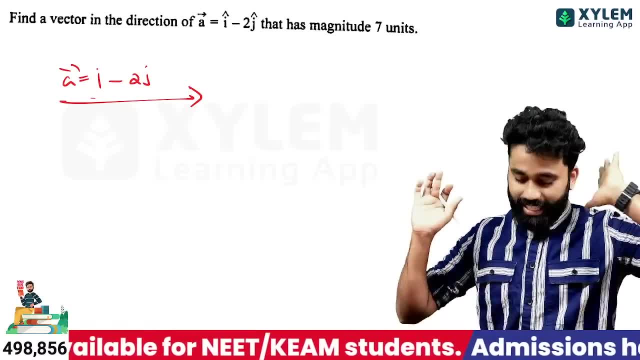 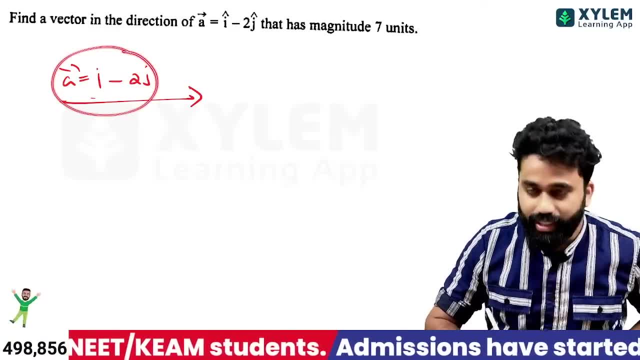 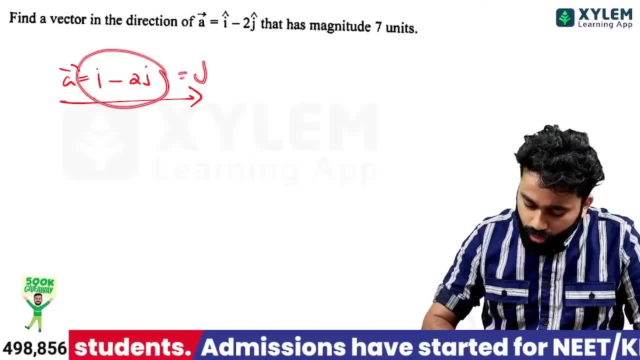 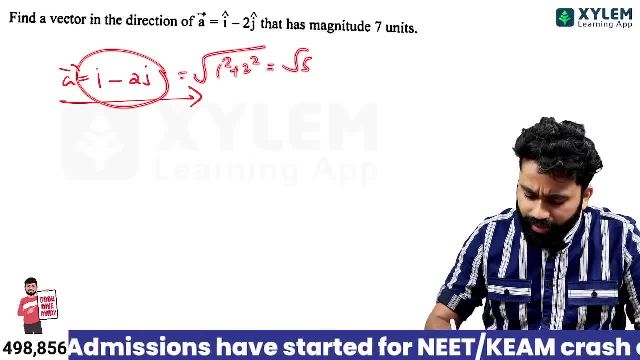 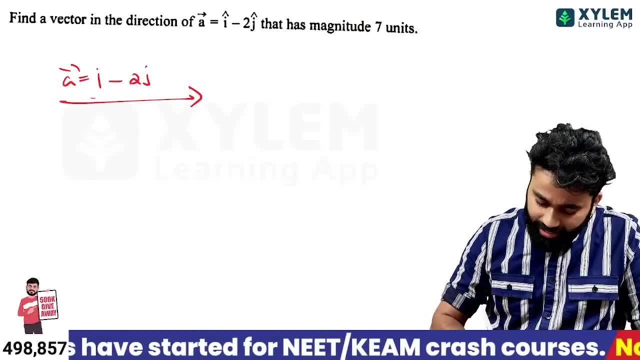 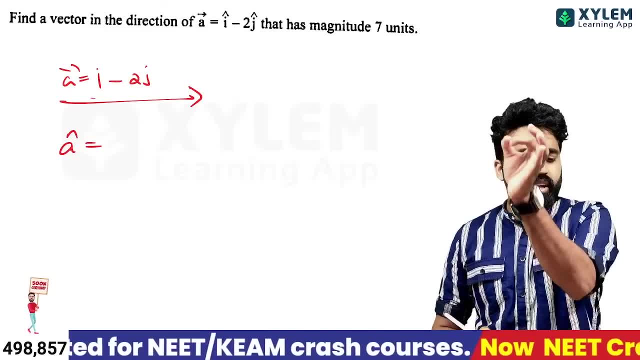 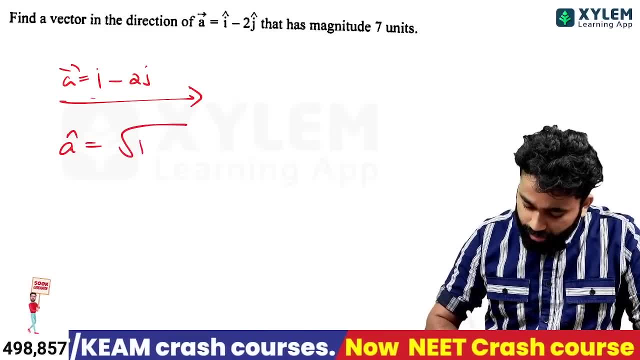 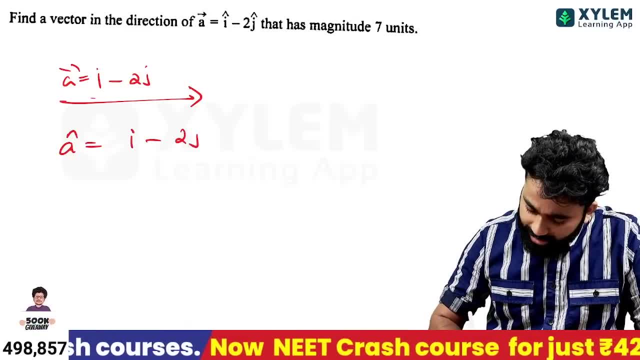 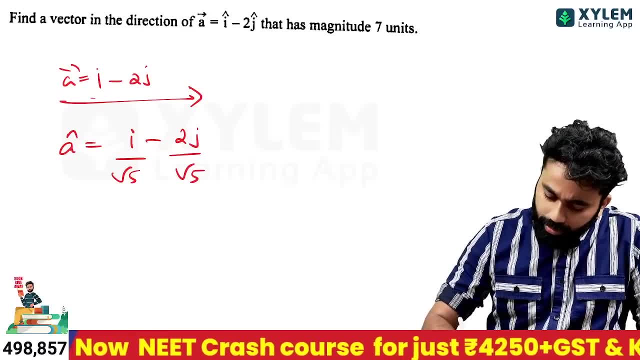 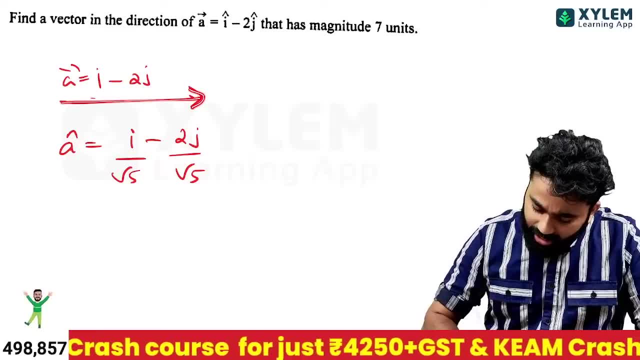 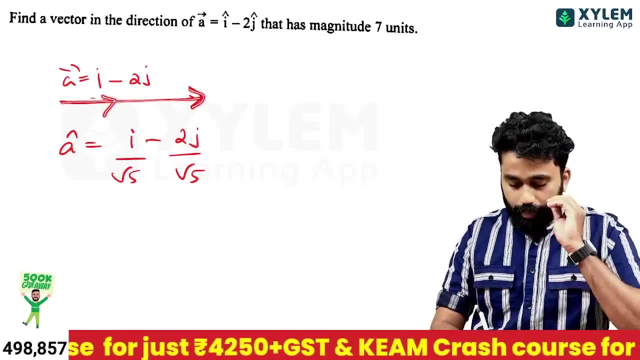 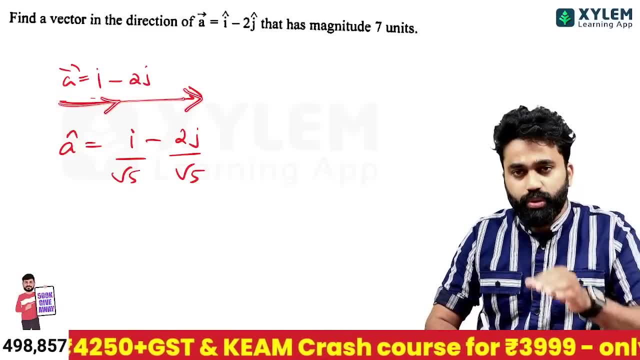 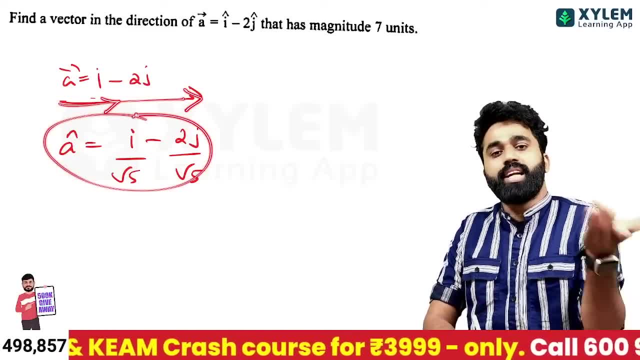 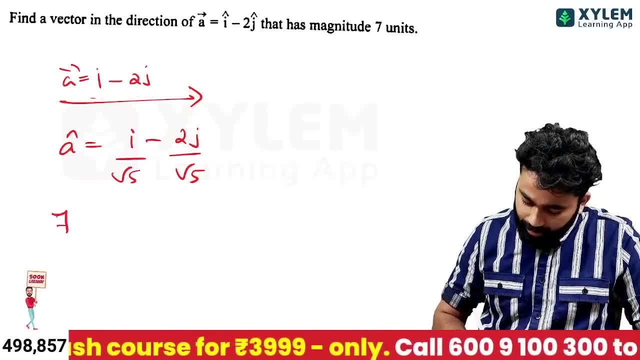 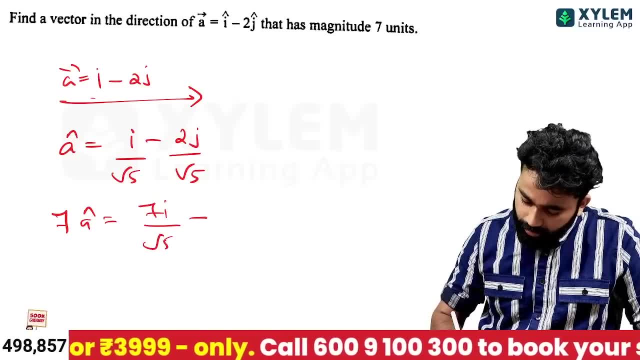 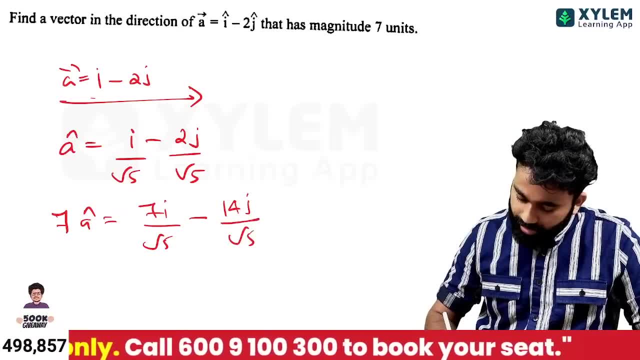 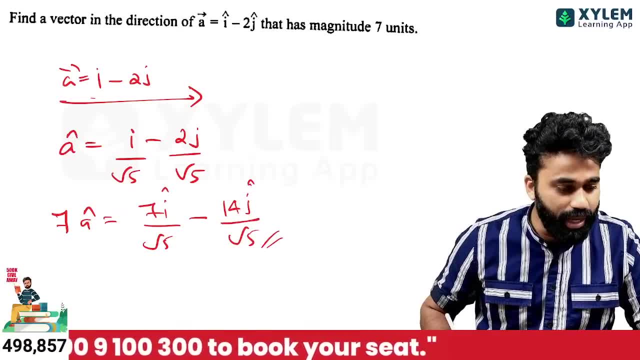 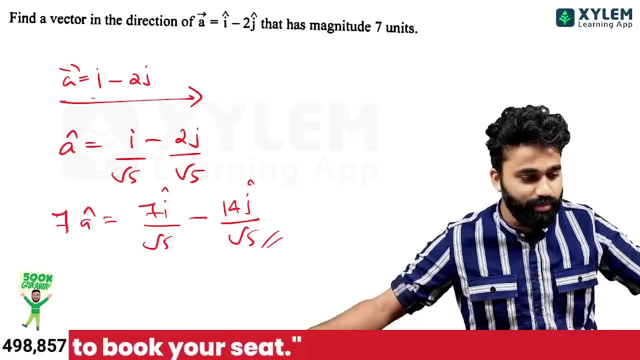 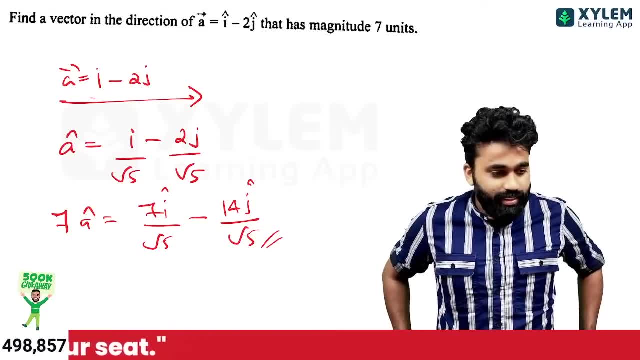 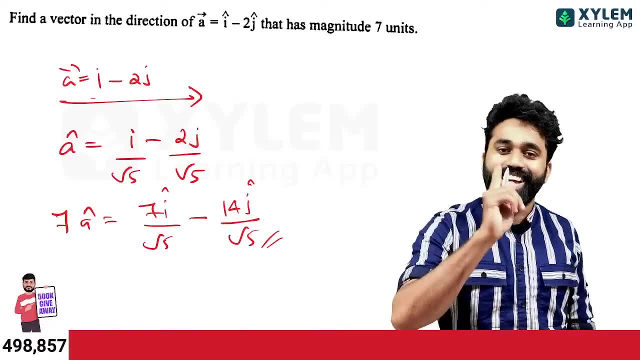 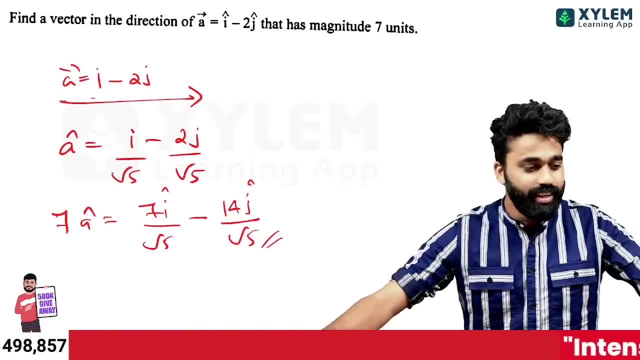 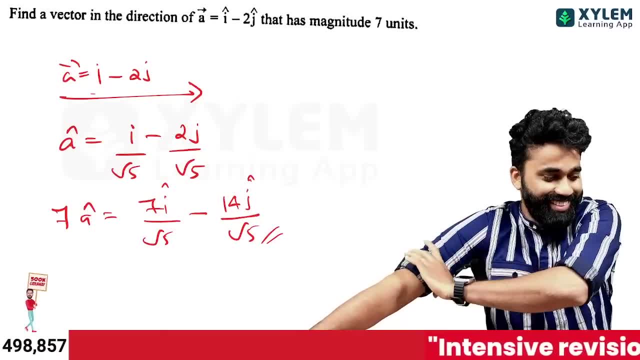 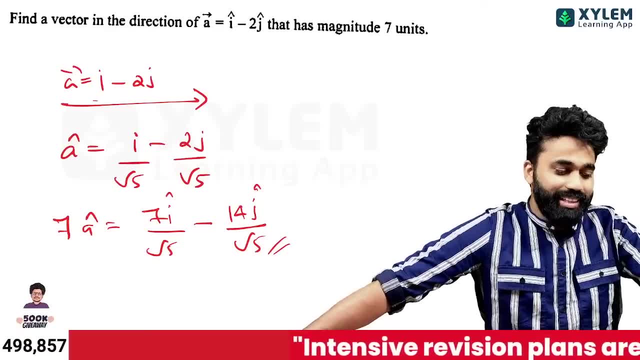 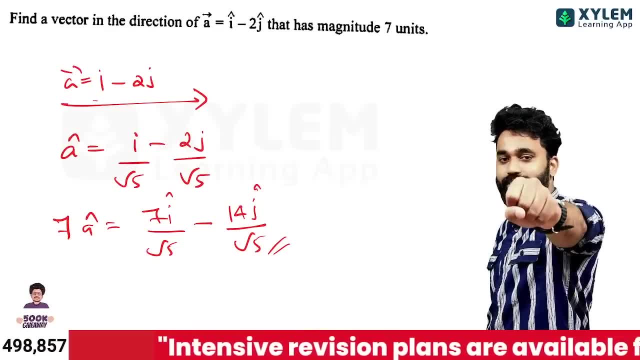 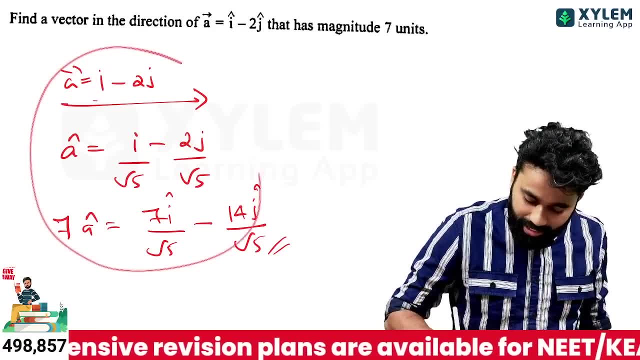 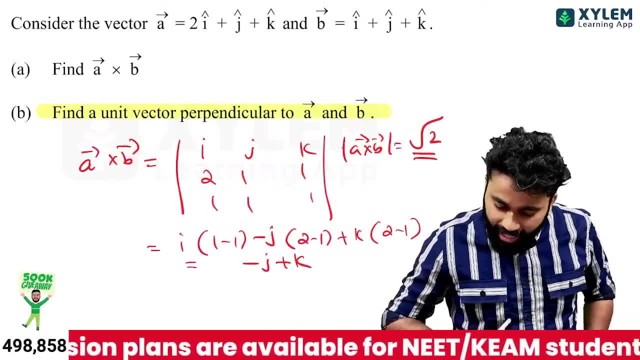 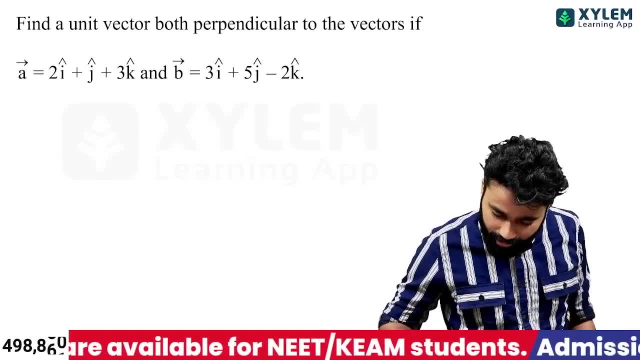 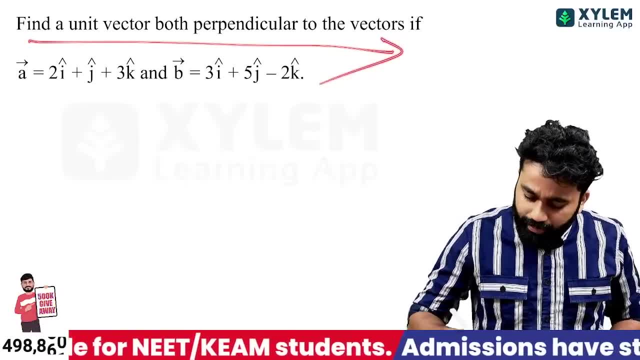 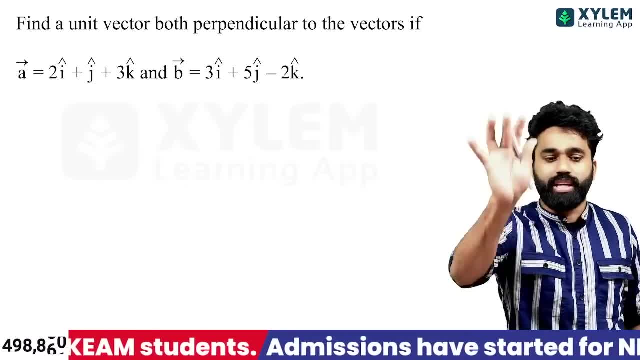 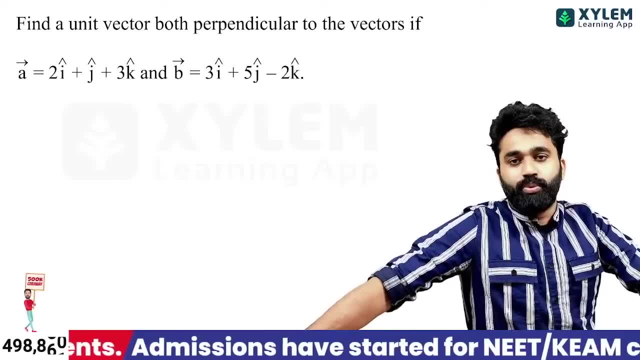 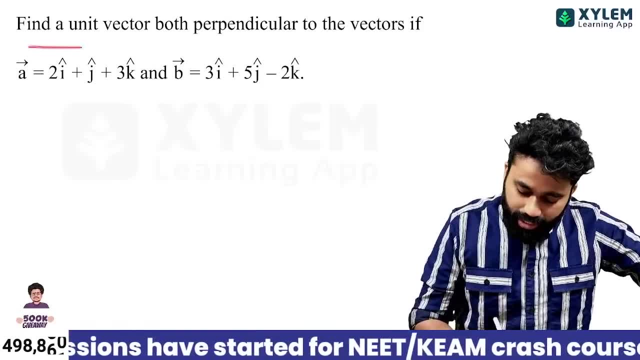 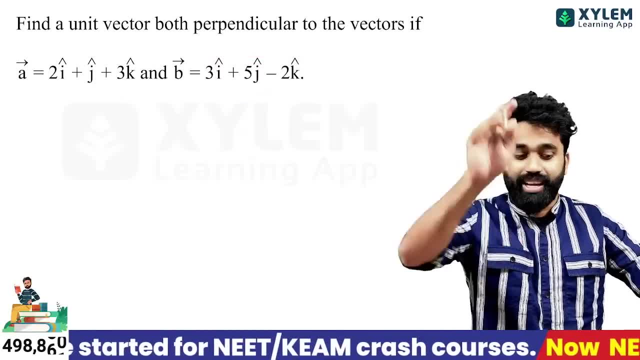 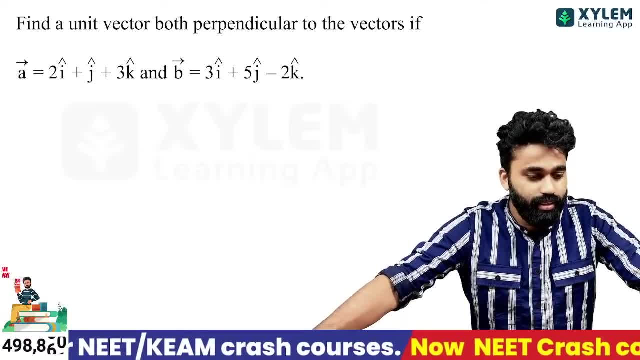 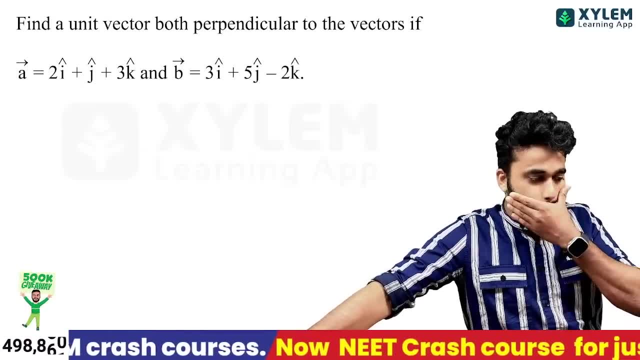 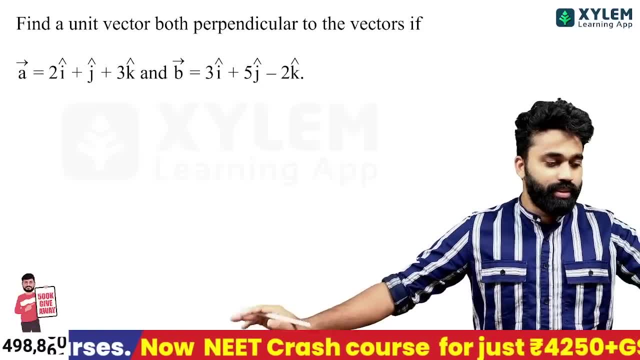 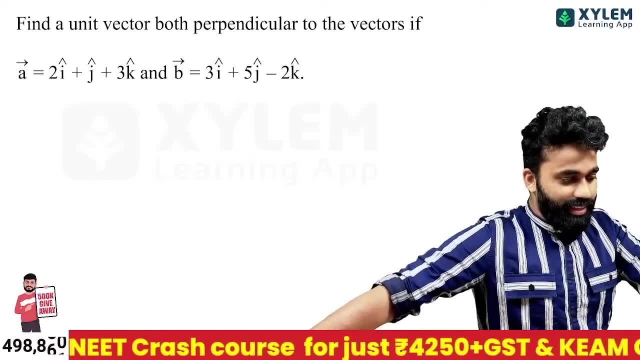 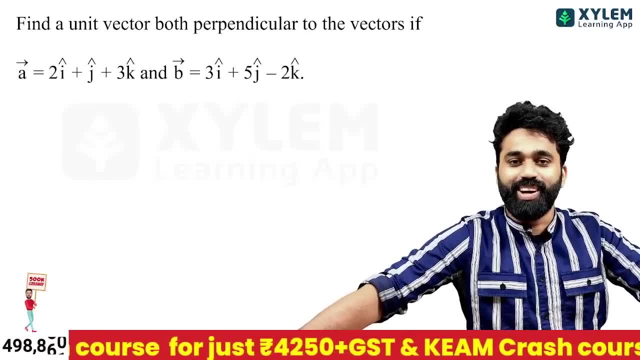 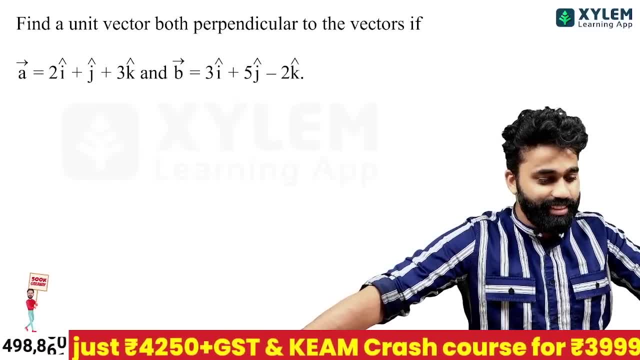 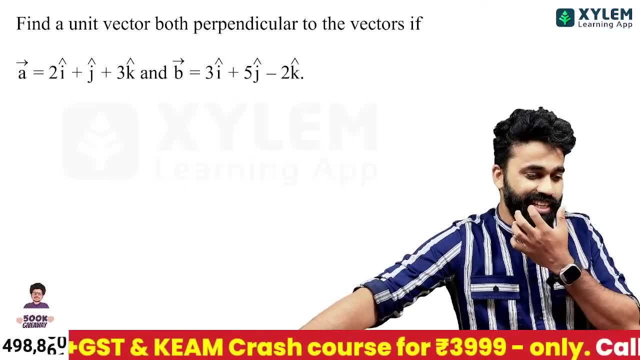 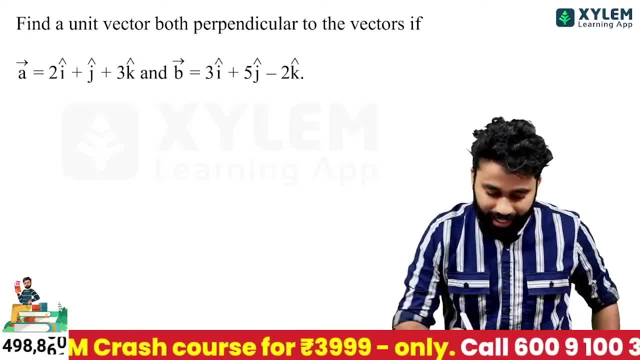 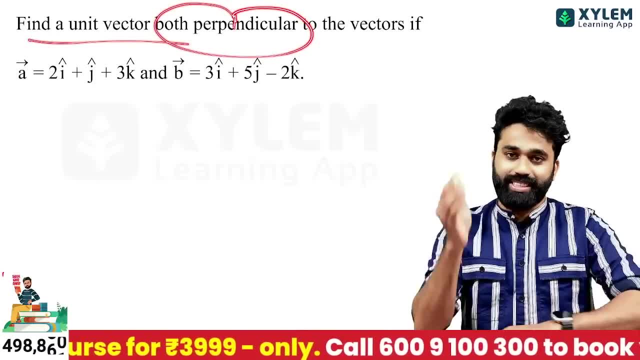 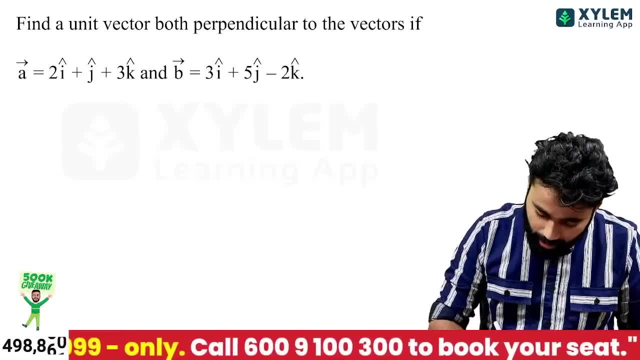 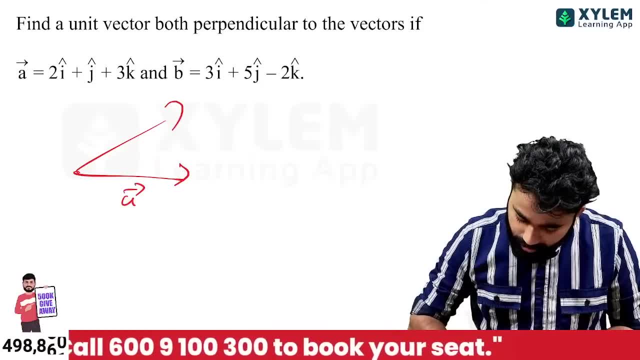 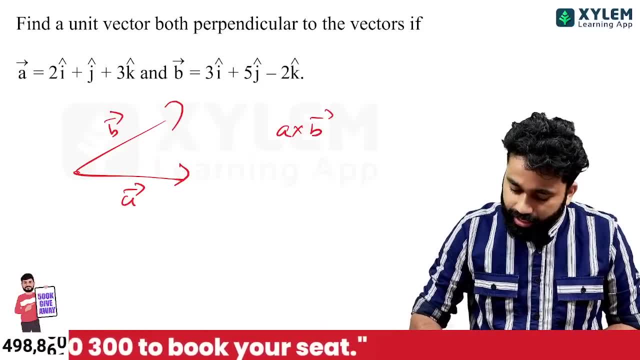 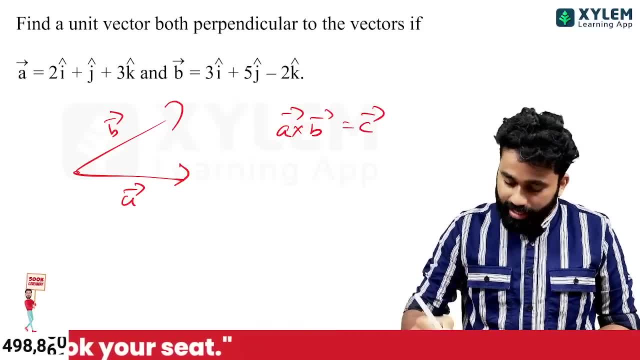 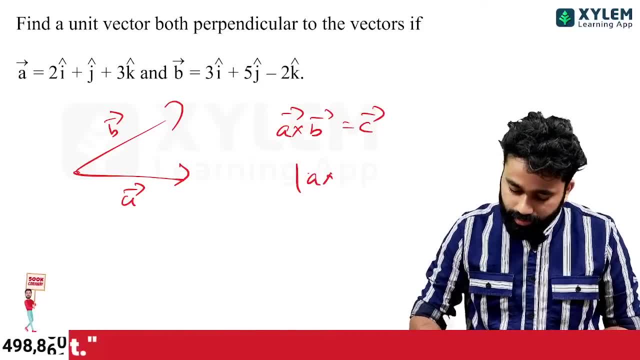 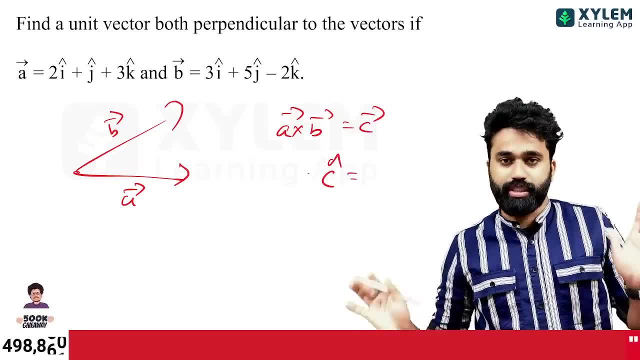 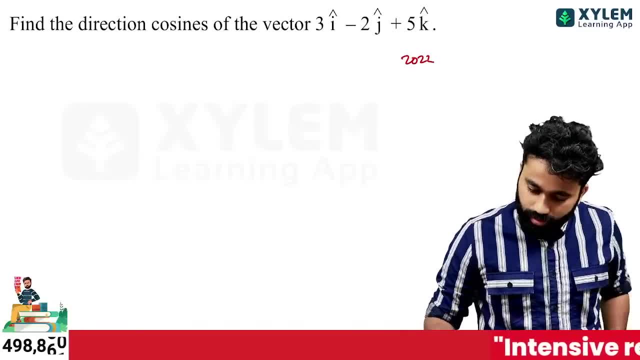 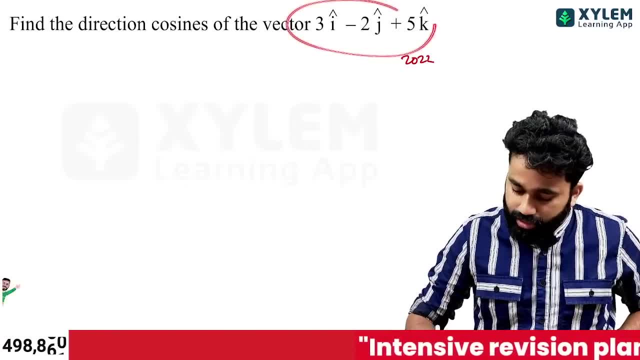 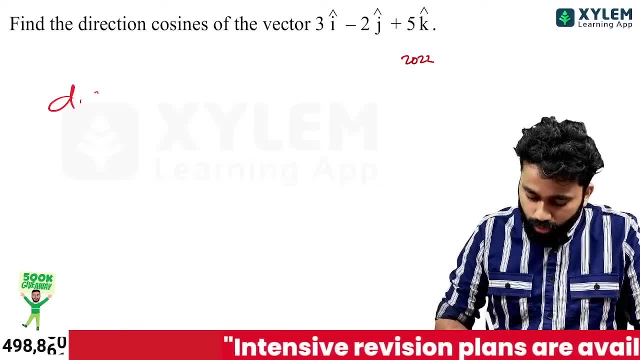 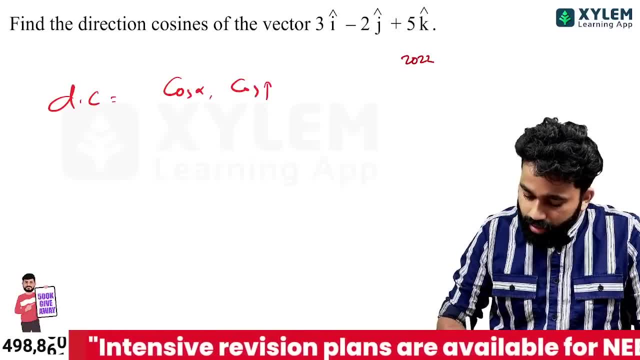 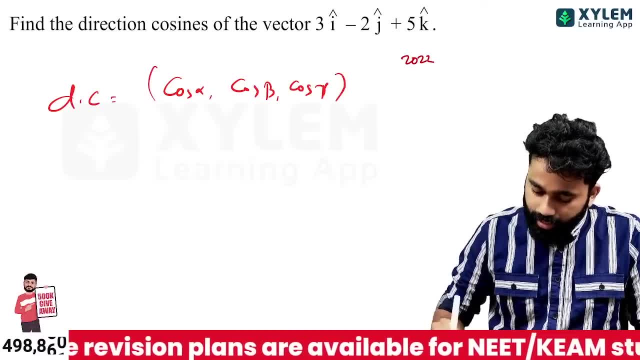 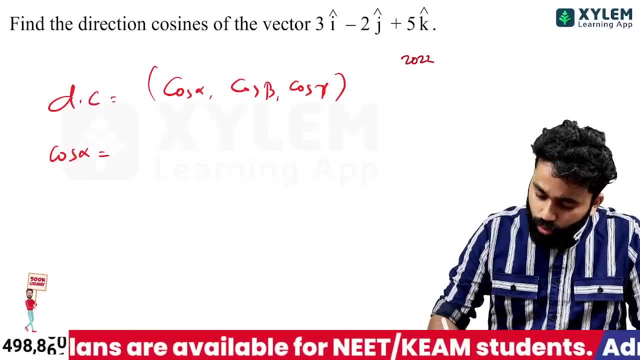 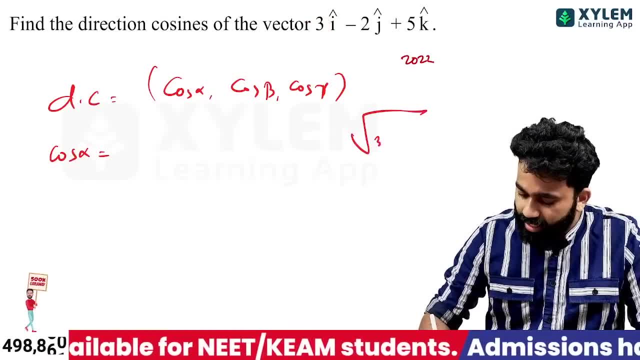 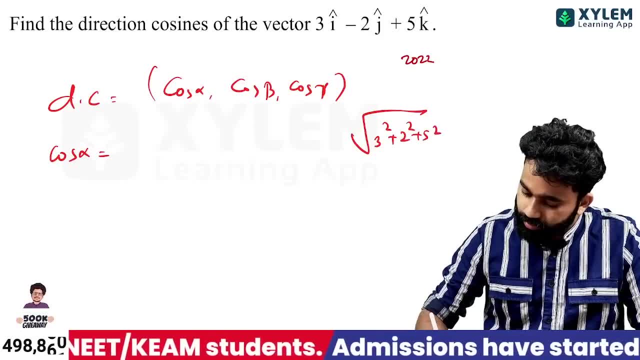 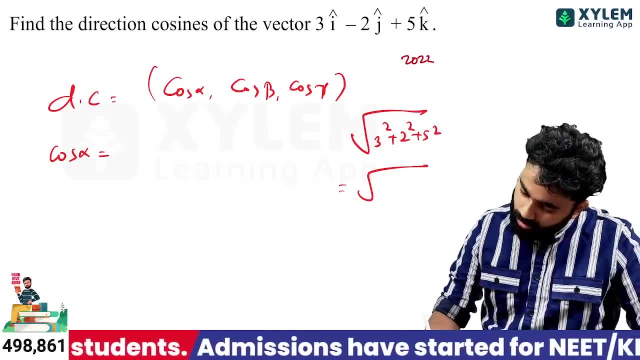 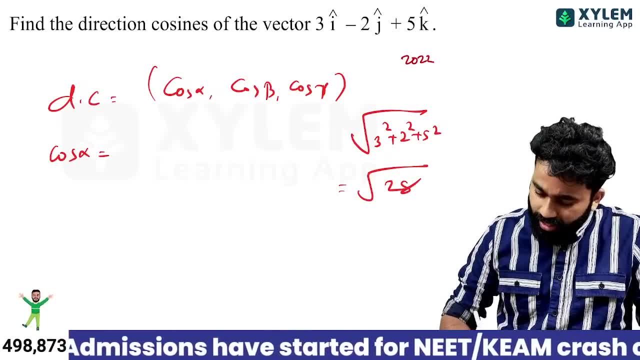 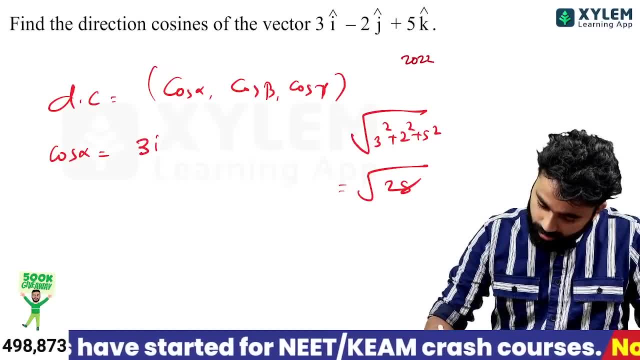 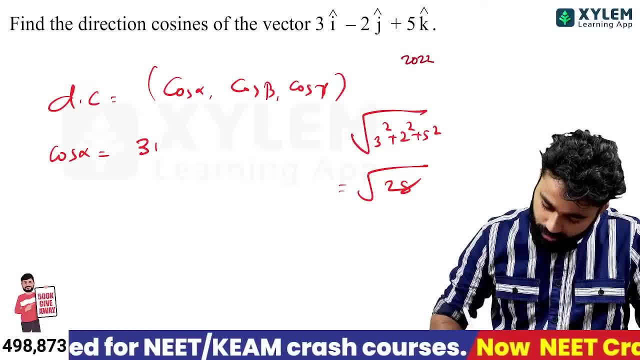 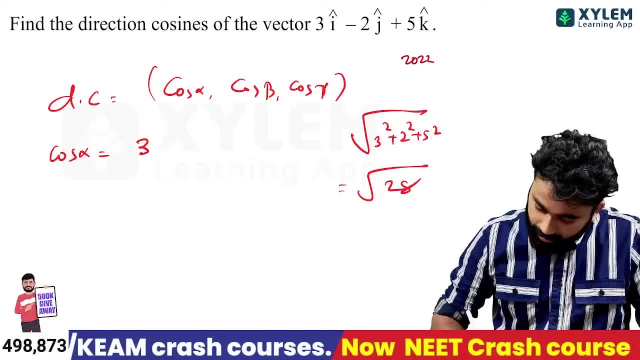 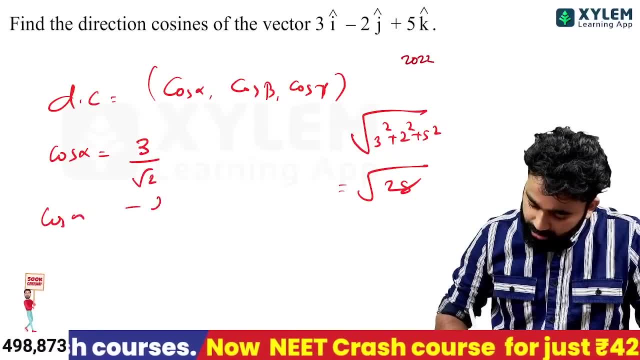 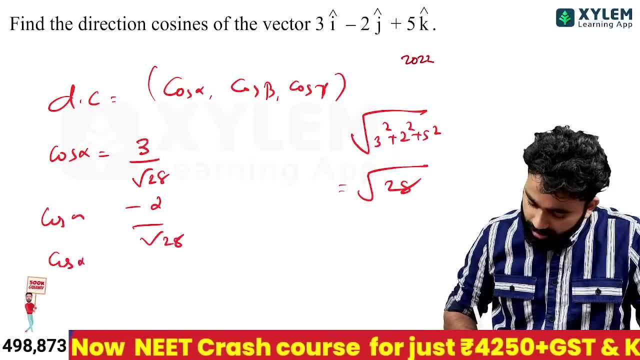 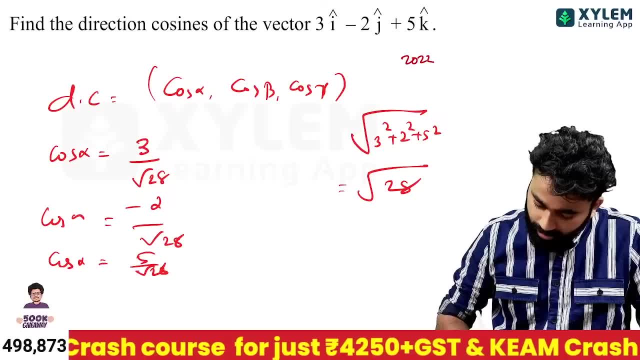 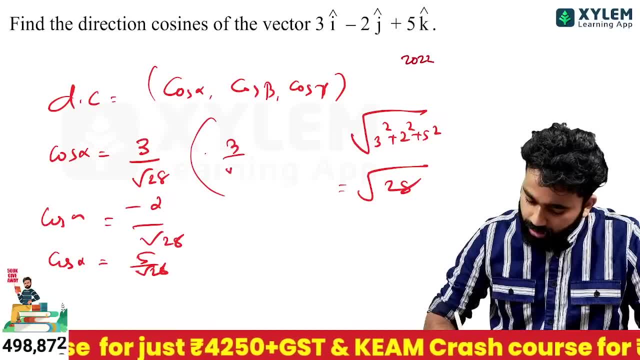 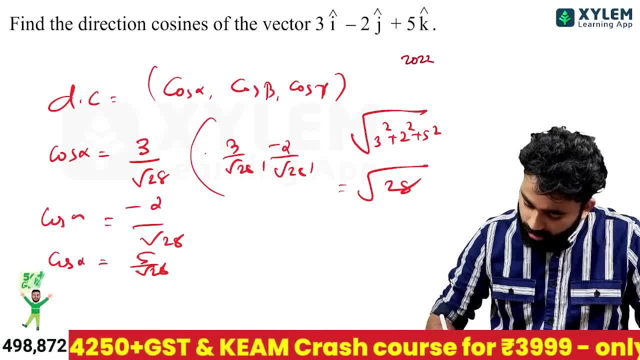 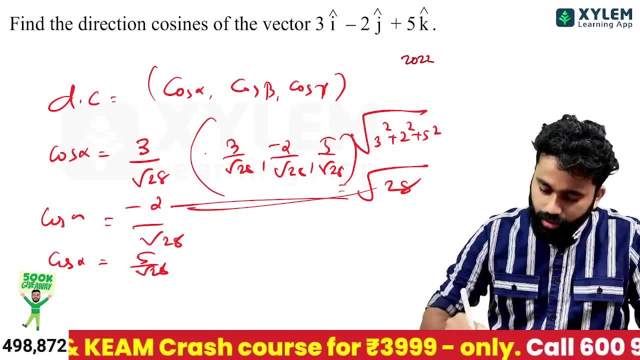 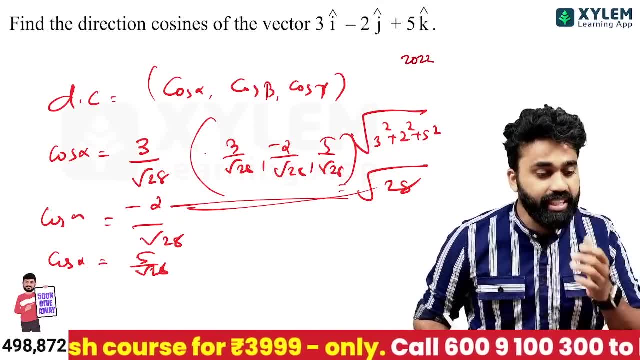 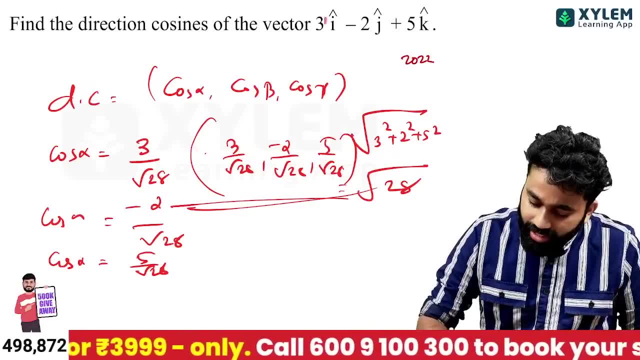 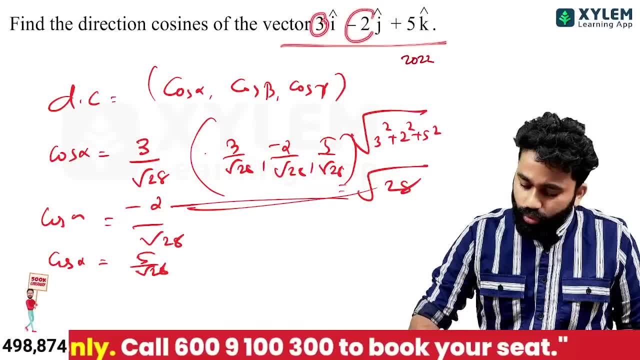 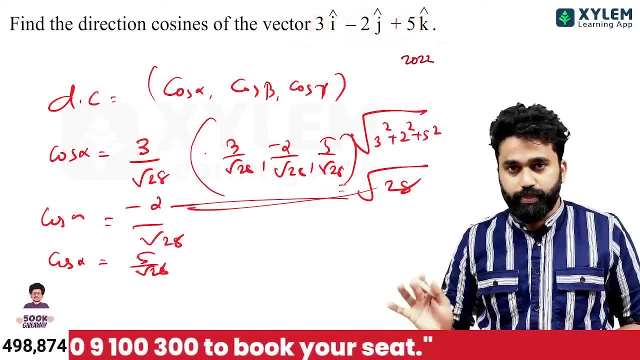 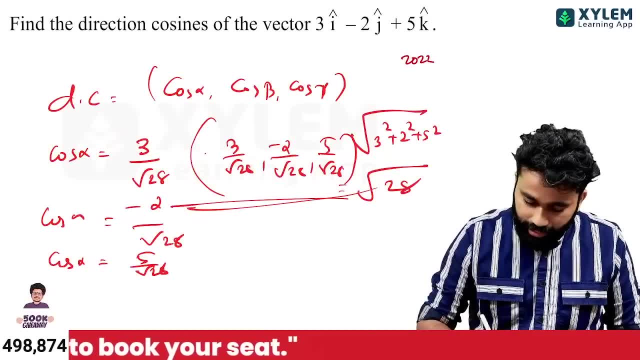 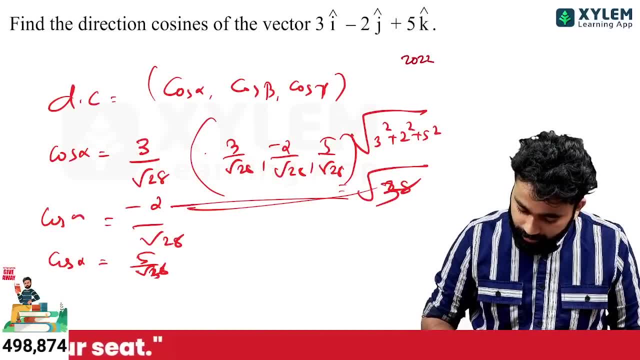 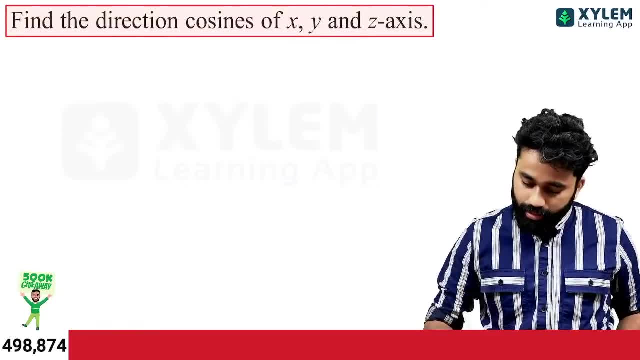 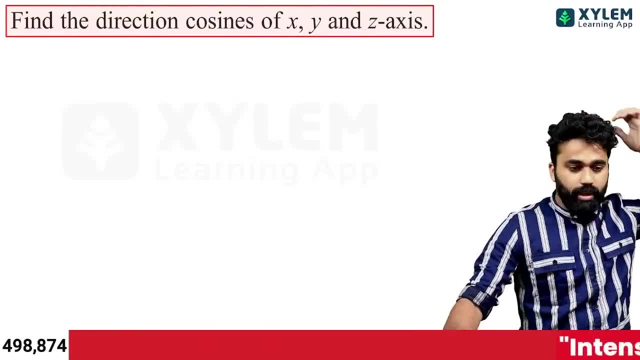 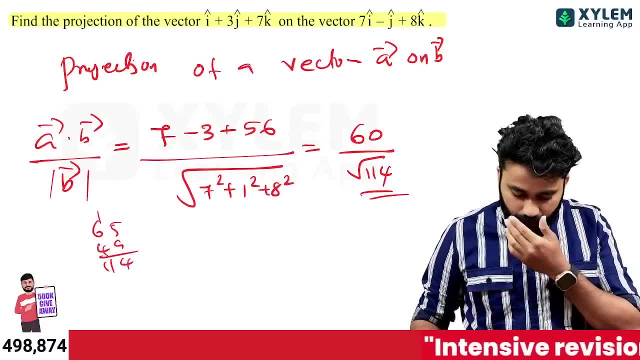 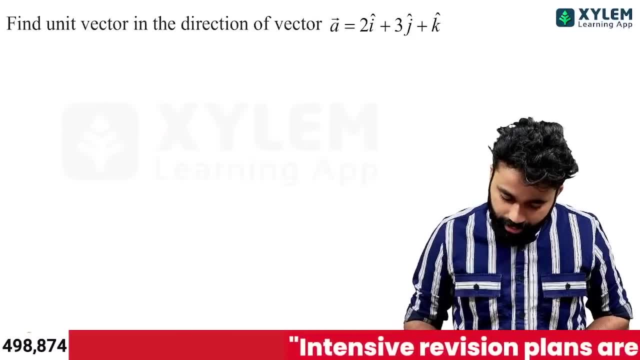 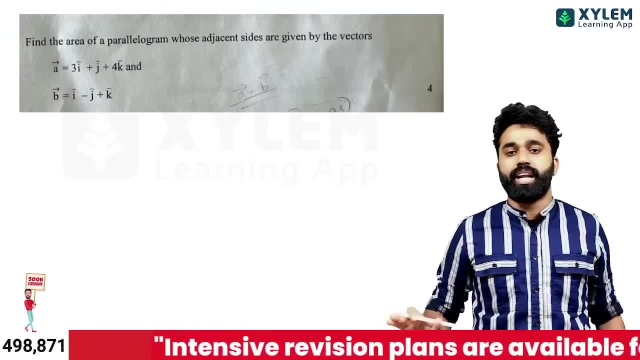 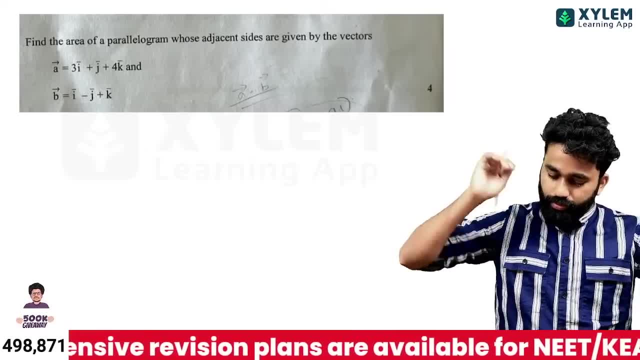 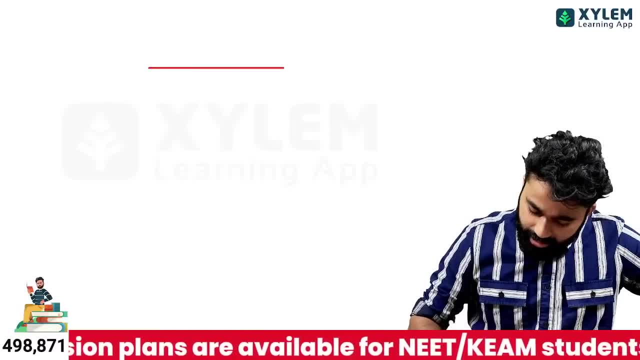 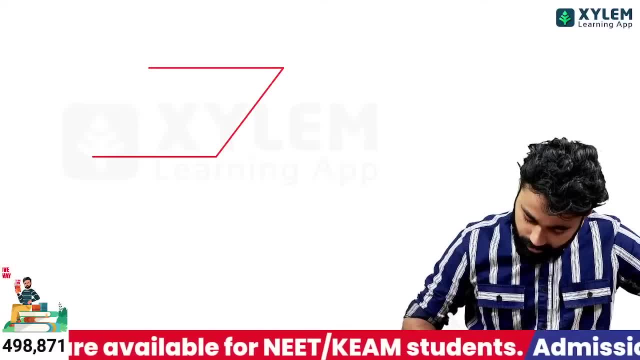 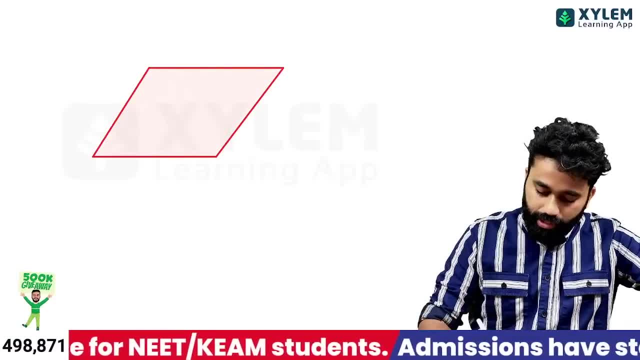 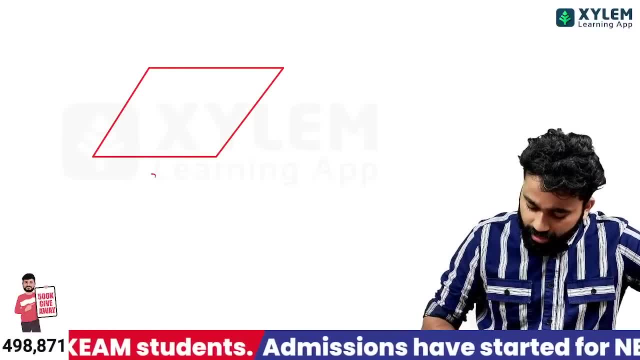 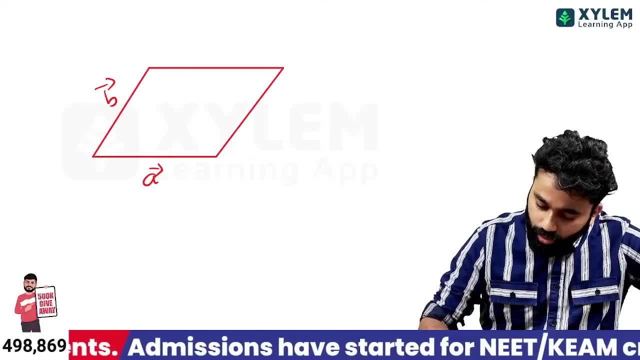 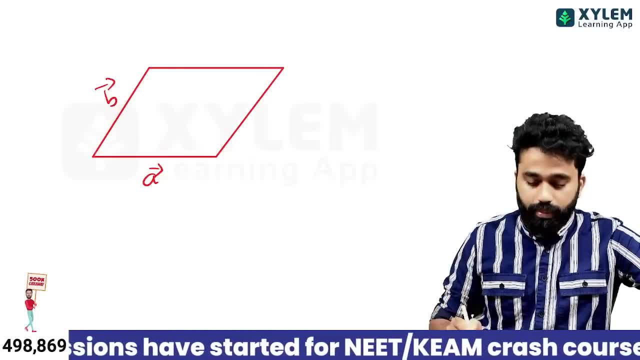 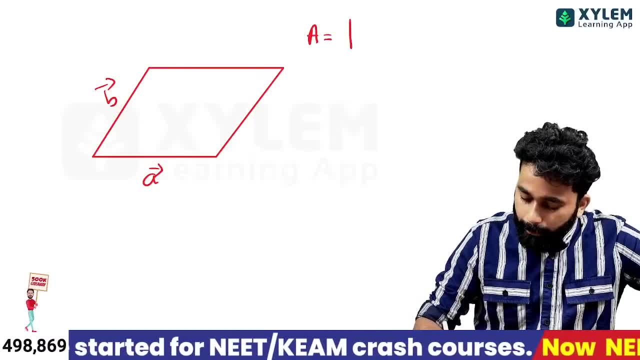 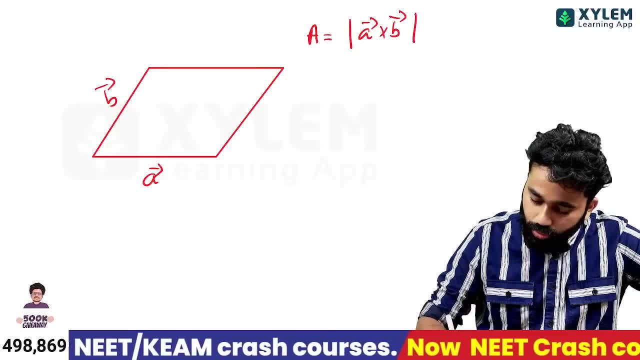 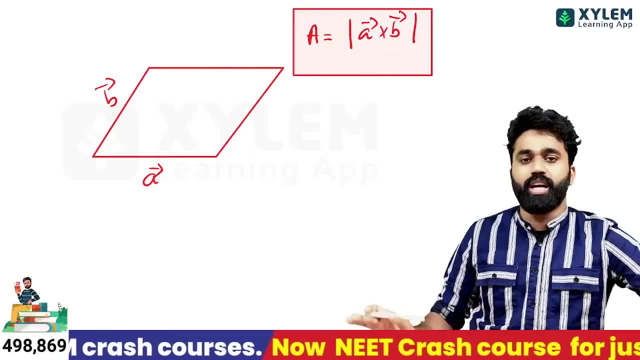 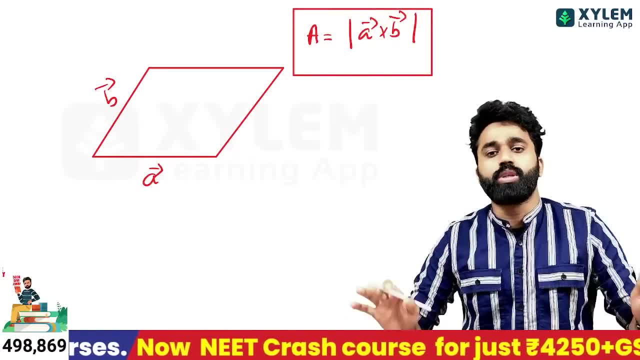 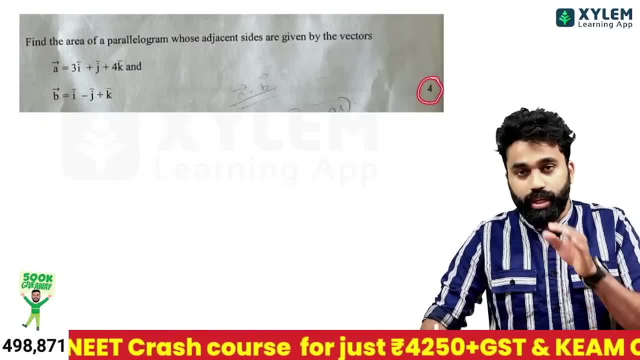 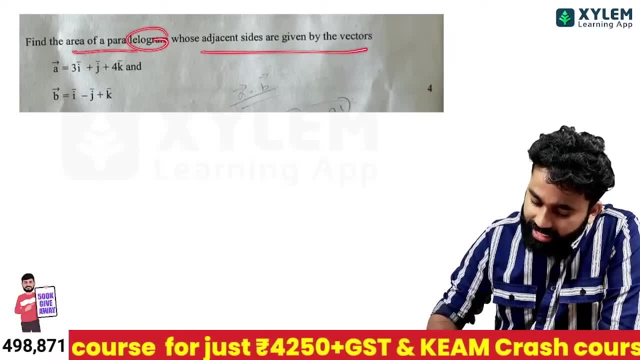 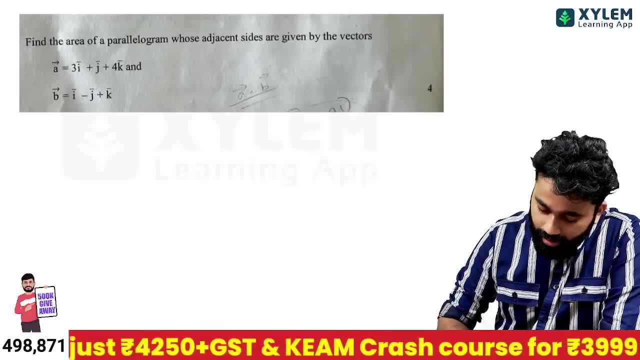 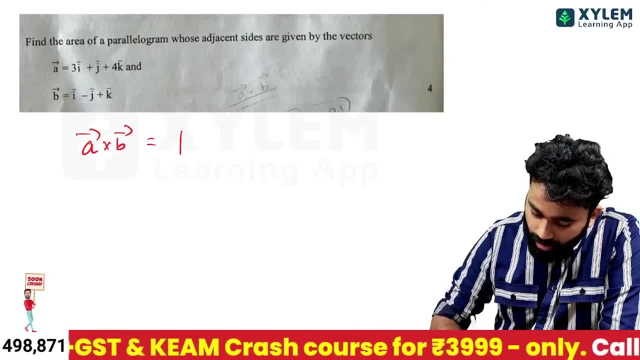 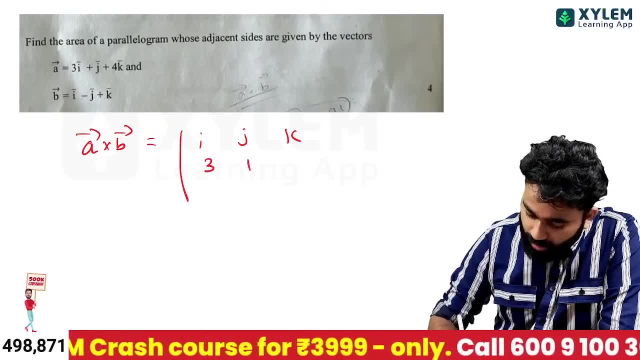 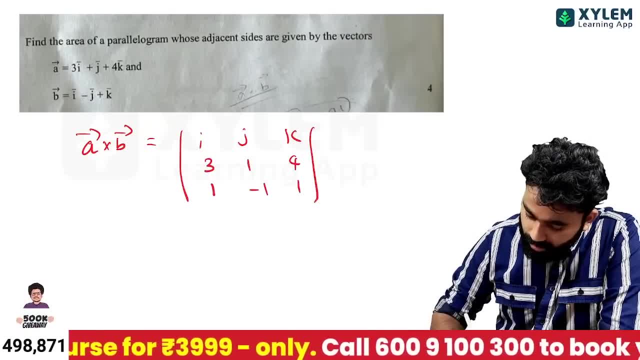 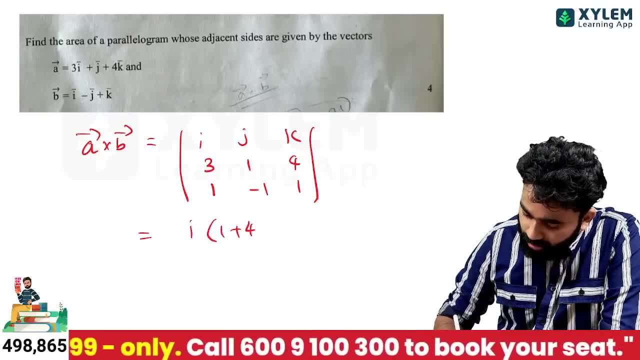 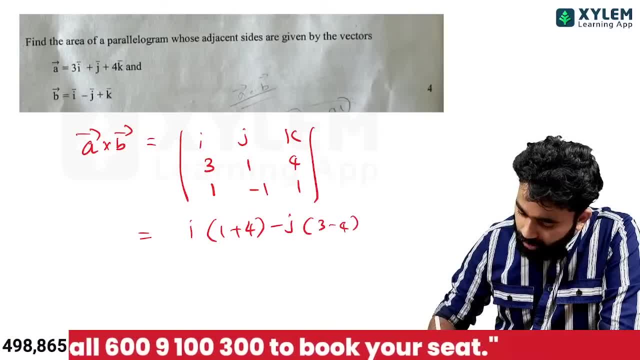 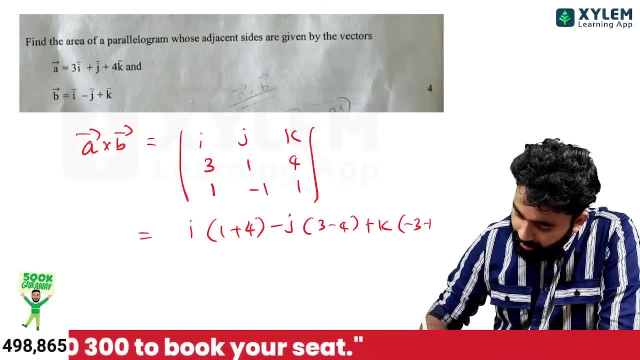 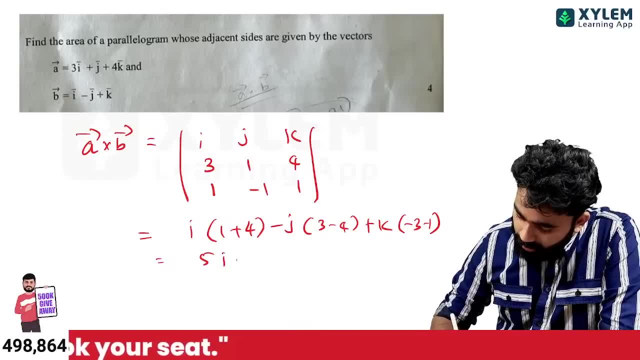 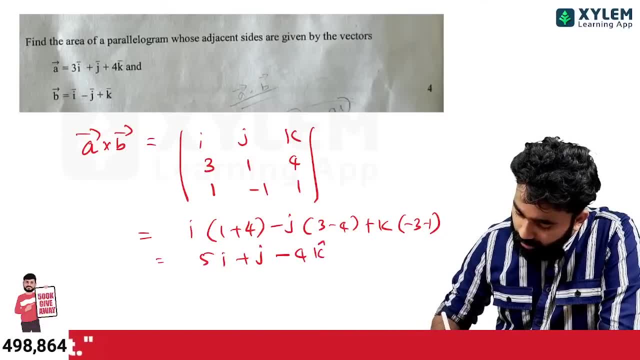 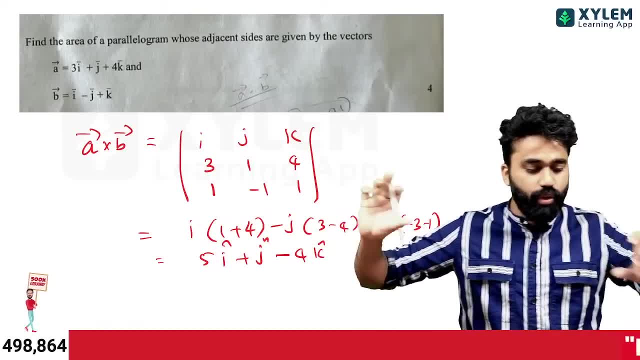 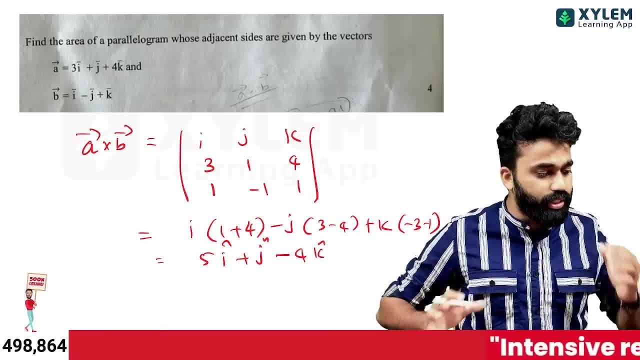 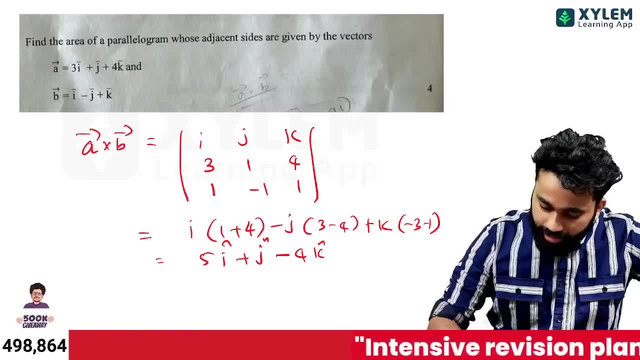 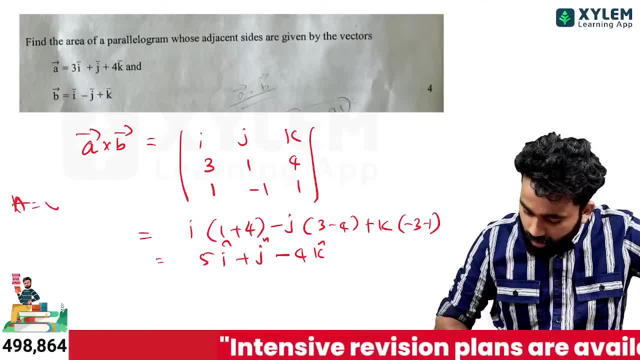 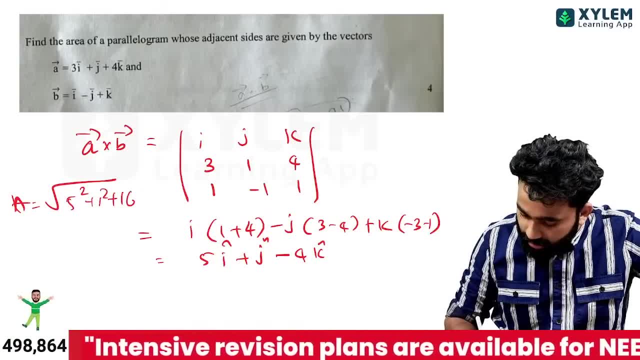 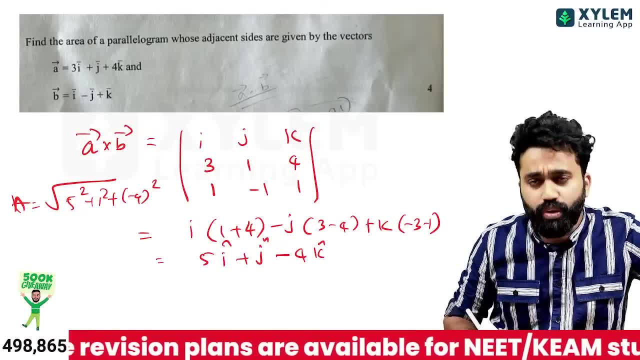 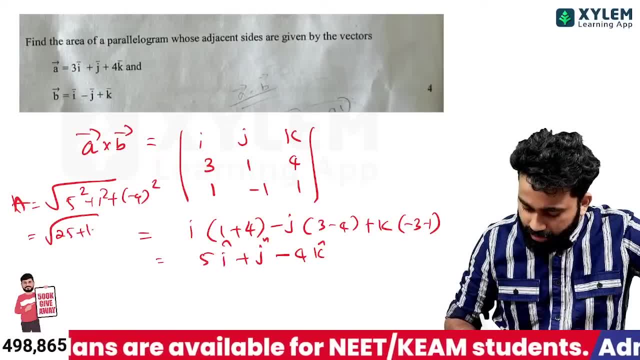 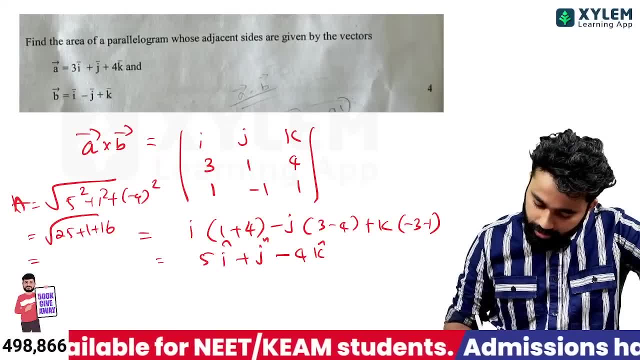 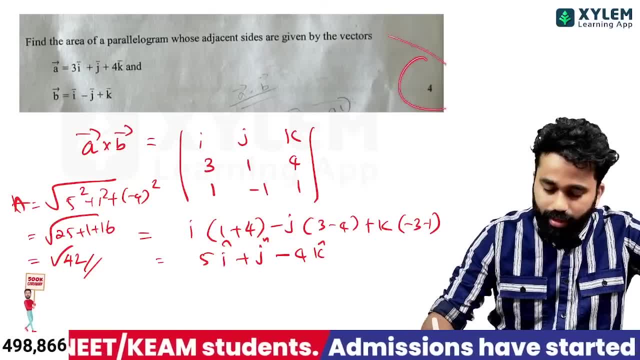 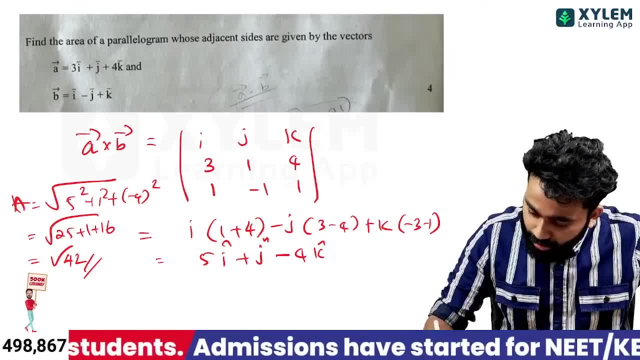 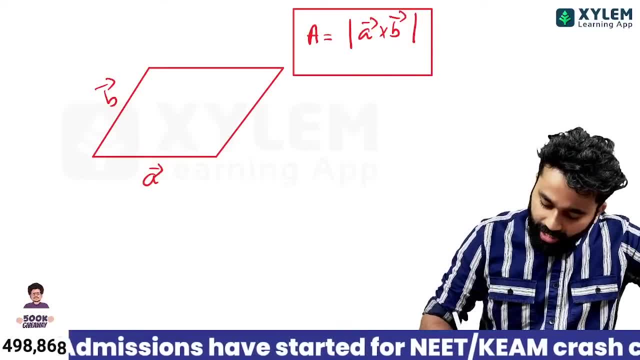 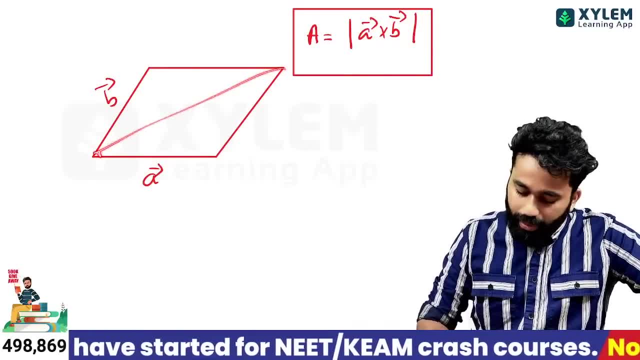 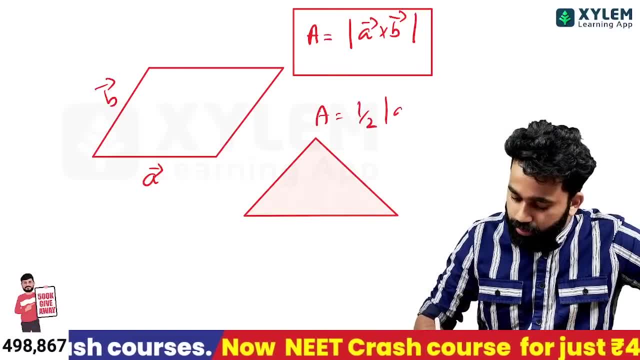 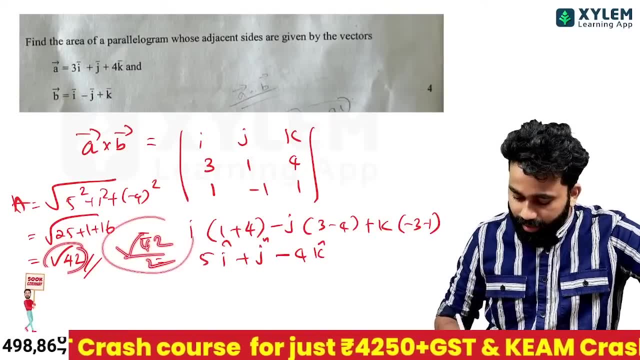 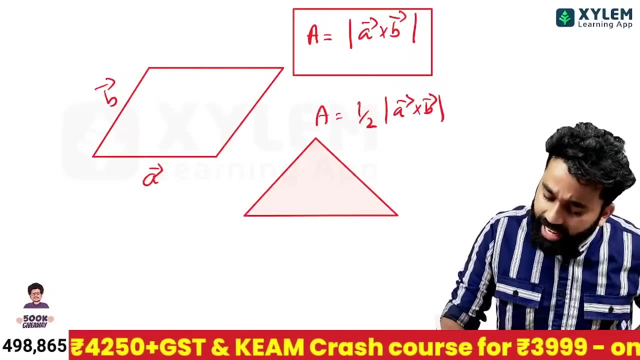 So the area of triangle is equal to half times A cross B. Now, if this is root 42,, then root 42 is equal to 2,, which is the triangle area. Is it true? Did you study both? Now I will tell you one more extra thing. 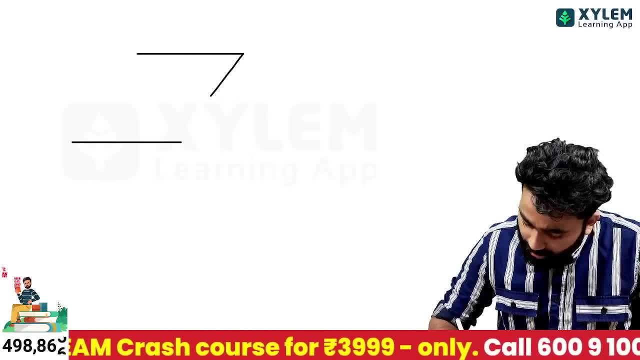 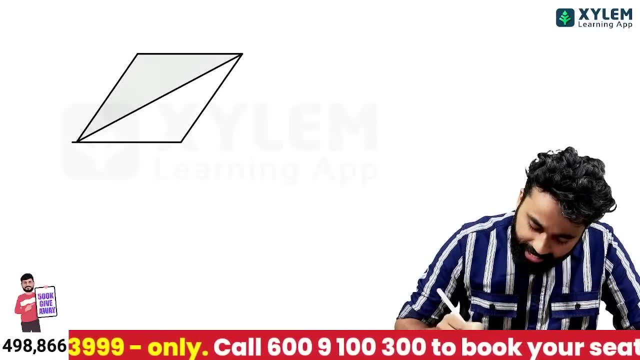 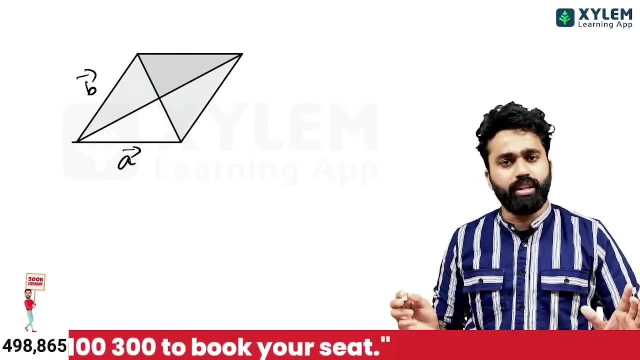 Those who get this A plus level if that question arises, those who don't want it, please study it. If you ask to find the area by using the diagonal vectors of a parallelogram, I have given two vectors. I am just telling you to study. 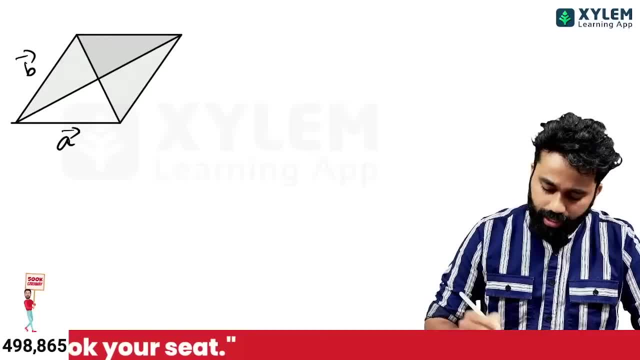 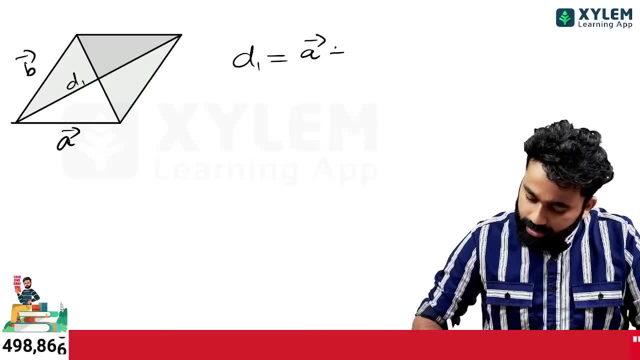 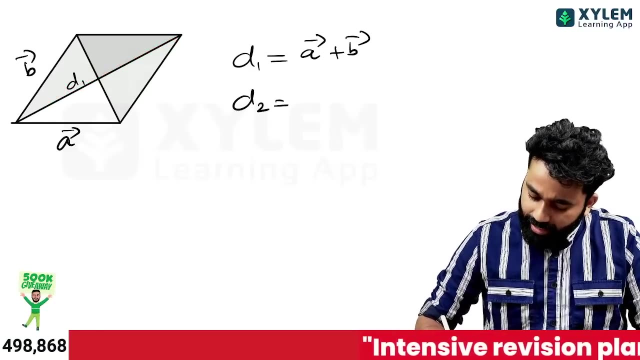 Not everyone has to study. Those who want to lose A plus in one way, please study it. A plus B is the diagonal of D1.. Add two vectors. What will you get? You will get the diagonal of 1.. D2 is B minus A. 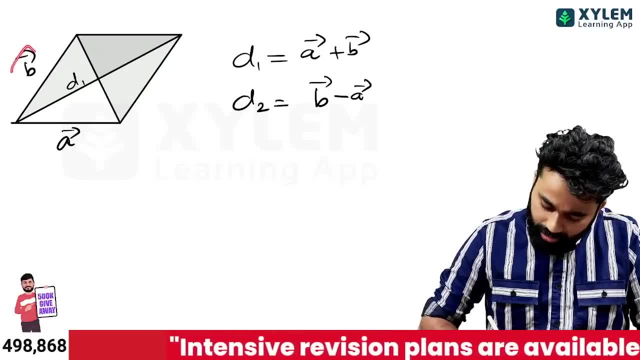 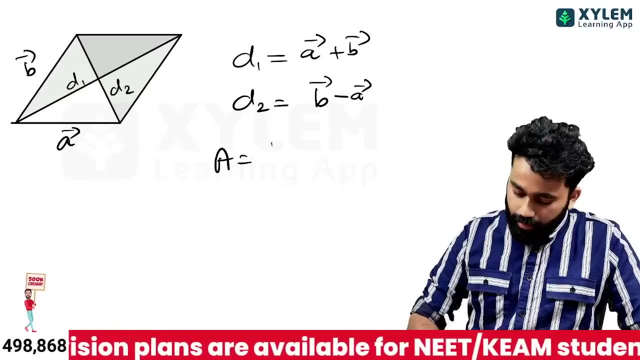 When the first vector is reduced from the second vector, D2 is obtained According to the parallelogram law. Add two diagonals. You can see its area Half times D1 cross D2.. This is the equation to see the area by adding diagonals. 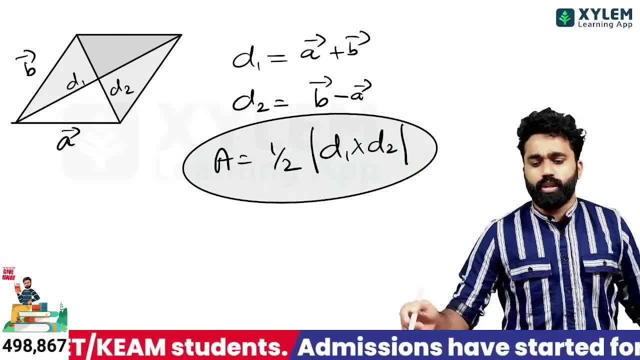 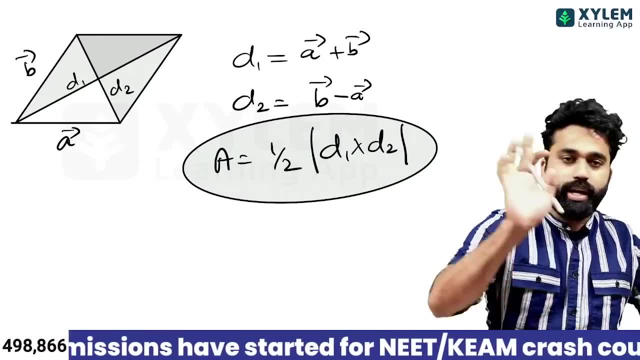 This is not that important. It is a question that is frequently asked in CBSE. It is not that important. So if you want this, please study it. If you want, please study it. Don't lose A plus 1 anywhere. 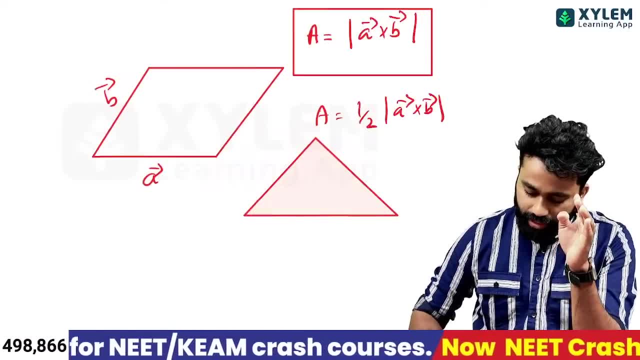 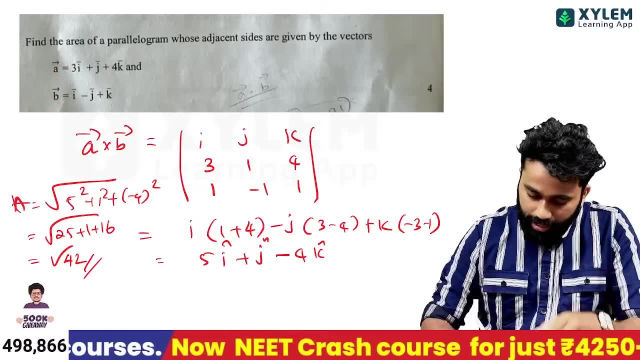 Is it correct? You can see it directly. D1 is two vectors. If you see A plus B, you will get D1.. If you see B minus A, you will get D2.. If you want, you can do it. 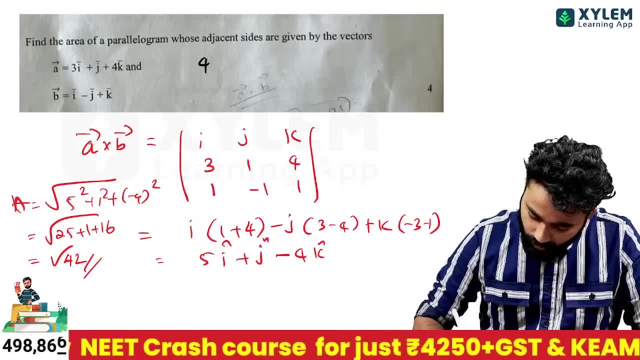 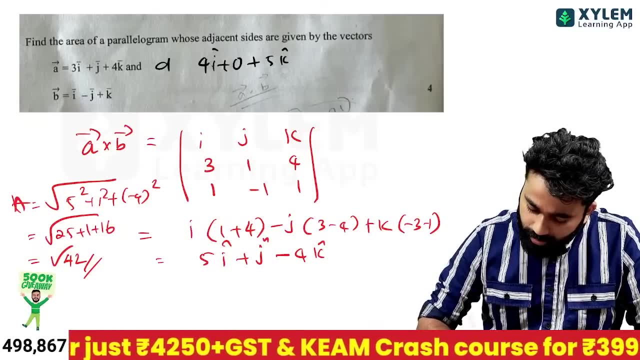 What is A plus B? 3 plus 1 is 4.. 1 minus 1 is 0.. 4 plus 1 is equal to 5k. This is A plus B. This is D1.. What is D2?? 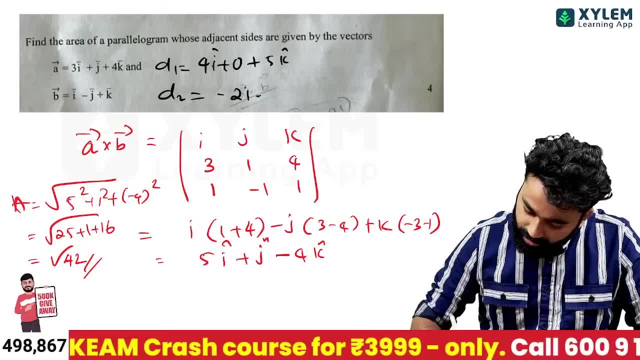 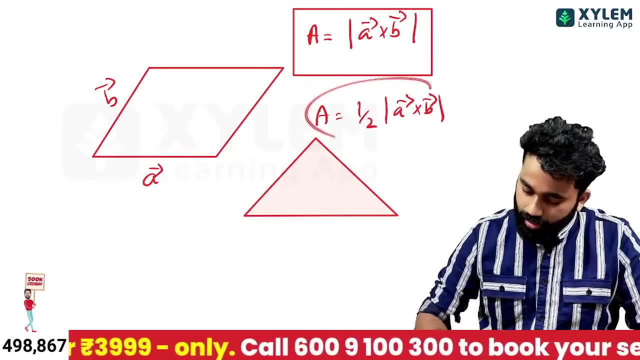 B minus A, 1 minus 3 is minus 2i. Minus 1 is minus 1.. Minus 2j, 1 minus 4 is minus 3k. This is D2.. Please try to answer this question. 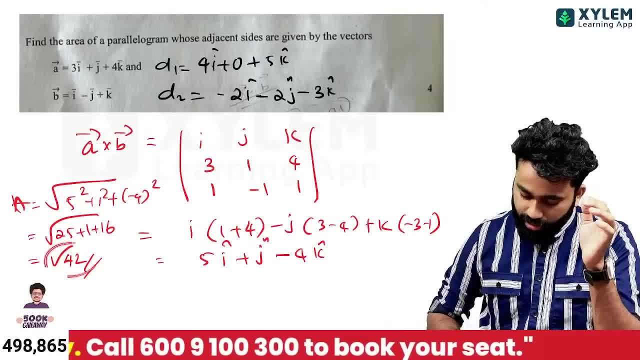 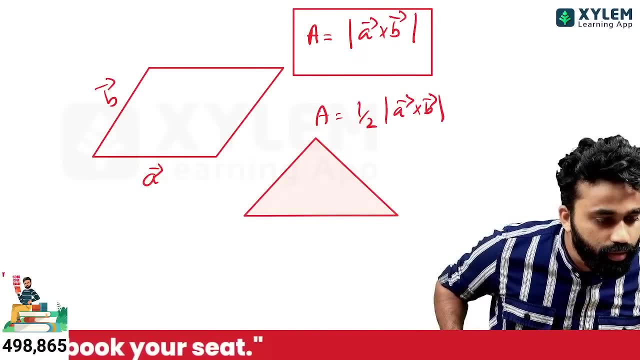 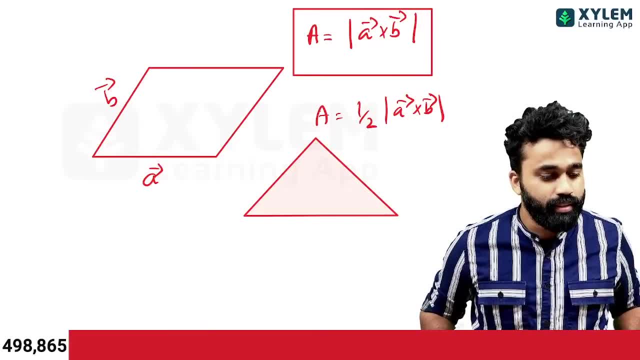 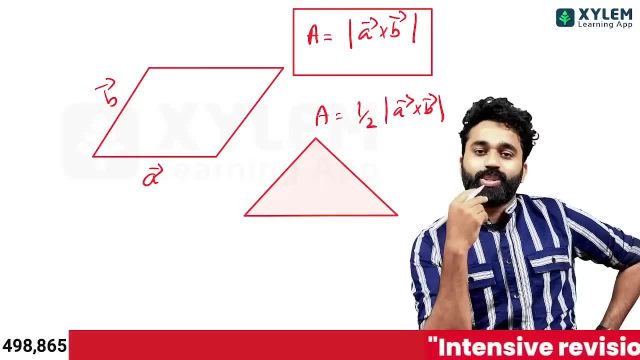 Does one character of Sir matter to us? Have you ever seen a big picture? Has this not the truth in my mind, Sir? please provide only the important questions. If you get an opportunity while taking one question, you have been told that important. 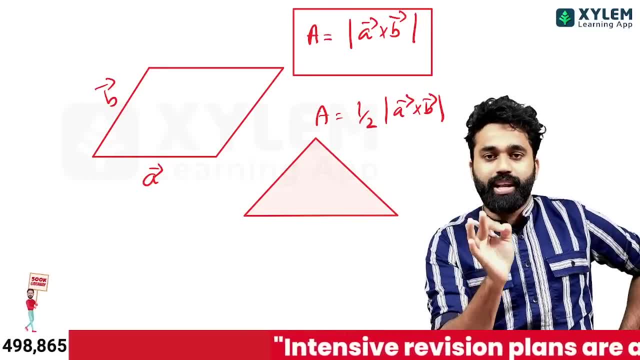 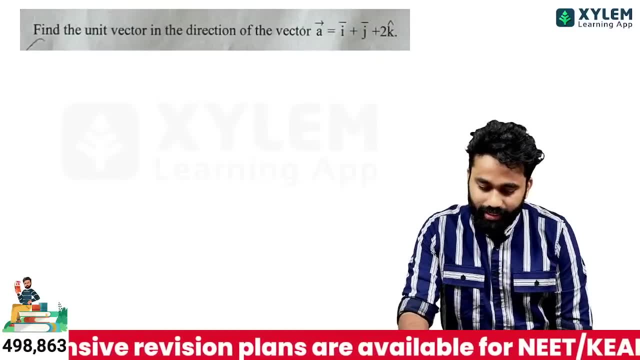 that infectious and other are all not important, Because in India They all have to study exactly as same. They all have to study exactly as the same. Please, don't be afraid. also, Please, If you giveА donc Time to thank you to you. 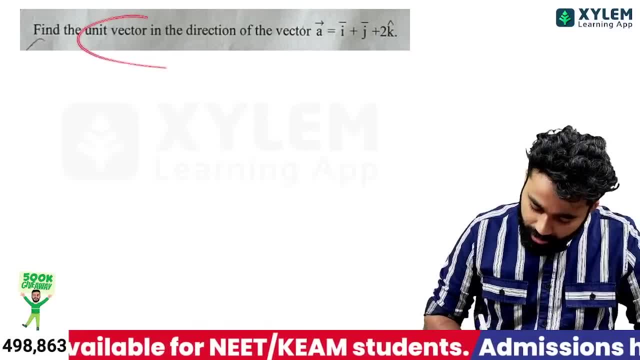 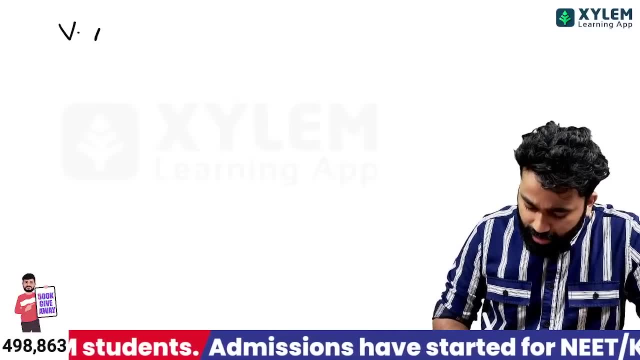 What is the answer, Sir? please confirm If it is correct. homework I decide on unit vector. gonna put up a channel. so McLean vector, algebra and the brain, that chapter in the name of the parish I could be involved in. the a to mark in the children are a little or a pitch or 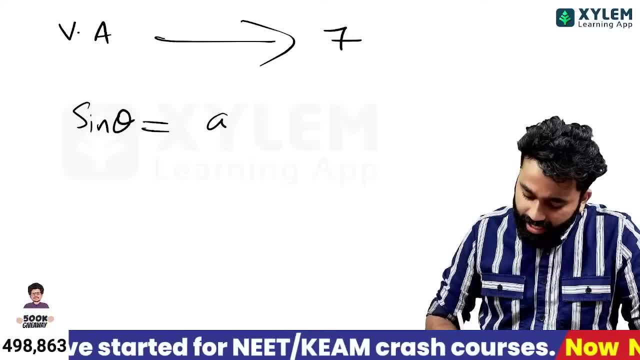 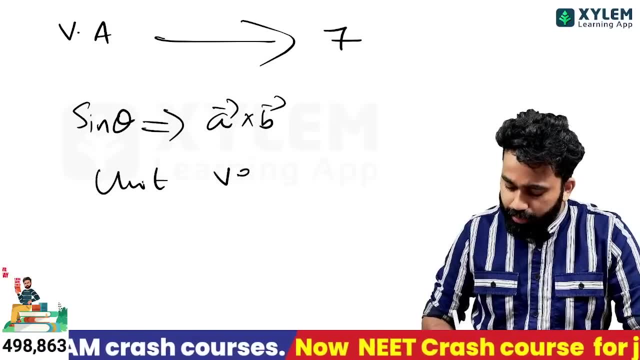 ningle color, or each other sign, theta which it ever a, cross B which it will, or each other, my region or each other other picture, and I'm at the unit vector which it will go, seen, I give them to mark in other, or pitch, or moon, I'm at. 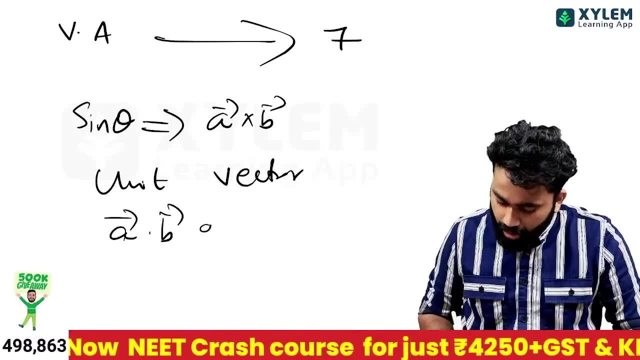 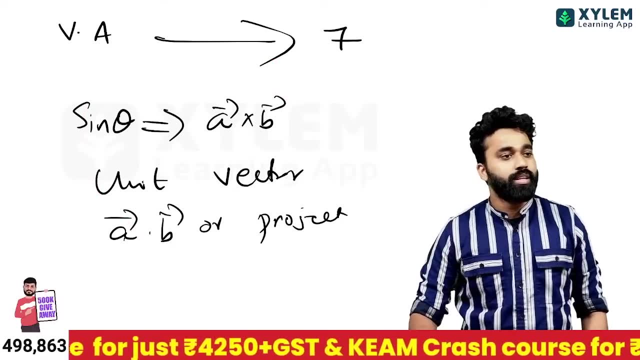 the a dot B which it will. a little projection a dot B or projection which it will. a or a question, I think you a moon ill or a more the children are a too important in the very little. a more the children are a too important in the. 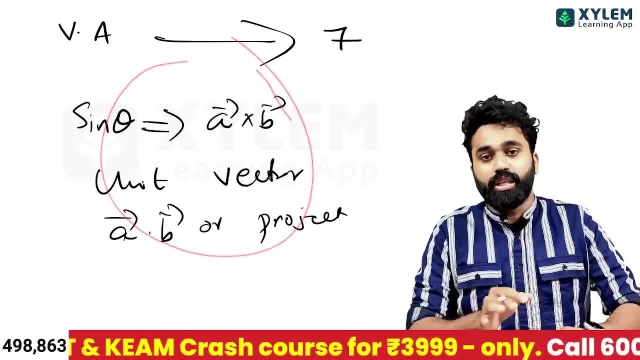 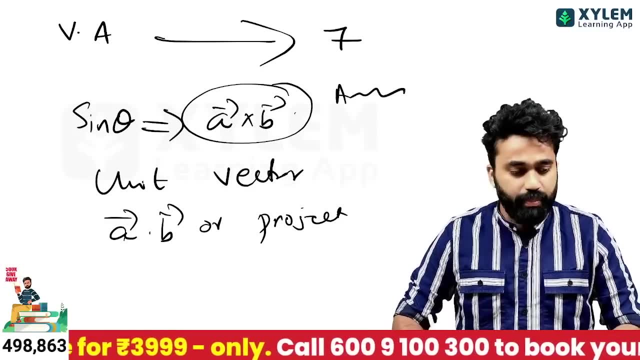 very little, a bogatyr in a lot of the children in the upper position and I engage our Brianna in the nana la bago closer to the tundra. a delay, a sign, theta across. we have to do that and silence. delay. area of parallelogram area. 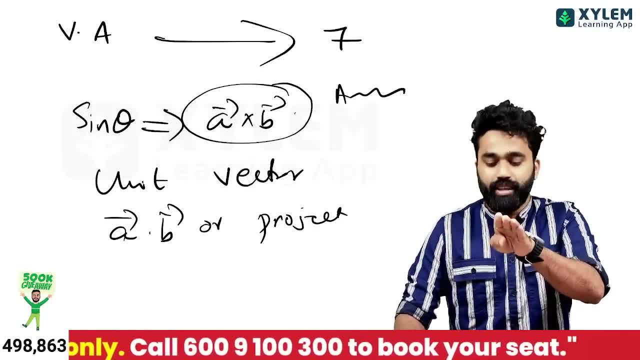 of triangle. we're upon your local, a triangle in the varanjala and Donna parallelogram in the area can do, but today method or a macho la in the tent that the Madi. I did a. how do you do that? I did a. how do you do that? 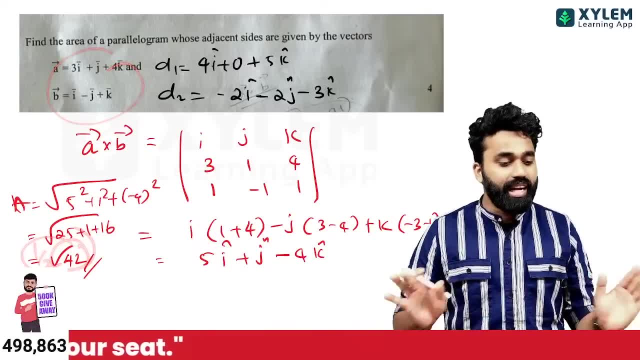 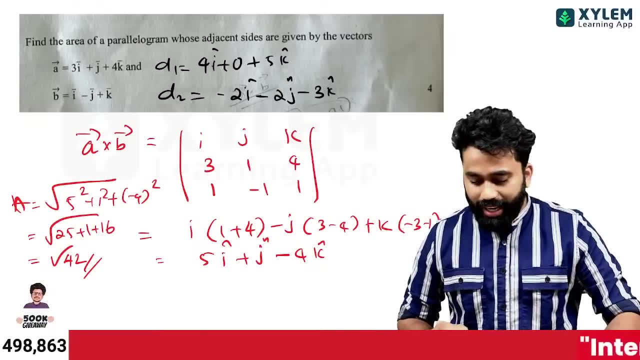 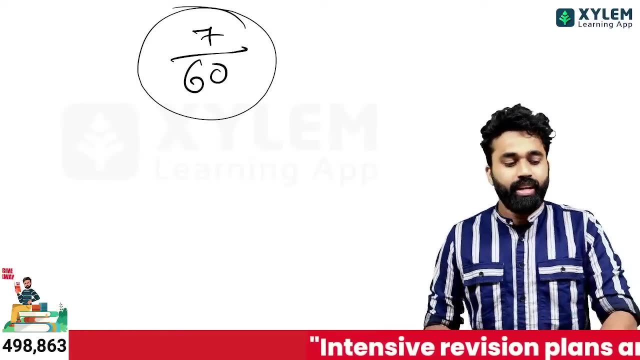 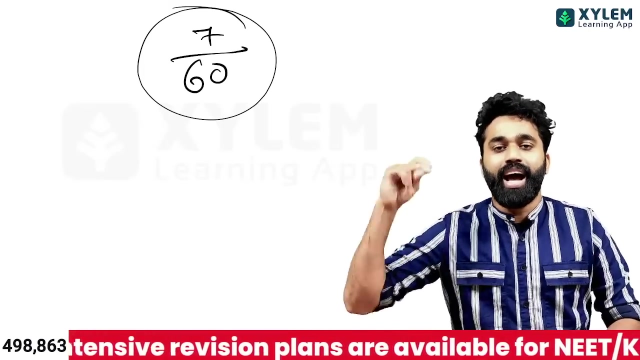 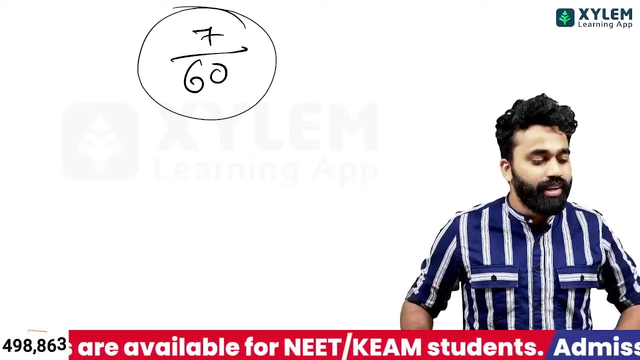 have to see throughout Omani raped damn round from the K tropic. have to see throughout Omani raped damn round from the K triumph eternity. I'm a amusing doing new using old political 對. don't extremely using old using old NA. wish you all the best and I am ending this class here. 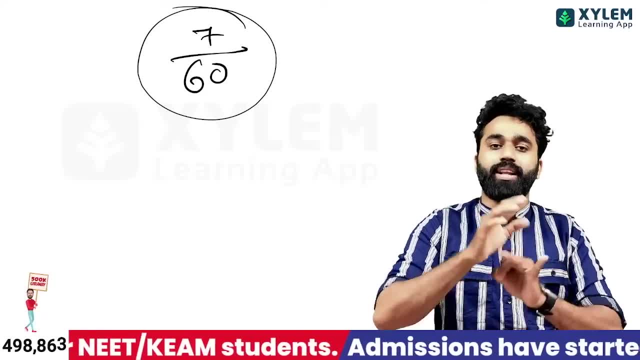 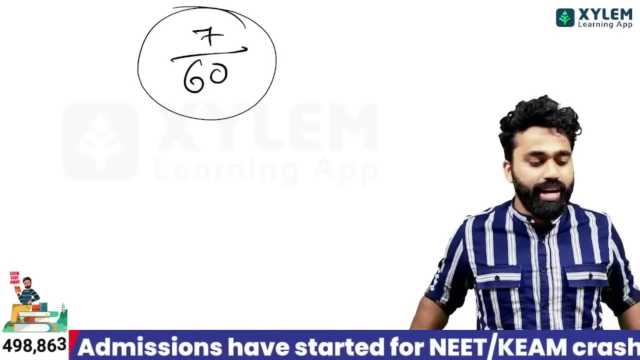 Shortest Distance Angle Between Two Lines, is another chapter called 3 dimensional geometry. you will get 7 marks out of it, so I am assuring that everyone will be able to study well, and I am telling you not to miss any class on any of the days. 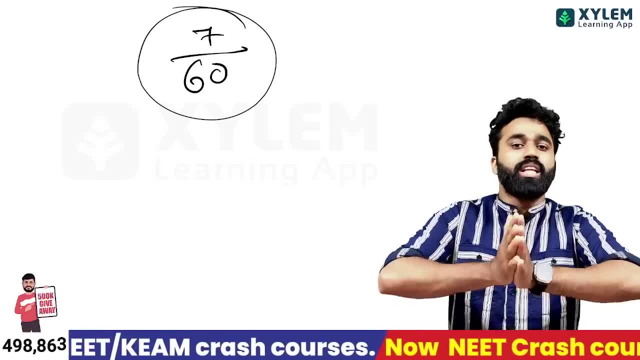 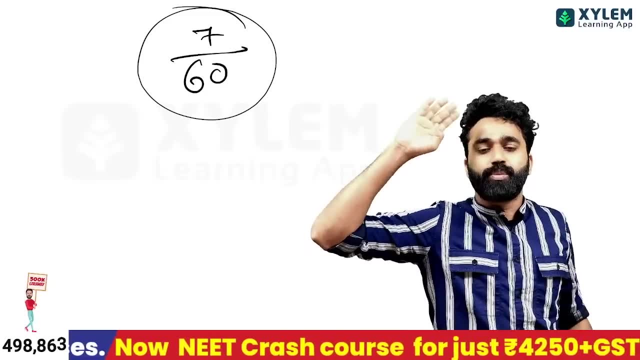 specially. I am ending it here, so today is Friday and many of you will have to go to school. I hope you all will go to school and come back to our next section. It's me Shahid from Sam From Silent Learning. Bye, Bye.